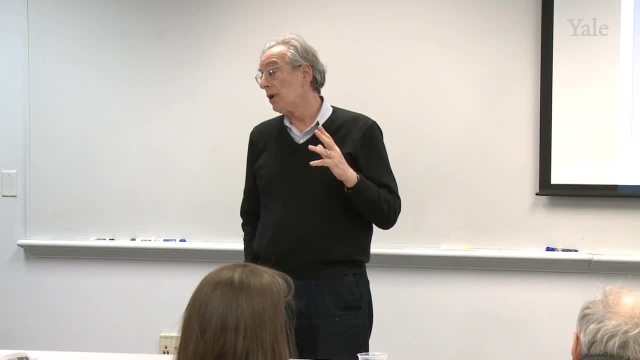 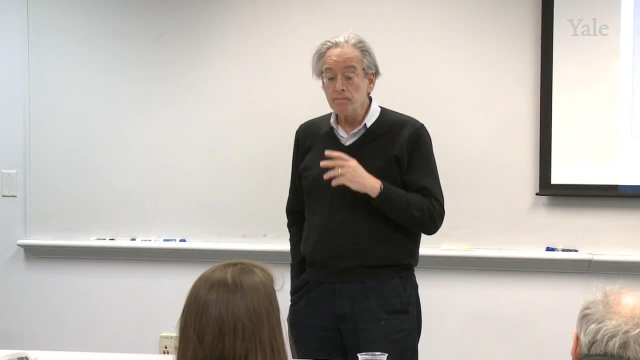 are extremely significant, particularly his work on tectonic uplift in Tibet with Kutzbach and his former student, Maureen Ramo, And the origins of the East Asian monsoon, And then, beginning in 2003,, his publications concerning his discovery, his realization, his early anthropogenic hypothesis, which 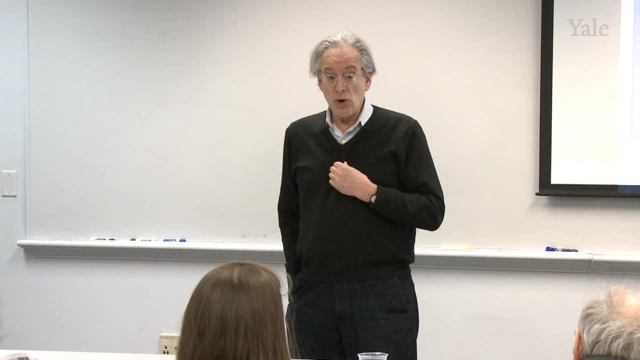 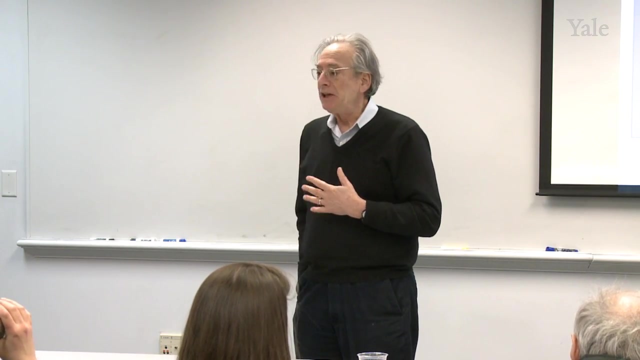 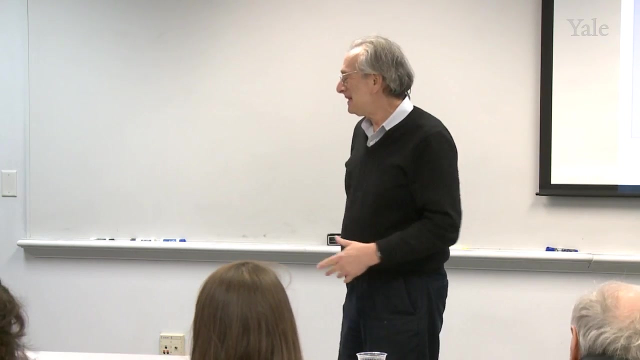 has received a great deal of attention over the past more than one decade. More recently, he's been the recipient of the Lyle Award of the Royal Geological Society and the Nobel Prize in Engineering. The invited guest at the Power of Yale University Lecturer-Service. we're very much pleased to 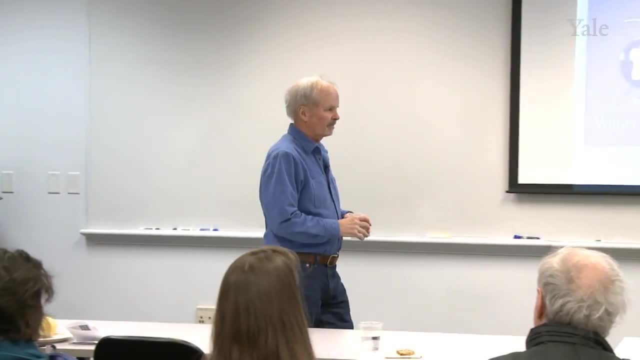 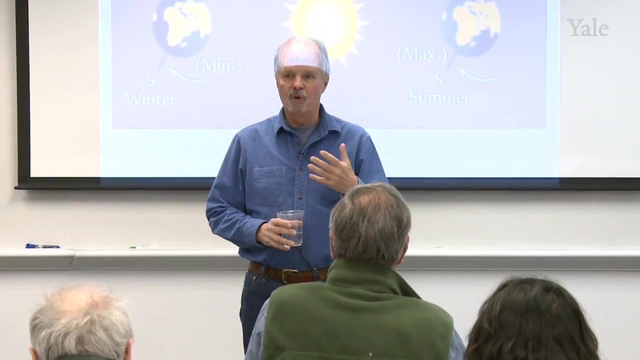 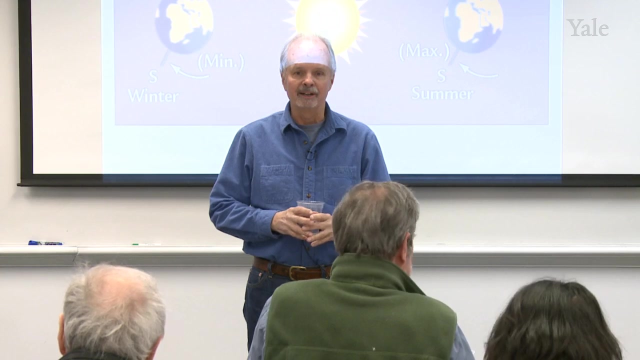 have him here with us, Professor Rudiman. Professor Rudiman, Thank you, Harvey. I had a very full day and one of these people has kind of a mushy voice And if I'm in a crowded room I'm up at the top of my range trying to be heard, And I have woken up the 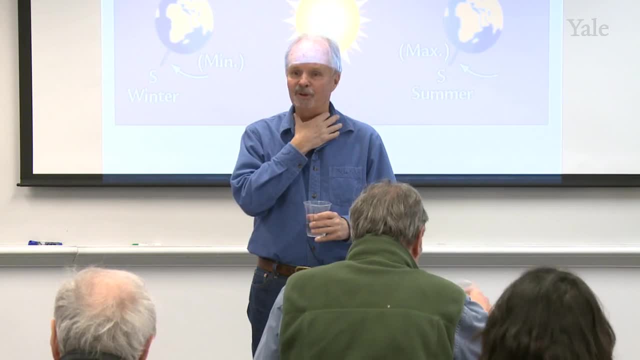 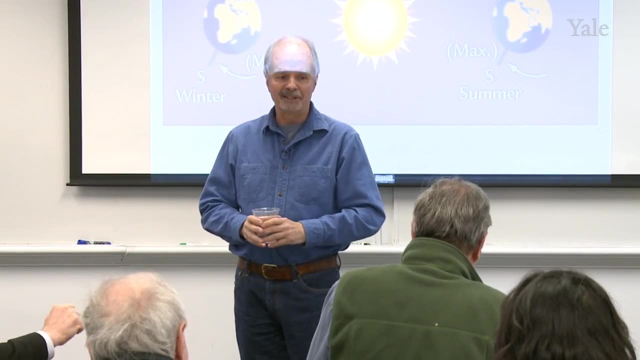 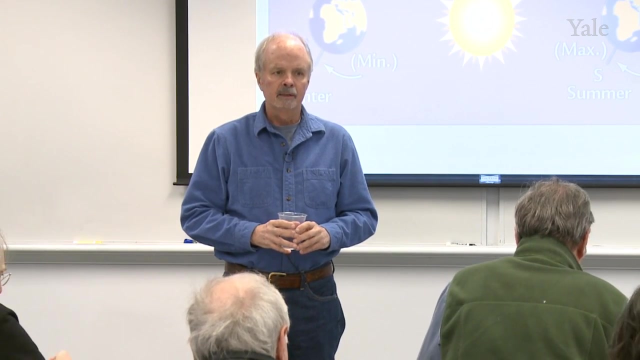 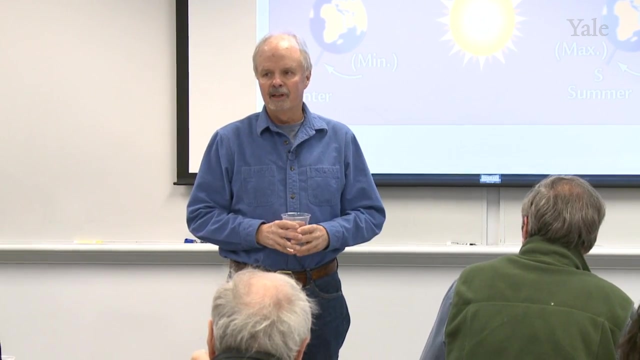 second day with virtually no voice before. so you're lucky, I'm still still got a voice. in fact, it's down in a far more impressive register that I usually speak- speak from. can you hear me back there? I assume you can. I once flew out to Illinois to give a talk to the atmospheric sciences department and on 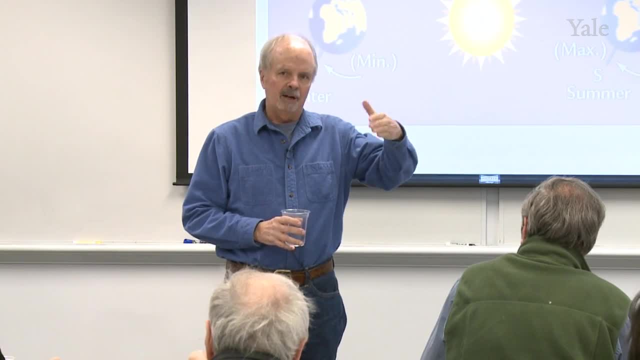 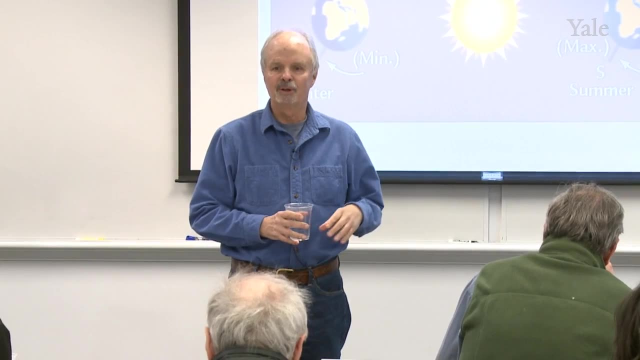 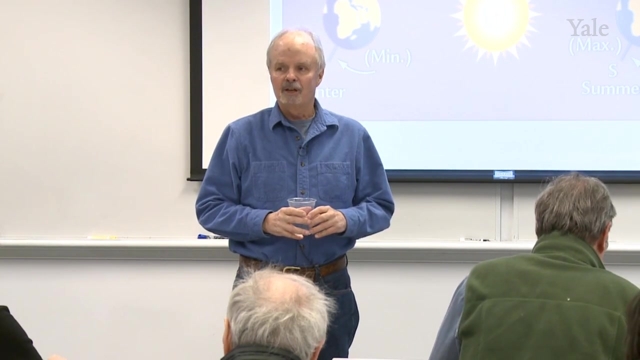 the way out I caught a cold. I had a couple layovers and long stops and I visited faculty the next morning and I was losing my voice and losing my voice and four o'clock came to give the lecture. I didn't have any voice left at all and I said: could you crank up the the amplitude on this microphone? I said: 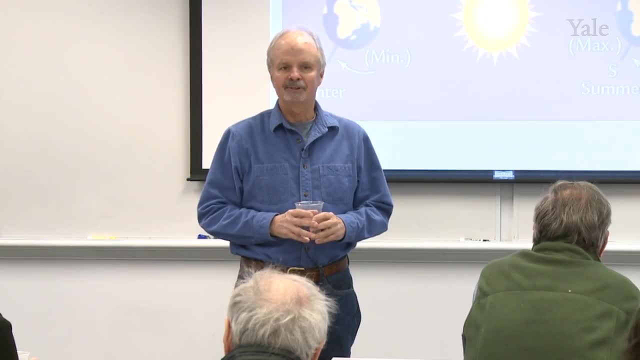 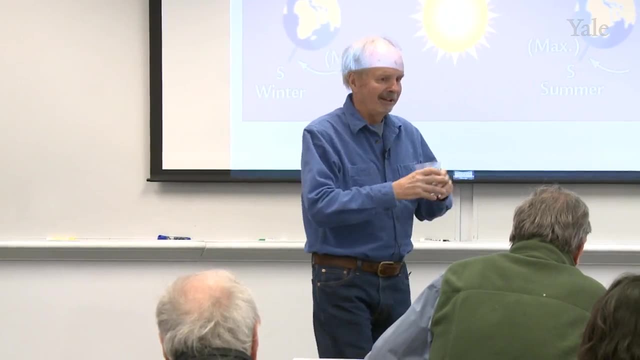 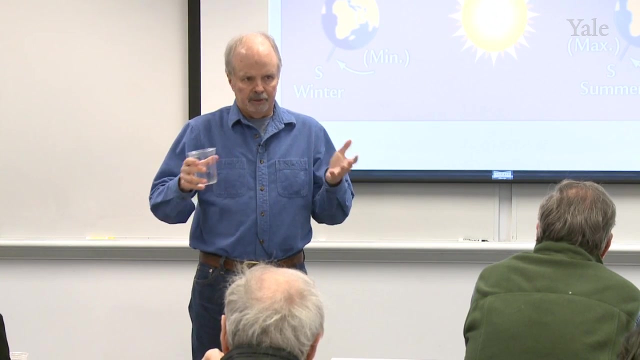 I'm giving this lecture and I whispered a 50-minute lecture. I said I swear I didn't say one word. that was whispering, so you're lucky today. this hypothesis that Harvey mentioned, it's kind of a interesting situation. most of you, I gather, would be scientists and you. 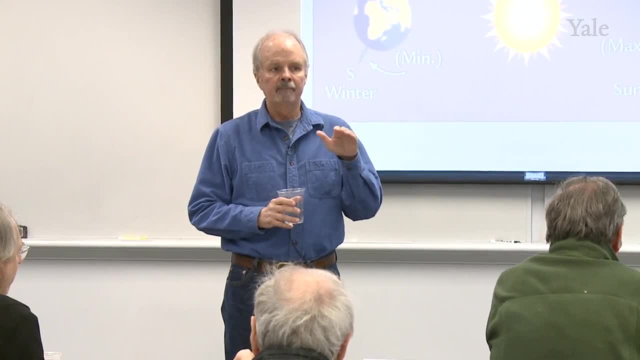 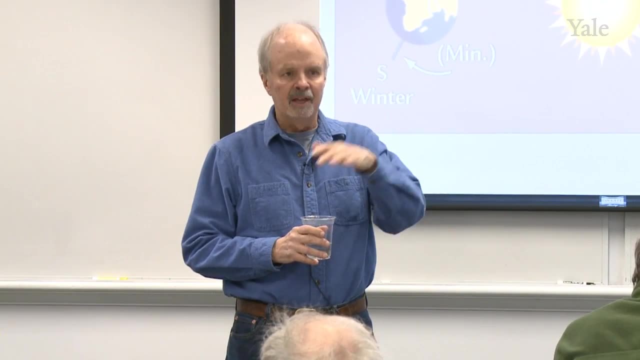 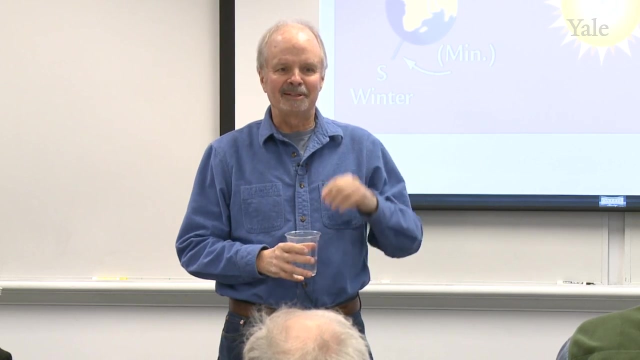 you know that hypotheses come and go. some of them are just ignored from the beginning. some of them get a little attention, are shot down completely and then they're ignored. some of them succeed and become theories. I see some smiles out there- personal experiences, I guess- and but this one is in a middle category, which is 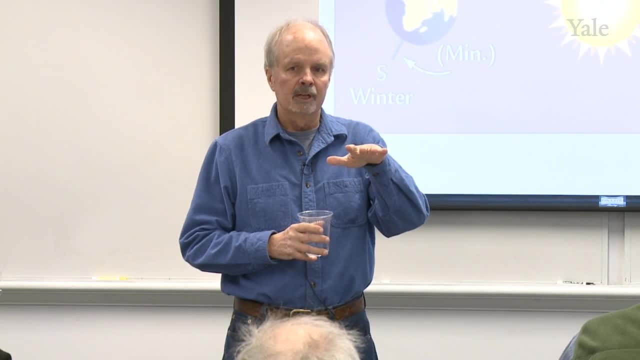 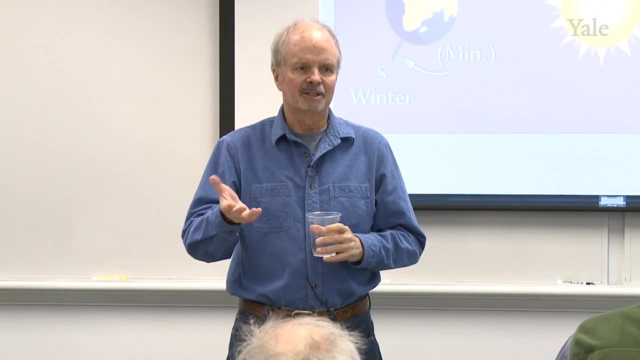 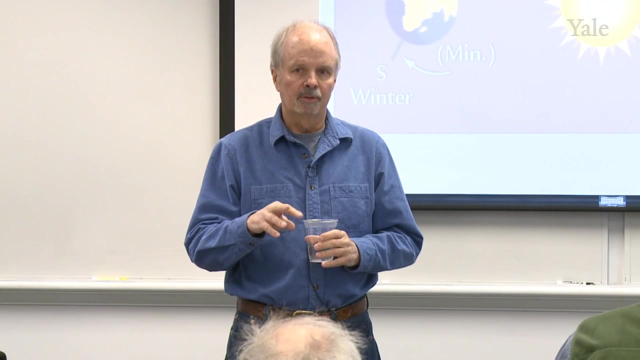 the hypothesis from the beginning had enough evidence that you just couldn't say it was impossible and it's. it made. it made pretty good sense, but there were. there was other evidence that argued against it and I'm going to try and touch on both of those and, if I skim over the criticisms of the hypothesis. 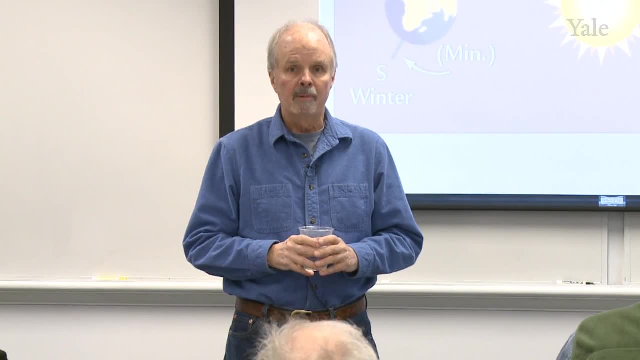 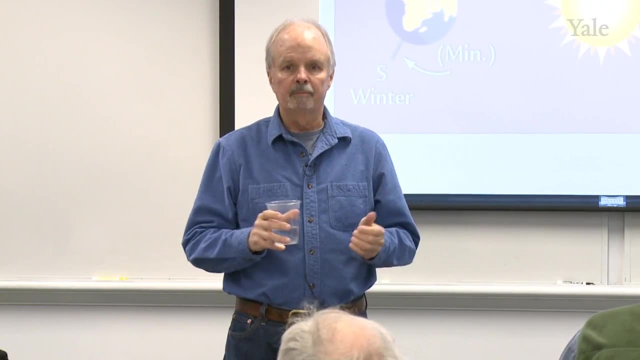 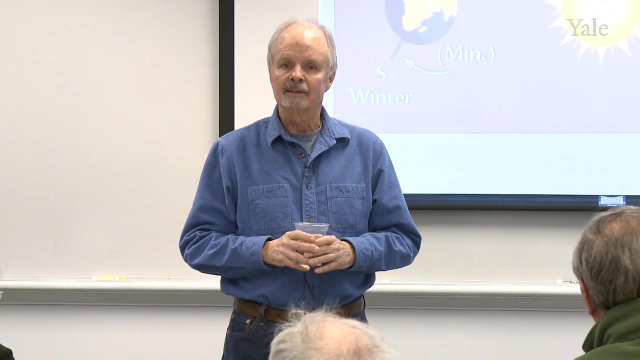 forget to get into that. you can bring me back, so, but I would describe. the situation is that communities like this: you talk to different people, you talk to different disciplines, you talk to different universities and you meet people that don't like the idea and you didn't meet people that think it's obviously correct. 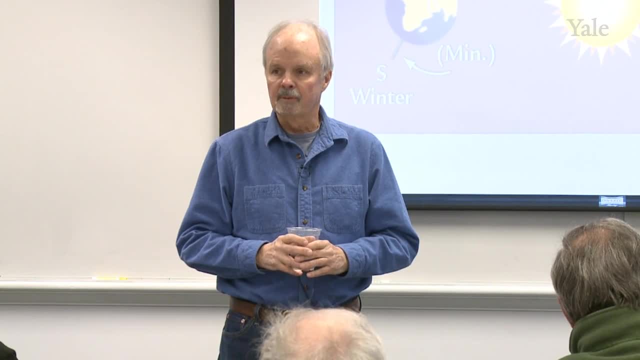 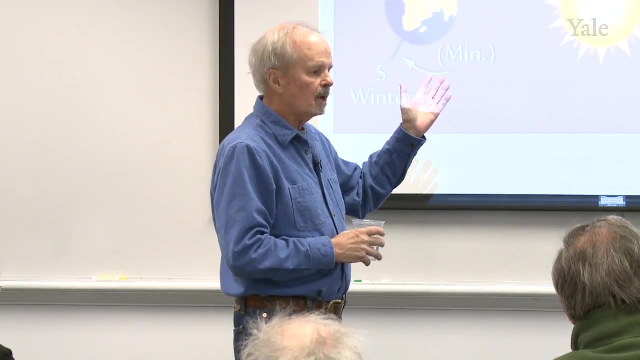 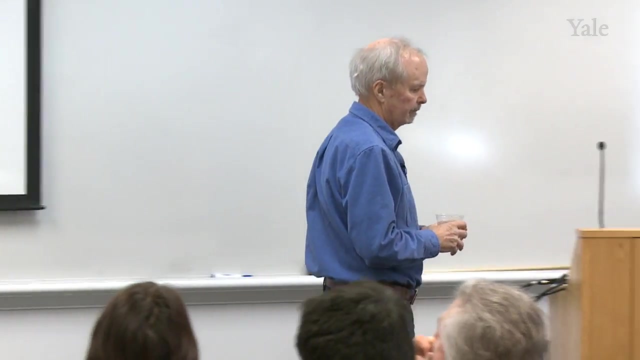 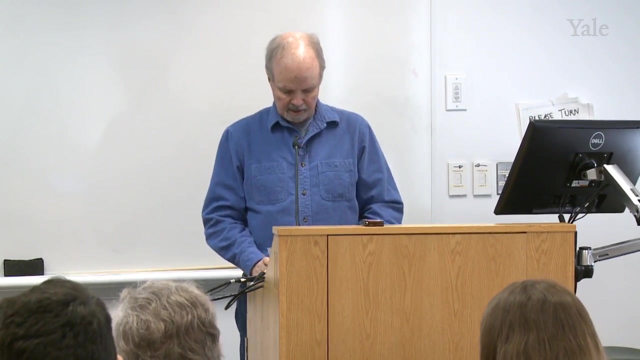 and so it's hanging out there. I'm very optimistic that I'll live to see it become a new paradigm, but it's not there yet. so I have two kinds of evidence the way the talk is structured, two kinds of evidence that bear on the hypothesis. how's this? maybe I'll save my voice a little more. so one line of evidence for. 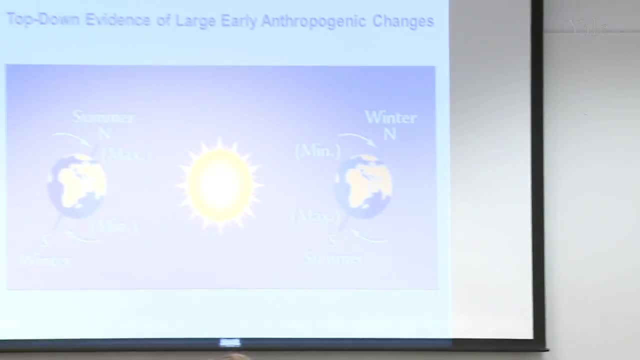 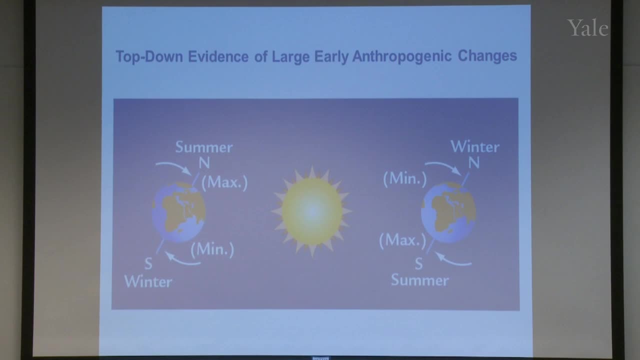 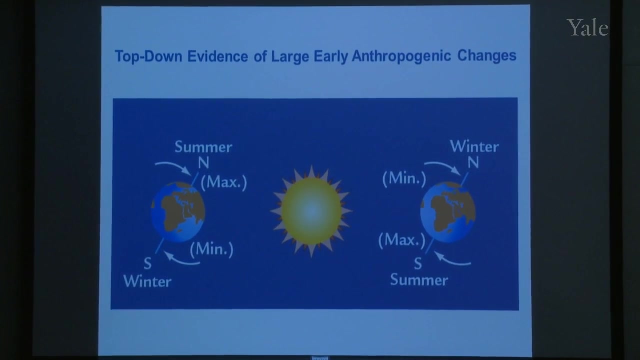 those of you you heard me yesterday. there'll be some repetition from yesterday's talk, but much more depth here. one is top-down evidence of these early anthropogenic changes, that is to say that farmers and agriculture were all altering climate thousands of years ago. it didn't all start with the industrial era. greenhouse gas increases that began. 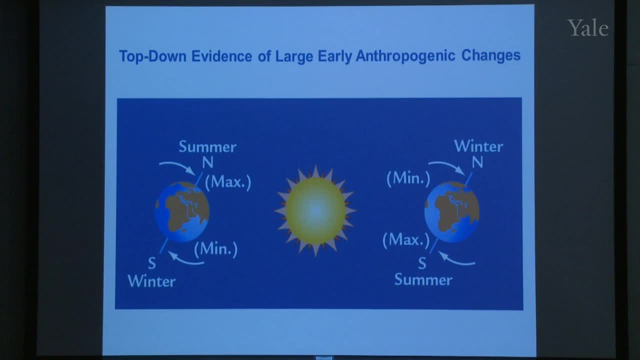 really noticeably around 1850, and this, this top-down evidence, has to do with the composition of the of the atmosphere, particularly carbon dioxide and methane, and the. the way that this evidence comes into play is that people that have drilled down through ice cores and retrieved dome sea Antarctica retrieved 800,000 year record. 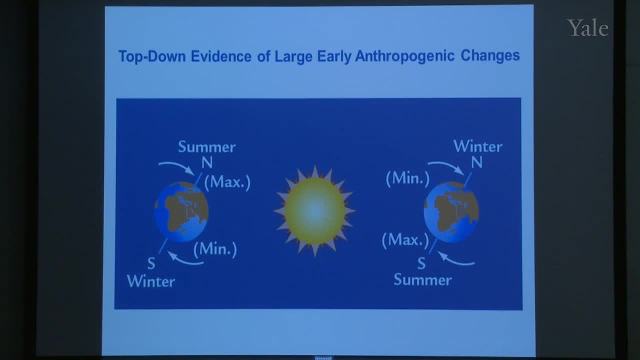 of past greenhouse gas compositions. that record goes through several more than a half dozen previous interglacials, and those are times when nobody's claiming that humans were massively affecting greenhouse gases. so there that's a time when greenhouse gas changes were natural, and there I'm going to show you results. seven of them. so we 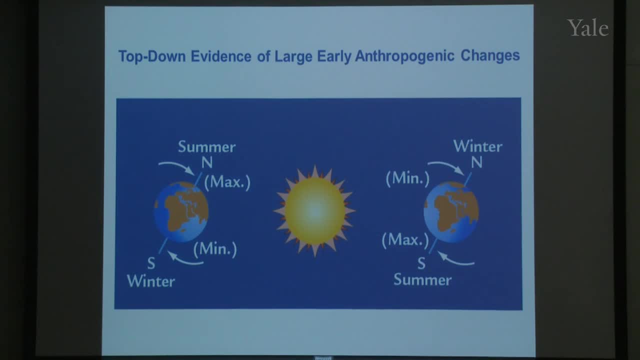 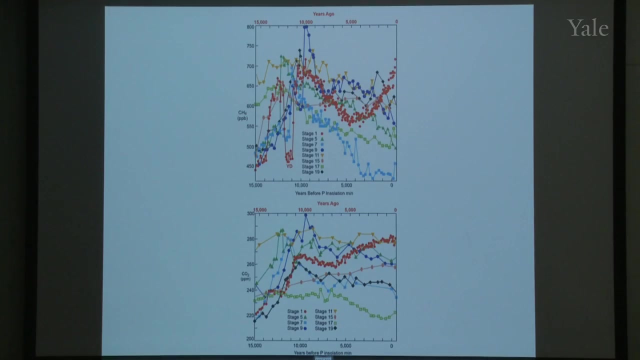 can take the Holocene, which has its own carbon dioxide and methane trends and which I say is over printed by humans, and compare them against these experiments that nature has run in the previous interglacials programs. have a lot of time to find out what thiskus graph actually did for the 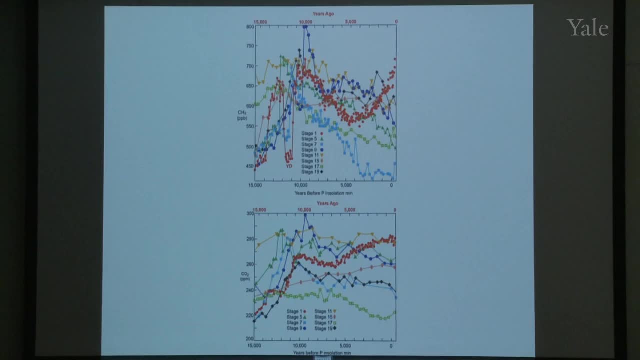 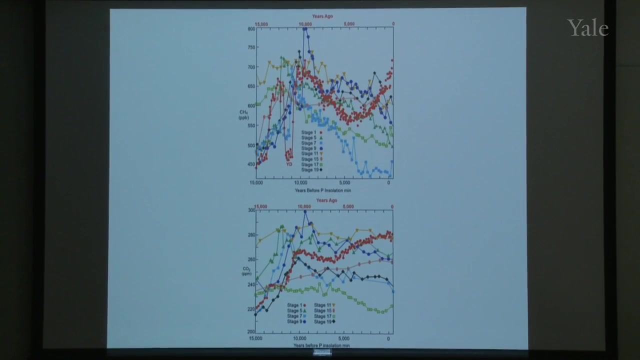 earth is a really good researchers and celebrates of what. Here are records from previous interglaciations of methane at the top, carbon dioxide at the bottom. and there they're all. they're all aligned on a common reference point in the ice core Tom time scale, which is set to the present day, which happens to be a. 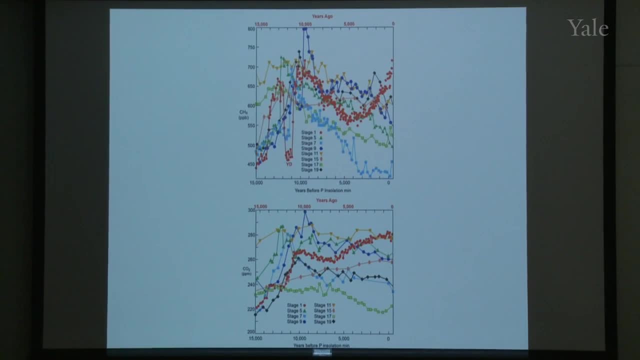 time when one of the orbital elements of procession is that the e sine omega, is that a maximum version of the uh, then there, then thisacto element, information did be victory over it in the early years, remove actually, and the évidemment in the early years of working. the unit collected addresses subso we pretty much had to end inерм 很nd. 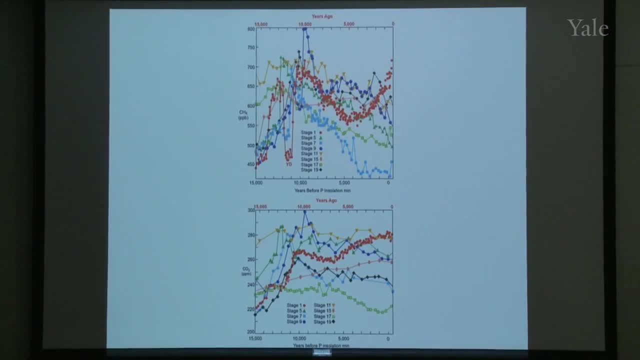 value. but you could think of it. northern hemisphere summer insulation is at a minimum. So these all have a common alignment within the errors of the time scale. so it's not perfect. Astronomically, from the orbital elements it's perfect, but when you try to. 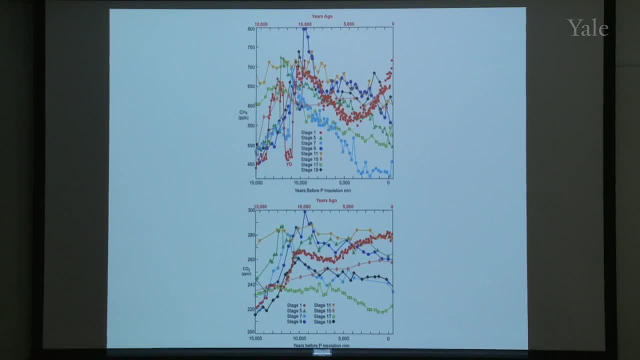 apply that the astronomical changes to the dating of the ice core. it's not perfect. Now you should be able to see here that I've left my pointer. I'll just walk over that. Oh, okay, that's better. There is something of a common pattern. you may be able to proceed. 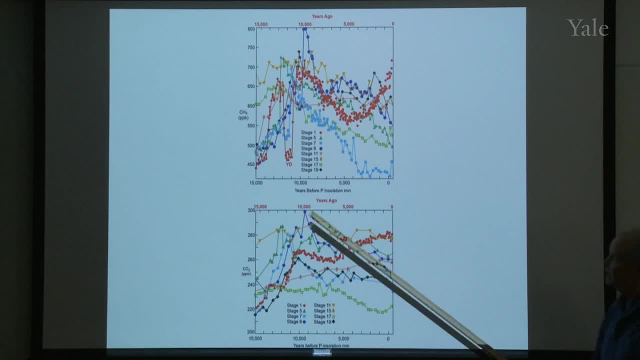 in both these trends and it's similar. it's more dramatic in the methane. There are low values, at times comparable to 15,000 years- Okay, Years ago, that's late. in the deglaciations that precede these interglaciations, There's 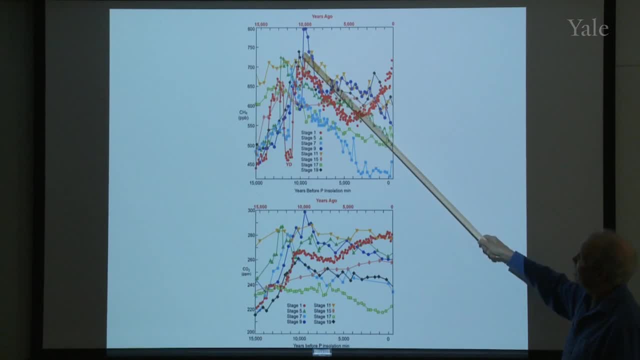 a rise to peaks somewhere in this interval and in most cases there are decreases- this is methane- to lower values, and those decreases go on straight through the time of the present. But plotted in red is the Holocene, which has a similar peak. I'm not going to talk. 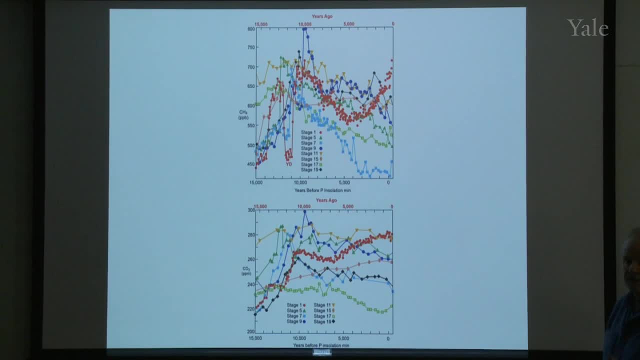 about this feature. This is the Younger Dryas, which is a different climatic beast altogether. But the methane trend also reaches a peak in the same general area, comes down and then it goes back up. I might catch these two high points. That's interglacial stage 19,, which is almost 800,000. 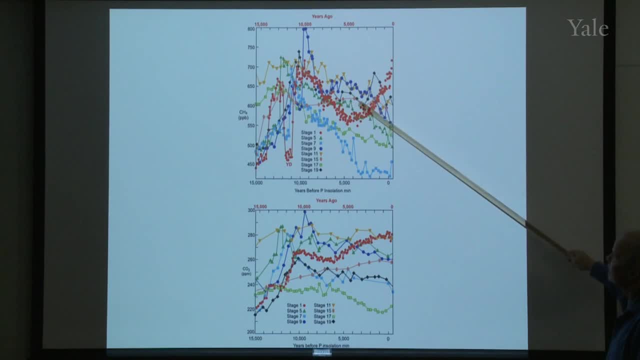 years ago and it looks like it's following the methane. But that's a brink of a peak. It's a brief peak, recognized from the beginning as being again one of these brief changes, If I extend this time scale for stage 19,. the methane trend went down, So they all go. 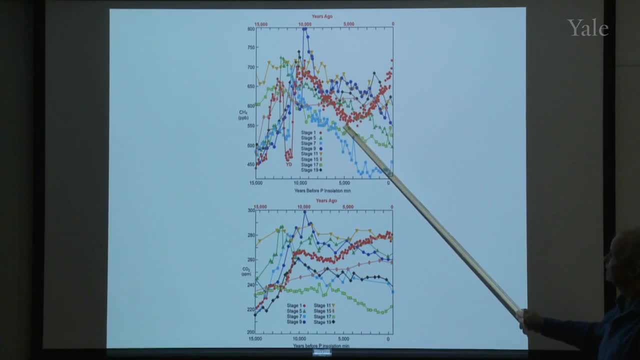 down, except for the Holocene, as far as methane is concerned, And methane goes way up instead of down, And so that was a first indication. I didn't have all this data 10 years ago, but that was an indication Something's different. 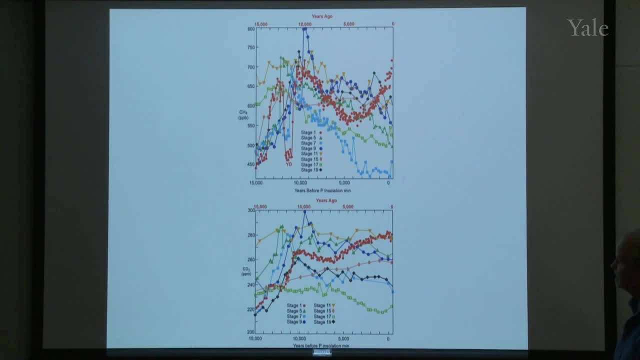 And for methane it starts at 5,000 years ago. CO2, at least plotted at this scale, is much more muted. Basically the same pattern: Lower values- in here- In this case the lower values are a little bit off to this direction- Peaks usually, I think always in the same. 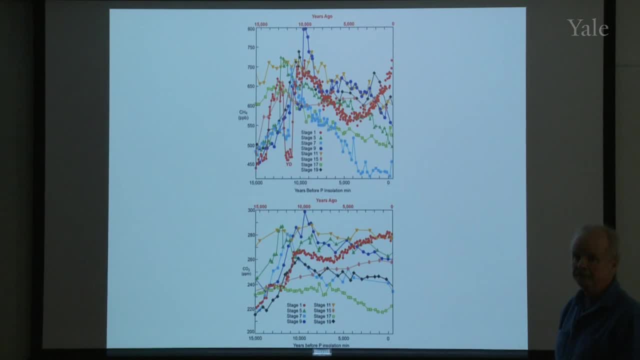 exact sample. as the methane peaks, So methane and CO2 reach a peak And then most of these trends go downward. Some don't go down very much, But carbon dioxide in the Holocene goes up, starts down and then goes up, So it's anomalous. There is one interglacial, I'll point out. 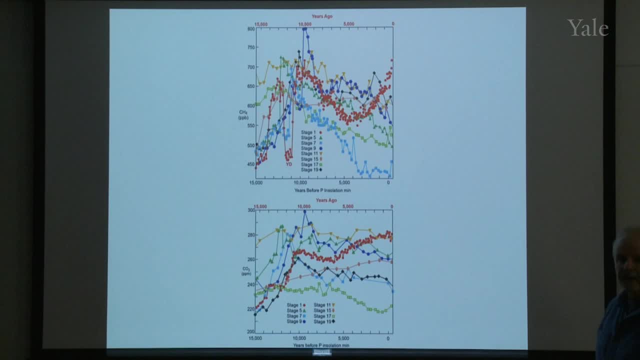 stage 15, which doesn't have this rapid rise. It doesn't have the look of a deglaciation And instead other indicators indicate that the deglaciation is somehow going on through the interglaciation. So whether you would even call it an interglaciation, 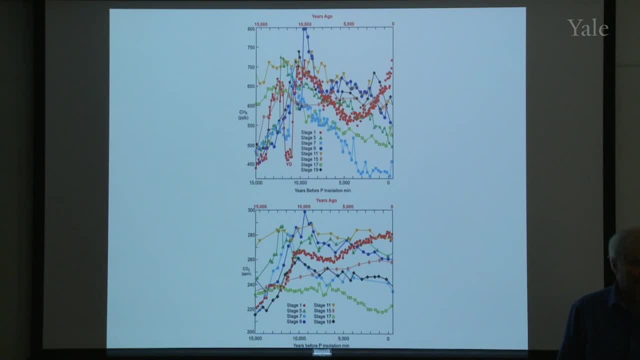 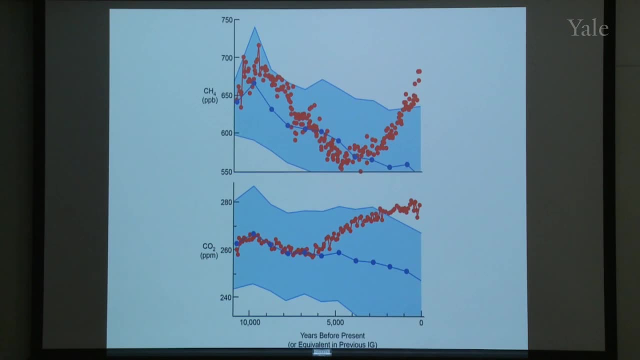 is questionable, But that's a lot of information for your eye to take in. So a few years ago I thought let's lump all those previous interglacials together and compute. this is the same kind of time scale relevant to the Holocene, So you could lock your time scale. 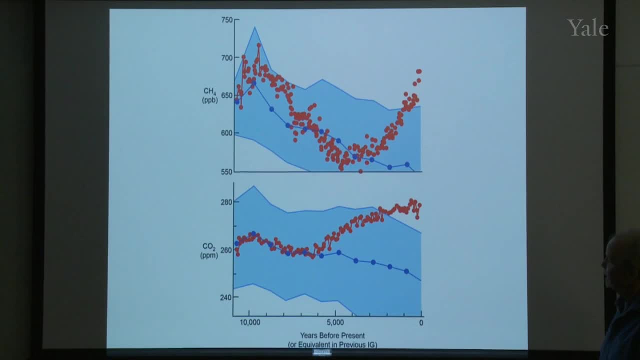 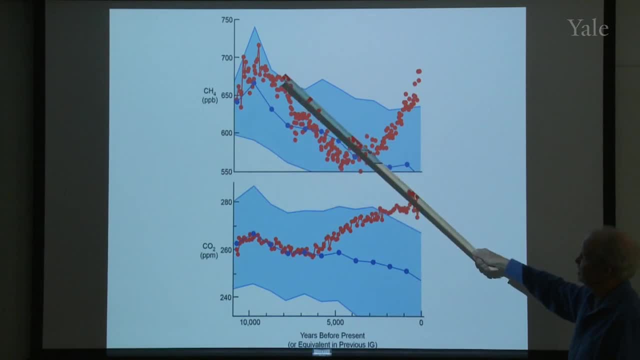 this is the standard deviation. You remember. some of those curves would come up higher and kind of drift down lower. Some came up not as far and drifted lower. So most of the scatter is due to that. Methane, like some other interglacials, is a little bit. 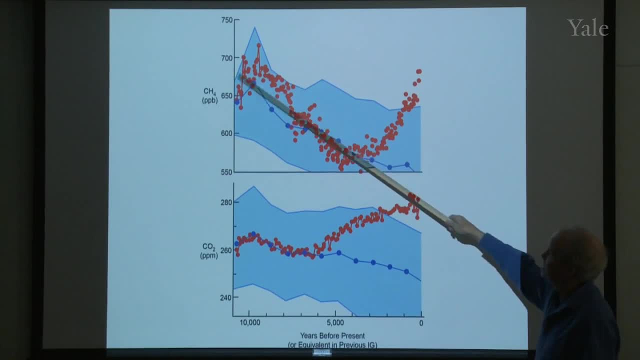 higher than the stacked average, although it's within the standard deviation, Comes down faster than the stacked average until 5,000 years ago, And I think I make the claim that downward is natural because that's what always happened on previous interglaciations. 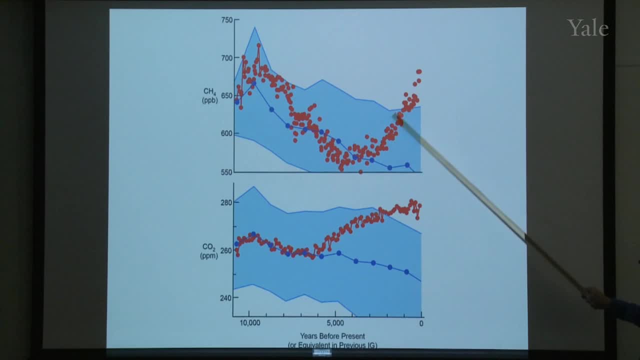 So very dramatically 5,000 years ago. methane takes off And by the last 2,000 years it's outside The envelope of variation of the previous interglacials CO2 is the same story Now. this is amazing overlap here, but individual CO2. 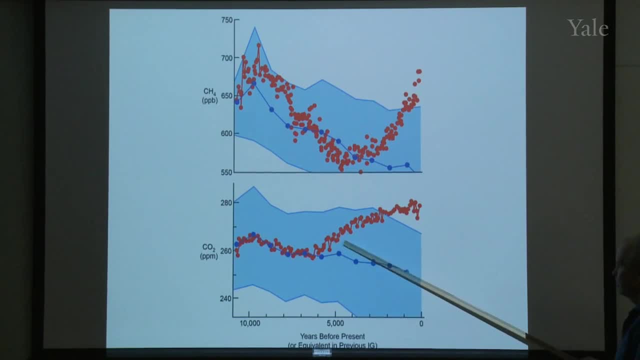 trends on those interglaciations. Some of them are up in here and then come down. Some of them are only up to here and come down. So I would say this is maybe the more typical case, but it's the same thing. 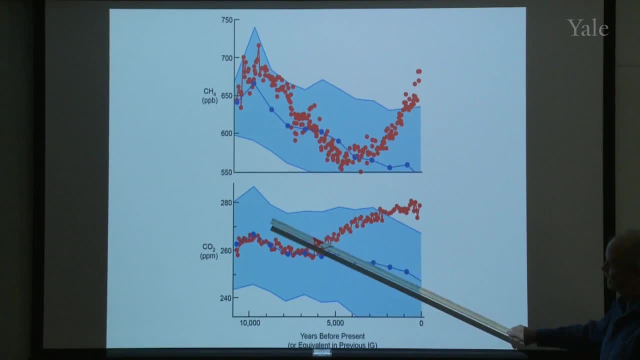 CO2 is close to the average, in this case well within the standard deviation. And around 6,500 years ago, 7,000 years ago- you get this what I call wrong way trend. Both of these are wrong way trends. 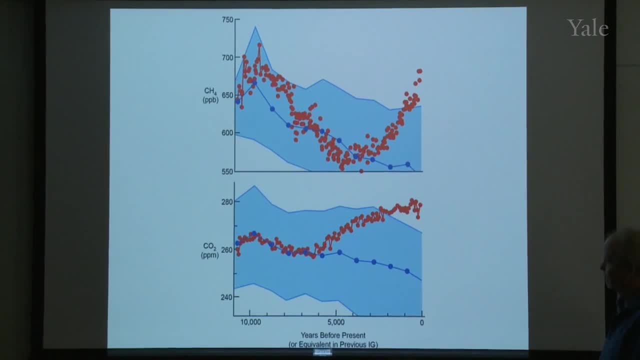 So if? Is that one sigma or two sigma? One sigma? So if downward is natural, I mean the whole first part of my hypothesis is: if downward is natural, these are not natural, And not natural is in my mind equivalent to: 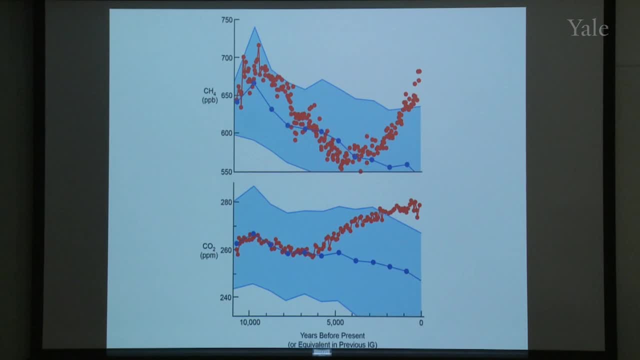 anthropogenic: Yes, For the modern data is zero. 1850 or 1750?? Oh yeah, this is pre-industrial. Looks like it goes to zero, but it goes, actually goes to 18, actually not quite, I think 1800 in this case. 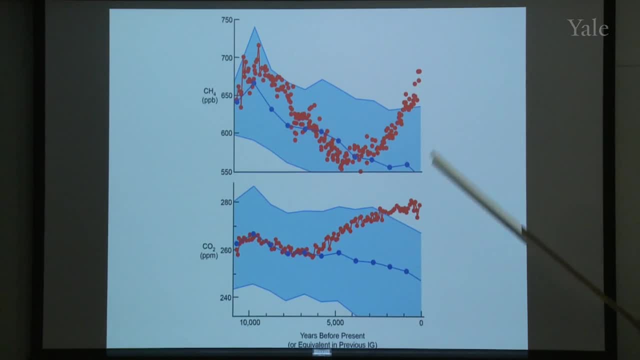 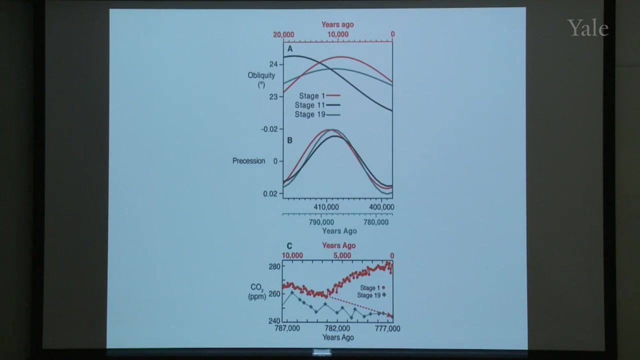 CO. methane gets up in here just before the industrial era. CO2 is about in this range just before industrial times. So downward is natural, upward is not natural. Now one of those interglaciations, stage 19,. I pointed out that 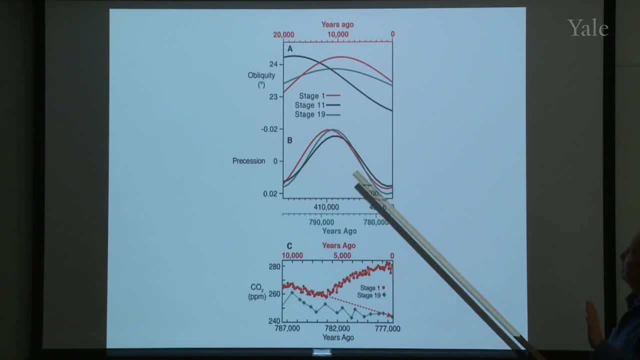 anomalous methane pump. Let me back up Early in the evaluational hypothesis. one of the major criticisms was that people started looking for analogs. What's the best analog for the Holocene in terms of insulation, And the one that was put forward with stage 11, and the reason it was put forward? you? 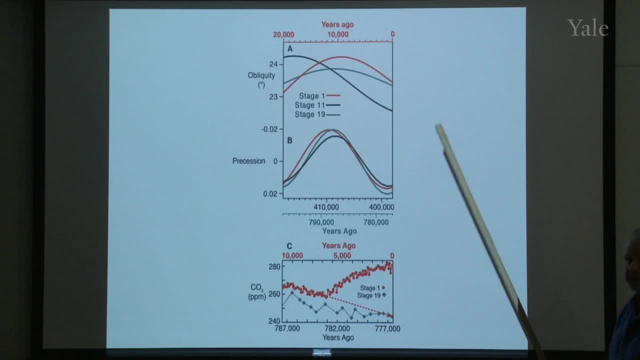 can see here, the red and the black are very similar in amplitude. Some of these other interglaciations: the amplitude of the precession effect gets much higher and gets much lower, but these are very close in amplitude. People say, well, that's the best. 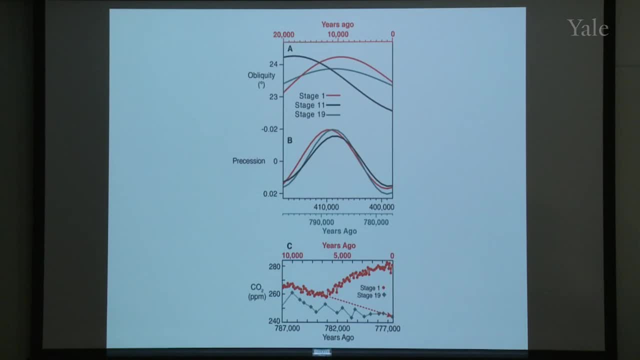 That's the best analog. That was back when the ice core only got back to about 400,000 years. Subsequently they go back to 800,000 years And that brings into play stage 19,. just after 800,000 years ago. 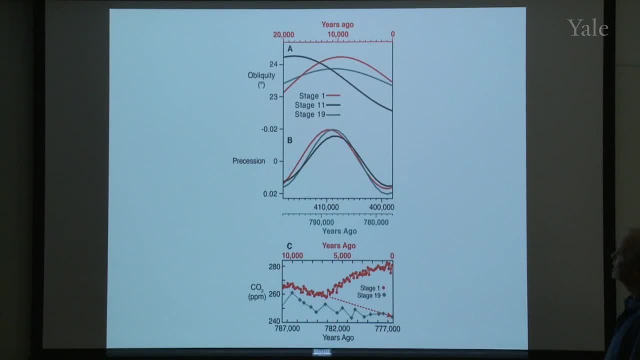 And it also has an amplitude that's very, very close, just as close, at least, to the Holocene as stage 11.. So now you have the two possibilities for analogs, But the only criticism was all focused on precession and ignored obliquity. 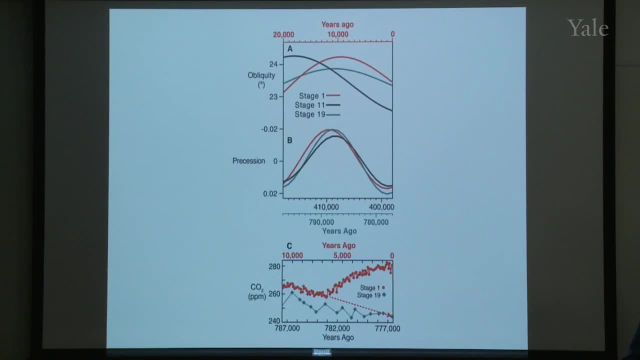 And all the science I'm aware of says you can't ignore obliquity in things like growth and decay of ice sheets. You've got to consider both of them. And so look what happens with obliquity. Stage 11,. these are aligned relative to these time scales, but also relative to each other. 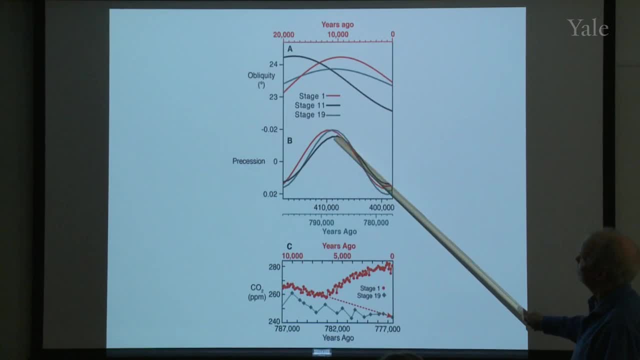 If you align stage 1 and 11 like this, then obliquity has a maximum way over here in stage 19, and much later in stage 11.. So stage 11 is not a good insulation. analog Stage 19,, in contrast, has its maximum at the same relative position. 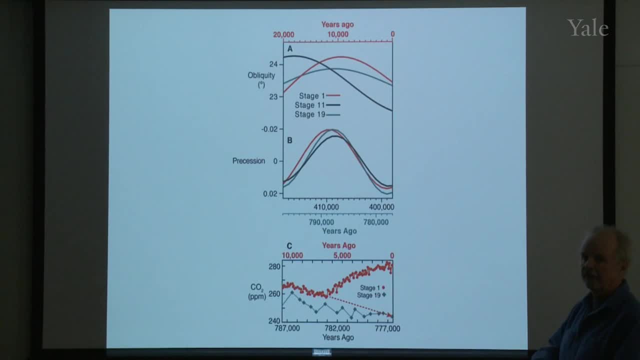 It's lower in amplitude. So that's the one shortfall of using that as an analog. There is no perfect analog, But it's much better to have some amplitude mismatch than to have a complete offset of relative timing. So stage 19 is now accepted among people who are paying attention to the problem as the best orbital insulation analog. 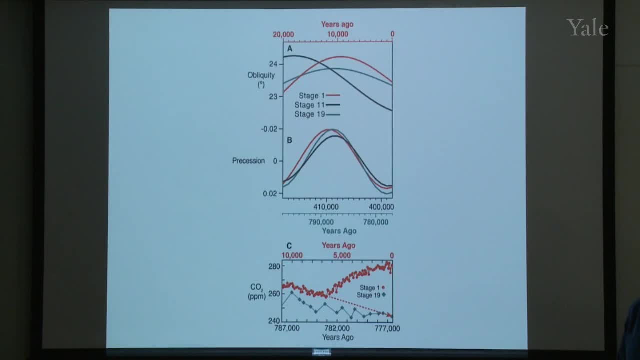 Now that's interesting because you could go to the ice core And CO2 is most important greenhouse gas in terms of anthropogenic impacts on the atmosphere. Here's that stage 1 high resolution trend- again You've seen it before. Here's stage 19,. much lower resolution, so it's not capturing the full signal. 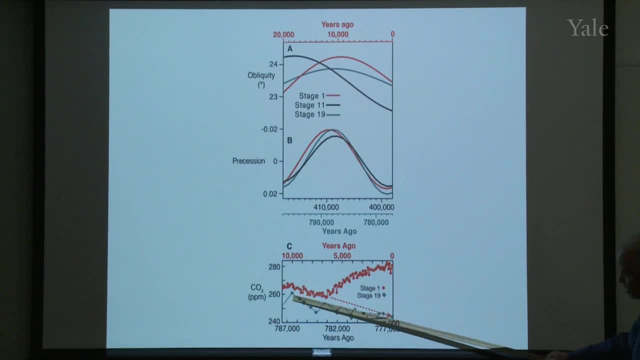 Peaks are very similar Downward trend. this one goes down faster. Here's that reversal in the Holocene. But look what stage 19 is doing. It continues down and it ends up at a point around 245 parts per million or less. 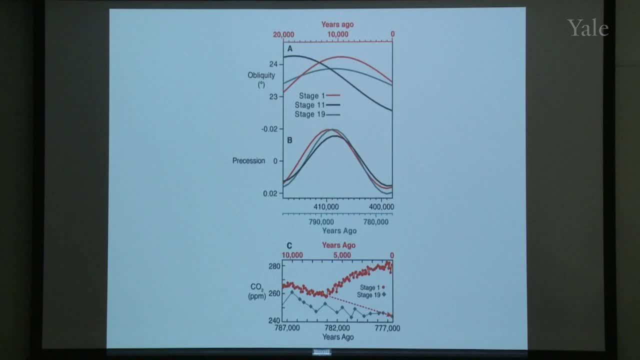 whereas in the Holocene it's 280 or more. Now, with the original hypothesis and not having all this density of data, I projected, or I estimated, that the value in the Holocene, today that is, would be between 240 and 245. 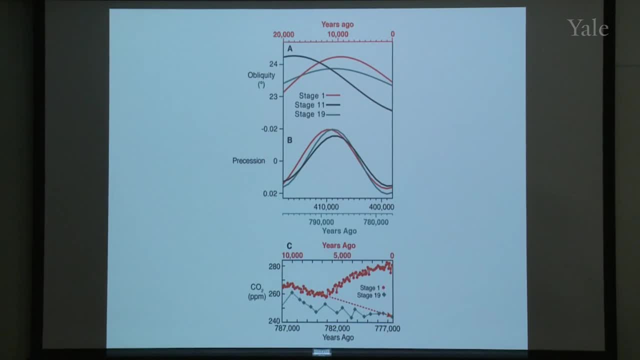 So I projected that kind of a value And I'm feeling pretty good about that estimate right now. So a natural experiment that nature has run gives you the CO2 value that the early anthropogenic hypothesis would suggest. Now, if you take. if you take, this is for stage 19,. 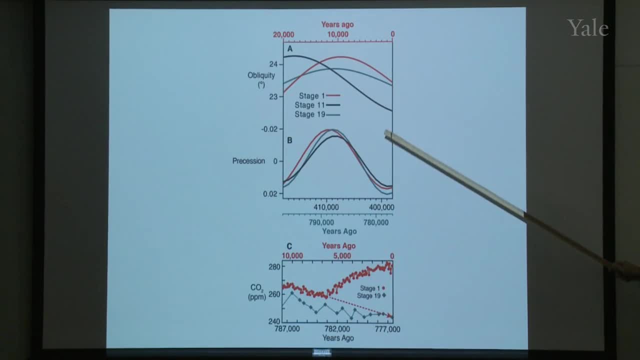 if you take the observed obliquity value, precession value and CO2 value and the methane value and run a climate model experiment, it obviously gives you a colder Earth. It's not much difference up here, but 40 parts per million of CO2 is a big difference. 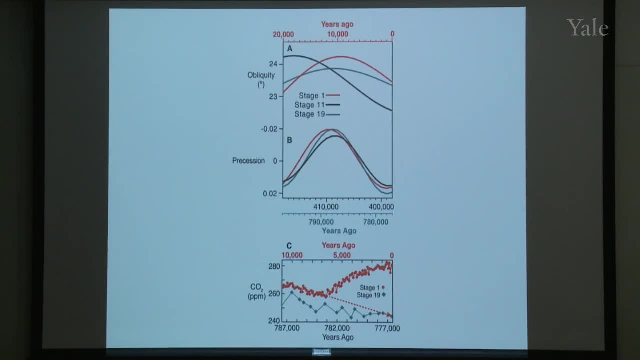 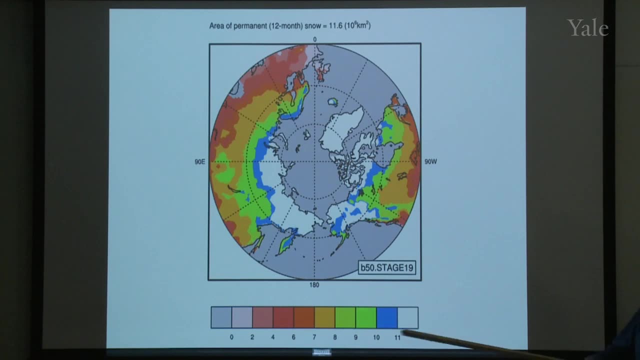 That's half the glacial-interglacial signal, almost So it gives you a much colder Earth. and on that colder Earth, in the kinds of models, that full general circulation models, you can't run an ice sheet, a coupled ice sheet. 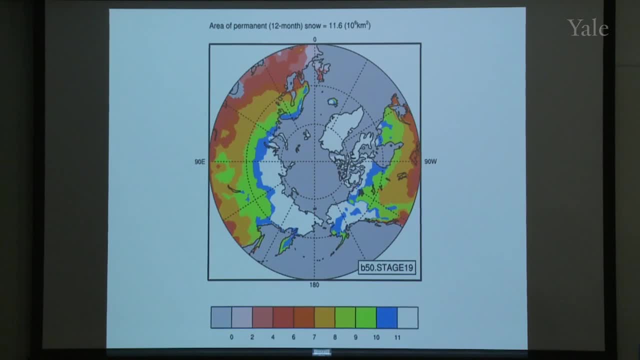 because it's too. the model has such complexity it can only run for decades, unless you have a lot of money. So, but what it can tell you is what are the areas where the snow cover doesn't ever melt in the summer? 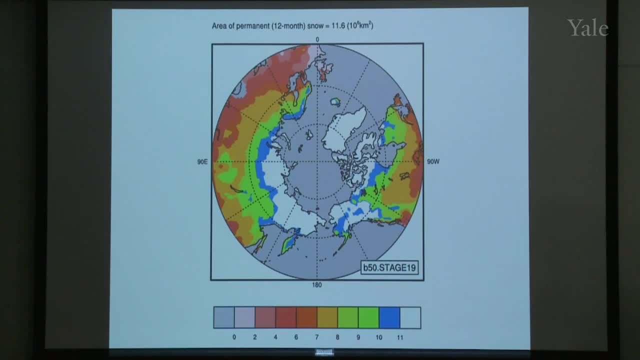 And, by definition, if you get through the summer and get into September with snow on the ground, it's going to get added to the next year and the next year, and the next year. So those are areas that my co-authors. 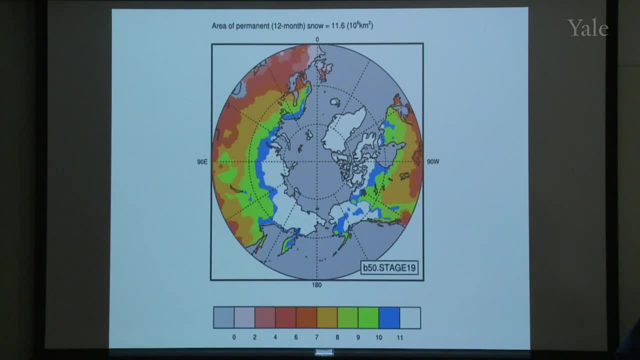 John Kutzbach, that Harvey mentioned and I say are areas of incipient glaciation. Those are areas that should get an ice sheet of some size and thickness if the model could run long enough. Big chunk of northern, northeastern Siberia. 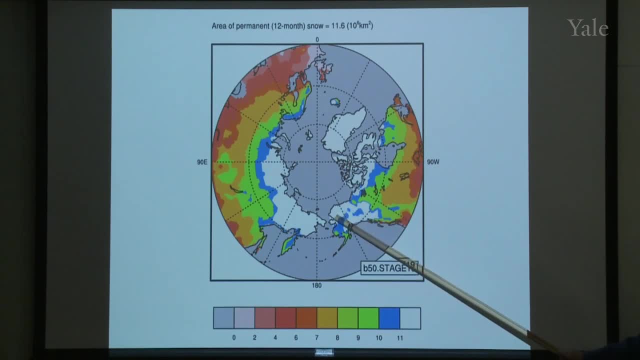 northern Canadian Rockies, Brooks Range, the Canadian Archipelago, Baffin Island. just to give you some scale, Baffin Island is about the size of California and Oregon. put together, Oregon, sorry, So those areas would all be going under glaciation. 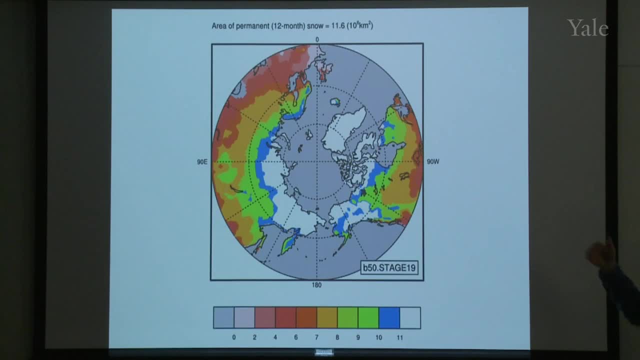 Of course, Greenland's already there, so it's just going to get a little more glaciated. So stage 19 is telling us that there should be a small glaciation underway, which is also a part of the original early anthropogenic hypothesis. 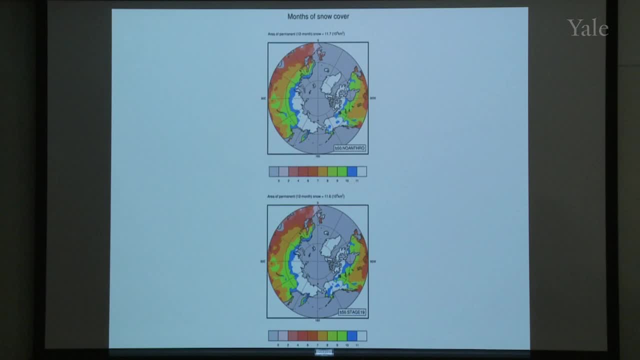 Along that same line of thinking. here is that's a repeat of stage 19,. let's see, this is the repeat of what I just showed you. It's hard to tell them apart. and this is this is a run. 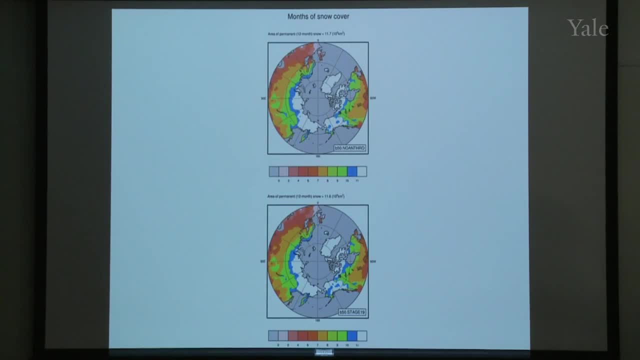 a simulation for the projected greenhouse gas values according to the early anthropogenic hypothesis. There's almost no difference. so stage 19 is: is the nature's test run of the early anthropogenic hypothesis. I think the biggest differences, I recall, is a little. 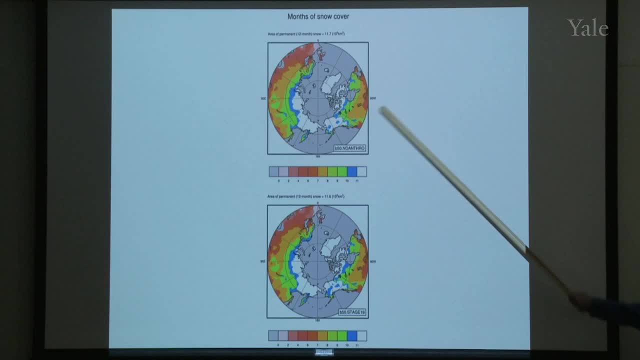 a little bit in the Alaska, the Canadian Rockies a little more. a little more snow cover up here, but not enough to worry about. So the looks like the Earth would be glaciated in these areas. not big ice sheets down in Chicago. 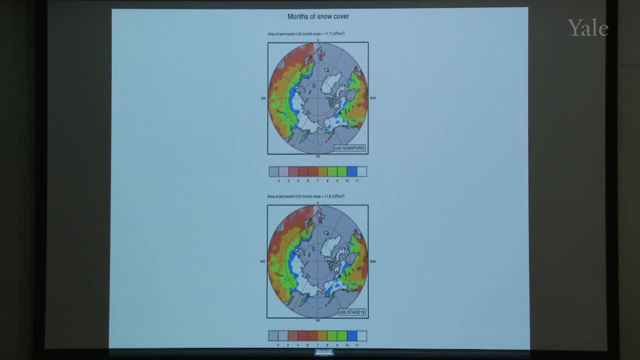 or anything like that, just small or medium-sized Greenland-sized ice sheets or ice cover starting to thicken. That and that's really upset people because it just sounds so unlikely we would actually be in a natural glaciation. But there's a. 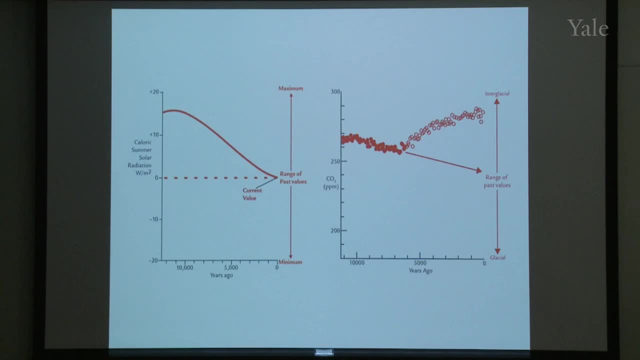 there's a way to look at it makes makes it sound pretty reasonable. Here is let's see which one should I do first. Okay, this plot shows caloric summer solar insulation, which is the in the northern hemisphere. 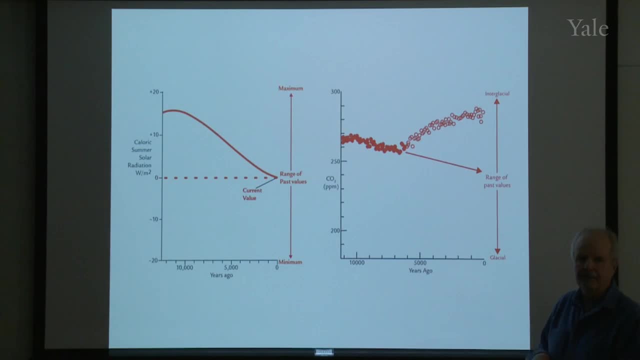 That's the one Milankovitch used in his theory back in 1941.. And here's the range of values from maximum to minimum insulation over the last half million years. So cycles don't always go to the full maximum, full minimum. 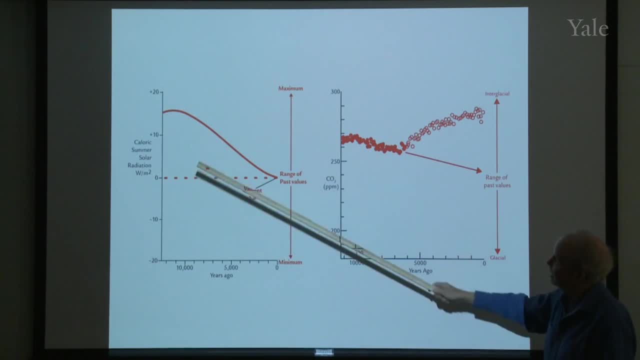 Some of them are smaller, but that's the full range. Here's the value, actual value, 10,000, 11,000 years ago. Here's the current value. So you're almost exactly halfway to a full, to the lowest extreme. 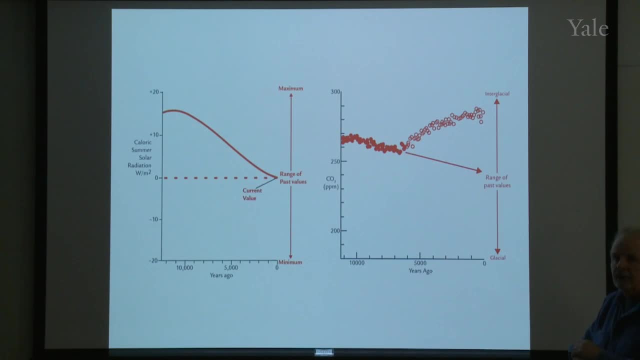 of of the insulation And that's certainly a push, but a plausible push- towards glaciation. Here's the CO2 value. You could kind of ignore the methane value because it's it's forcing a climate is much smaller, but it adds to the story. 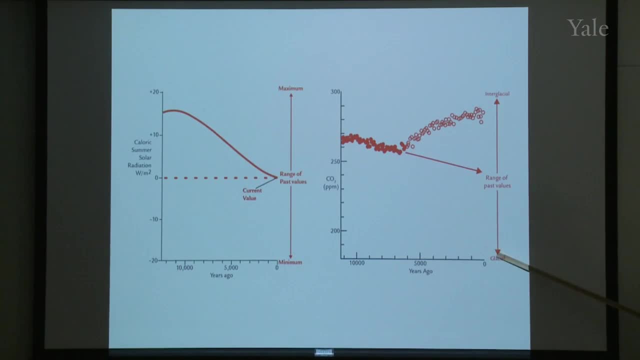 Here's the variation of CO2 over the last half million years- interglacial, glacial- And here's that downward trend and that projection that I mentioned earlier. You end up if you count in the methane. you end up about halfway again. 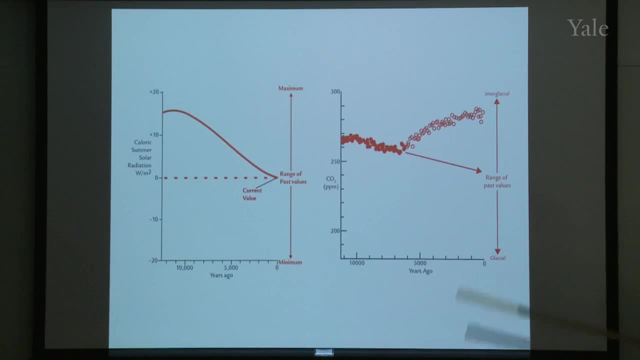 So you're, you're more, you're halfway towards the lowest values that push the fastest growth of glaciers. So it's it's not surprising that you could be getting the beginning of glaciation, if you look at it that way. Quick. 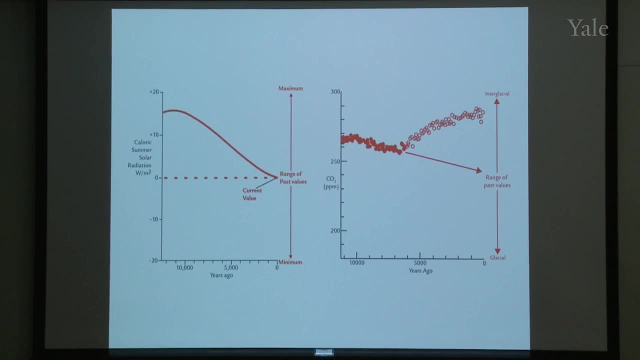 quick question. So on the previous slide, you you wanted us to focus on this Baffin island thing, for just because it's for scale, Wasn't that, wasn't that thought to be the seed of the of the Laurentide ice sheet? 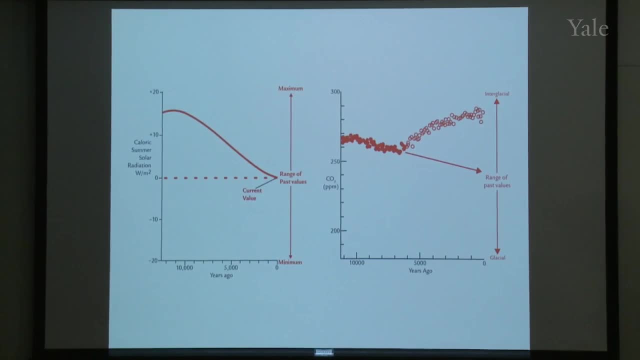 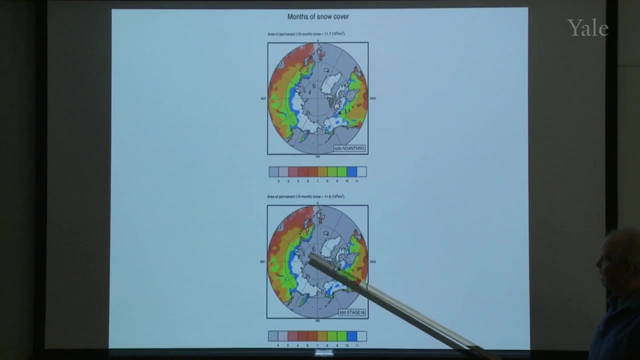 I mean, one idea was that the penny glacier there on the on the Baffin island was the seed for the for the Laurentide ice sheet. Is that important to your argument or not? No, not really, but there are different arguments. 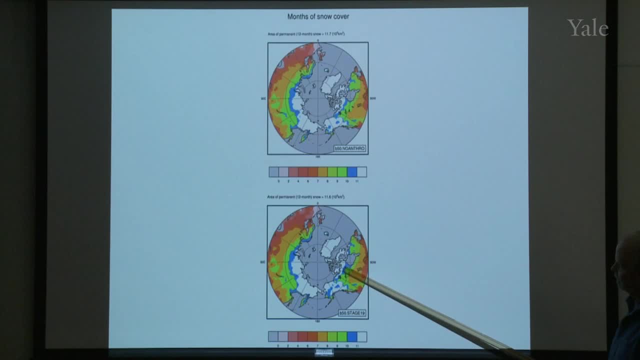 That's again. that's Baffin. There are some there. there's a number of hypotheses go back 40 years now. I think that do talk about that. the Laurentide comes out of this, this region. Some of them put it on Baffin. 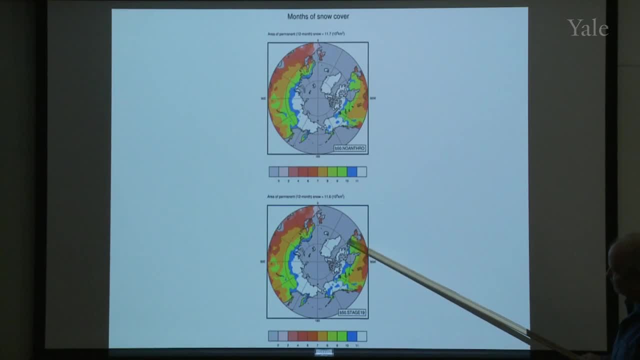 Some of them put it even in northern Labrador, Some of them put it up towards the archipelago. So that's, that's a, that's a part of the literature. that's not inconsistent with what I'm saying, but I'm not stressing it or leaning on it. 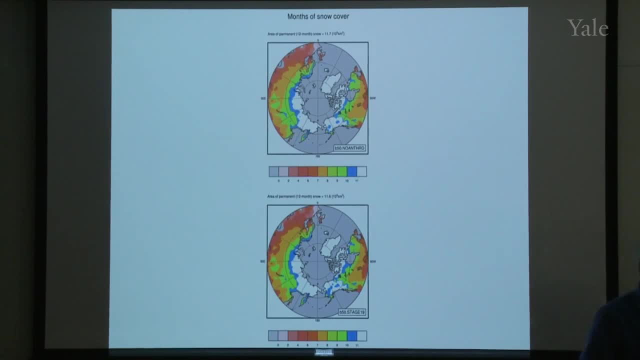 or I don't need that for my arguments. My, my question, though, is that northern Siberia, in some of the early reconstructions- of reconstructions of where, where the ice sheets had been, had been- didn't have as large an ice sheet? 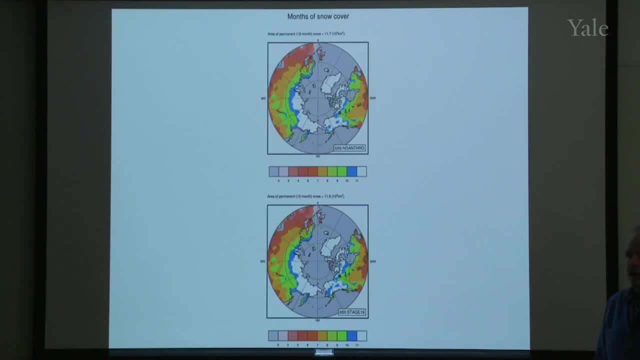 That's where the mammoths were. were were stuck in Rangelia, for instance. That's, that's correct, But here it looks as though you're going to develop a, a land, a land, ice sheet, The. 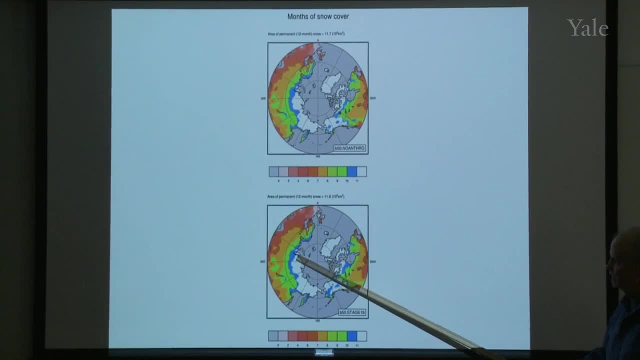 In that in that area, that's, in the rain shadow of the Himalayas, The evidence from a number of studies over the last few decades is that at the last glacial maximum there's no, there's no massive ice sheet in Siberia. 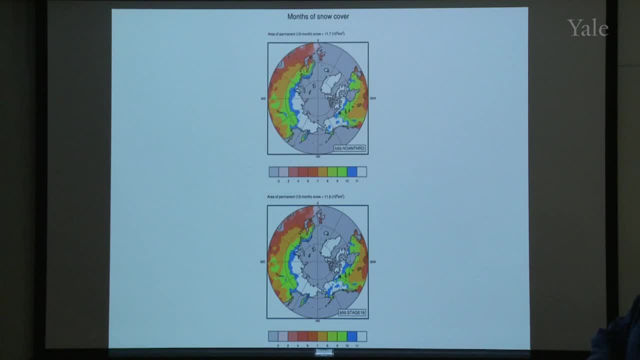 There's a number of smaller ones scattered in through there, but there's no massive ice sheet. But by the time of the last glacial maximum Siberia is much drier than it is in the early growth phases. And there's there's scattered evidence. 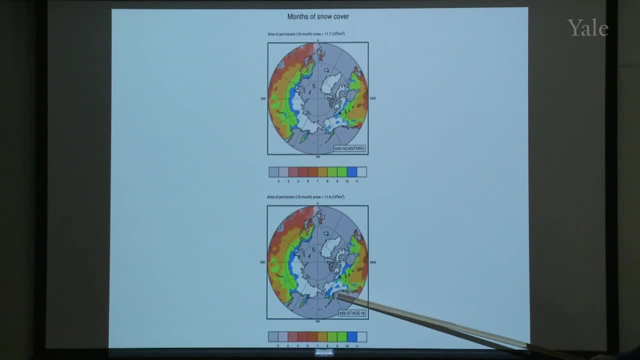 for instance, along the coast of Africa and along the of Siberia and the coast of Alaska, There's scattered evidence for new ice sheets draining into the ocean, So there was almost certainly more more snow, And there've been people who've said there were larger ice sheets. 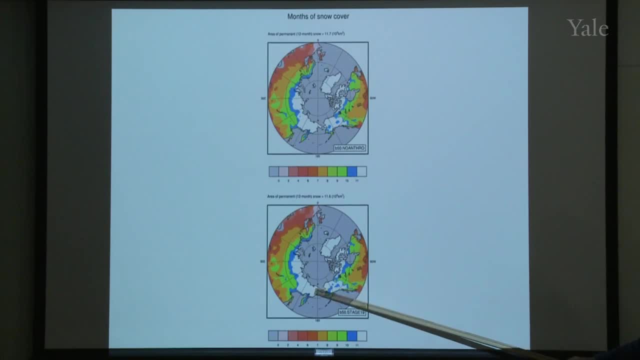 still not Laurentide size, but larger ice sheets early, because it's there's air. you know, air masses with more moisture are making the trip from the Atlantic or from the South. So it's not, it's it's. 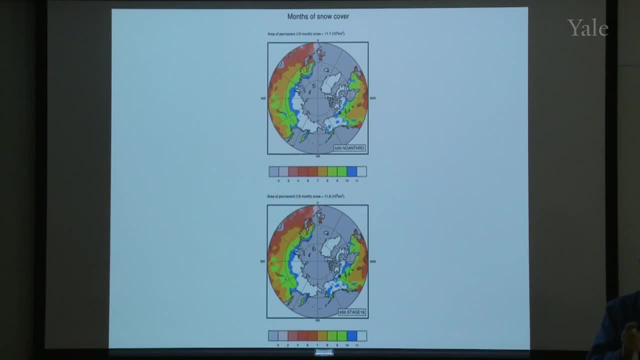 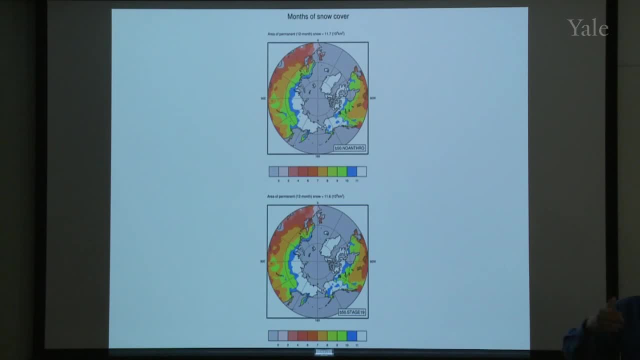 it's, it's, it's, it's, it's very, very, very, very, very obscure. It's a, it's a, it's not a, it's not a misprediction, unless you think it means that that. 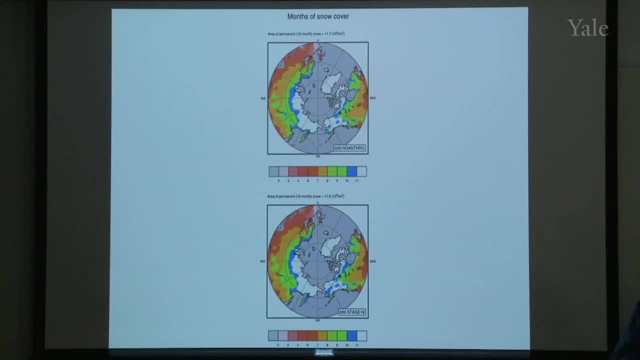 that's going to grow up to be a continuous ice sheet at 20,000, and it didn't. and the reasons? the region. the reason would appear to be that it got starved for moisture, and that's been in the literature for a while. 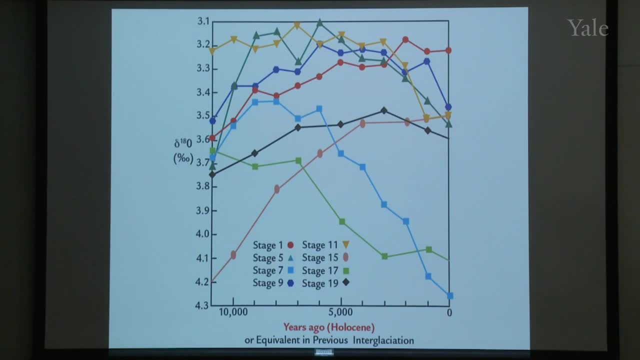 Okay, Okay, Oh yeah. I just this, this, I just re the Laseki-Ramo stack of oxygen isotopic values from the Atlantic and the Pacific deep ocean And I thought, well, I should do the same kind of thing. 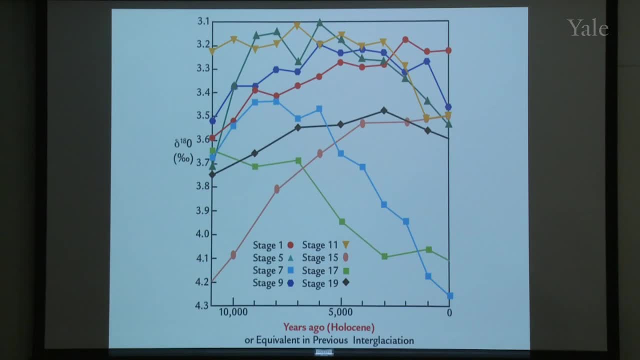 that I did for the greenhouse gases, And it's a little different in that the way this timescale is tuned. it's tuned under the assumption that the O18 record, which is a record of mostly ice volume but also temperature, lags behind the insulation forcing. 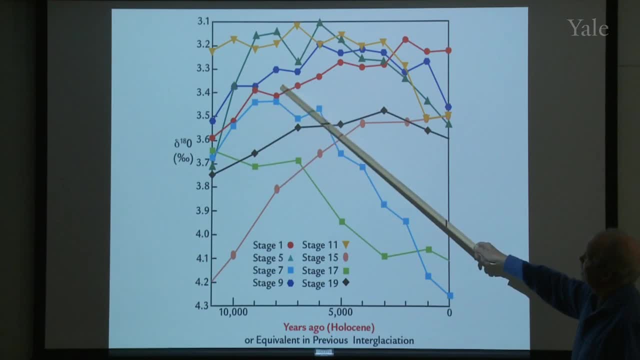 So what these curves do is they give you deglaciations up till about the equivalent of about 6,000 years ago, on average, And then you see that most of them start to turn around at some point in that sequence, Again, the Holocene looks different. 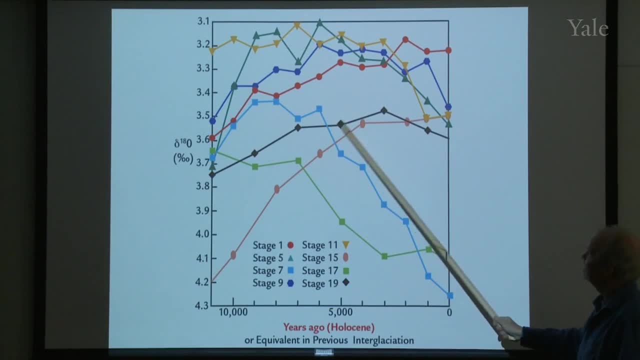 It doesn't turn around And again, stage 15 looks different. It just keeps rising and it's still rising at the end of the record. That was the one that gave you that anomalous CO2 plot, So we could talk about that later. 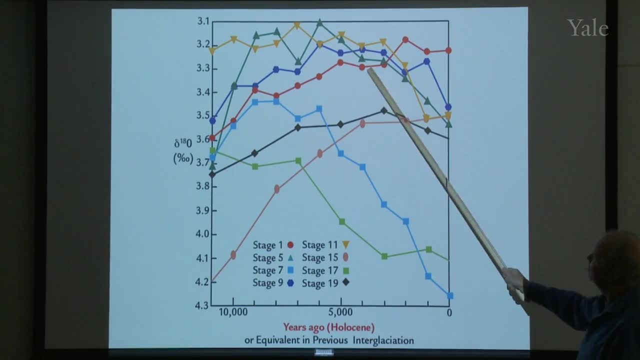 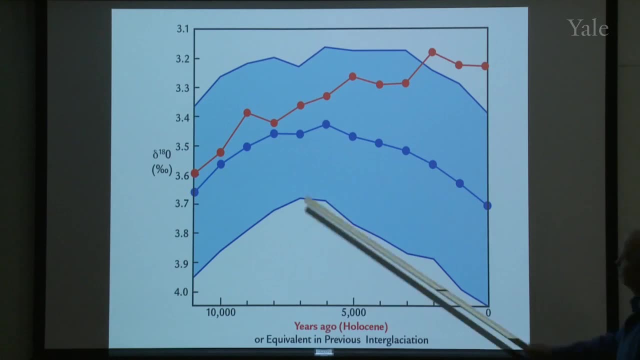 So there is a similarity in these trends and most of them are not like the Holocene, And if you do that same stacking exercise you get a pattern that looks like that. Here's the 6,000 years ago Ice volume, temperature minimum, the most. 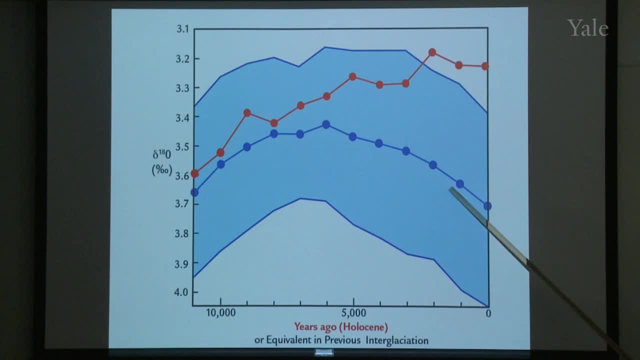 interglacial climate state, And then the average is going steadily towards a more glacial state for the last 6,000 years. Holocene is running along looking like that until somewhere in about here and then takes off in the ocean. 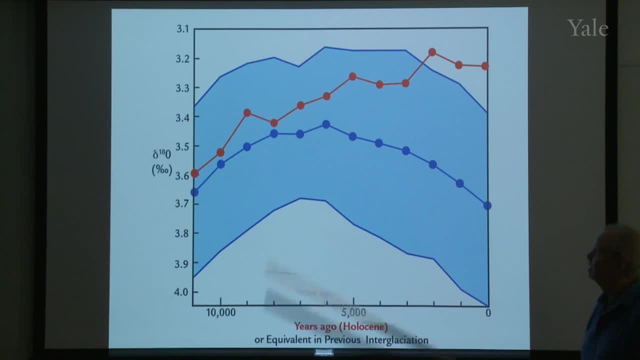 We don't think there's any major melting of ice sheets going on here to drive that curve upward. So it would seem to be. It's just a warming of the deep ocean. So that's just when the CO2 curve starts to depart from normal. 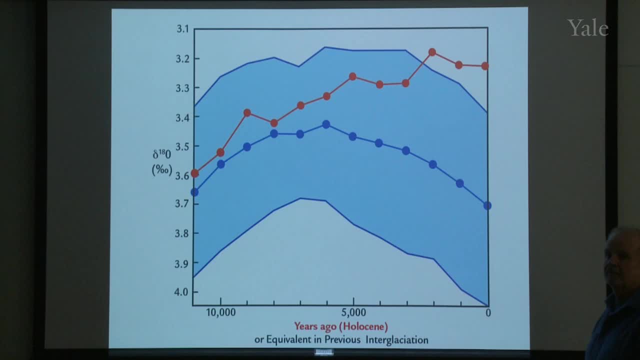 And CO2 curve. if it warms the atmosphere- because it keeps rising and that's anomalous- it'll warm the deep ocean as well. So that is consistent with the greenhouse gas information. Is there a question? RICHARD SCHMALENSEE? Yeah, 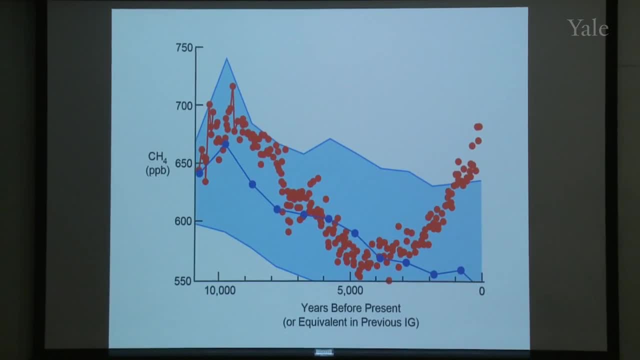 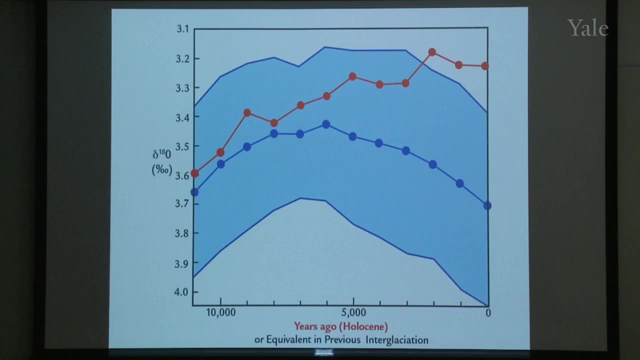 Just to go back to that image that you did. please let me know what you mean. Let's see What am I doing here. Who Who's? No, the next one. Sorry, I'm too forward now. Thank you. 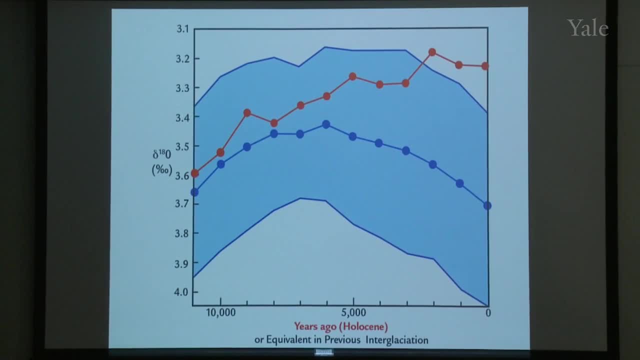 So just to please remind me what the chronology when people think the Laurentide Ice Sheet collapsed as well as the Tuscandian RICHARD SCHMALENSEE. OK, The Laurentide Ice Sheet, I won't use the word collapse. 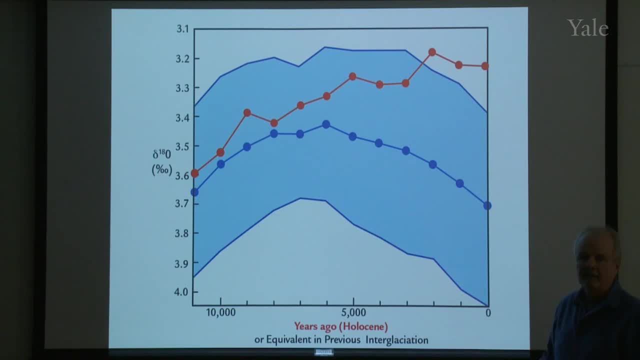 but it started melting. It started melting 17,000 years ago And there's plenty of glacial geological evidence that the last little remnants of it melted between 7,000 and 6,000 years. It's just a tiny little fragment up in Labrador. 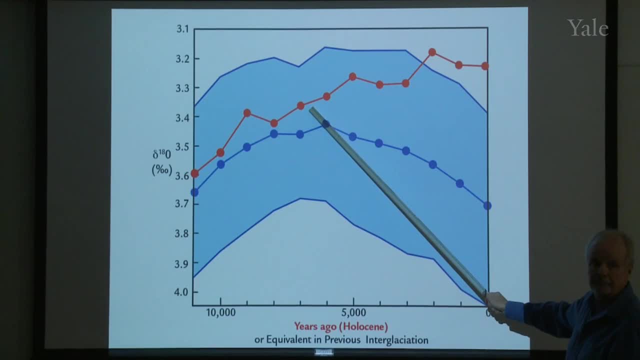 So it would be in about here, which is right close to the other curves, reaching their minimum ice extent. So just to say that there's something anomalous about the oxygen isotope curve in the Holocene and it's anomalous in much the same way. 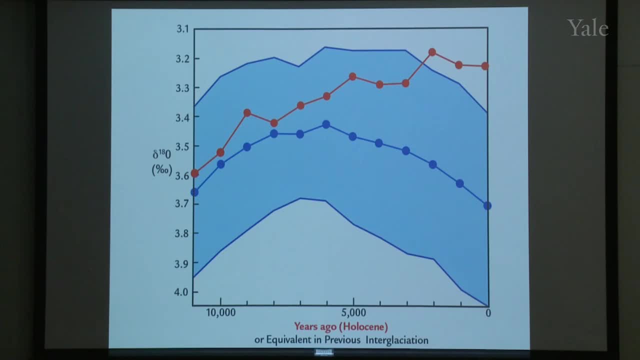 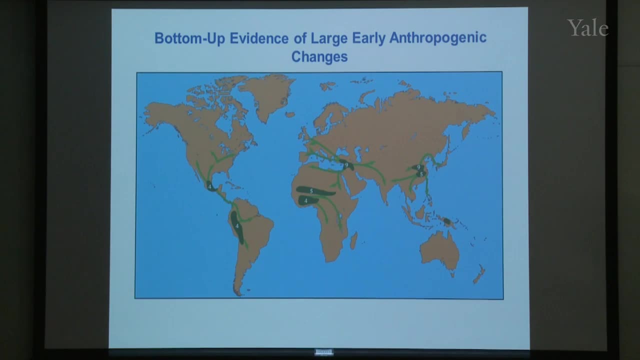 as the greenhouse gases and it's anomalous at a time that the greenhouse gases could be contributing to it. So that's the first body of evidence. I would make the claim and I don't convince everybody. but if the Holocene is that anomalous, if down is natural, 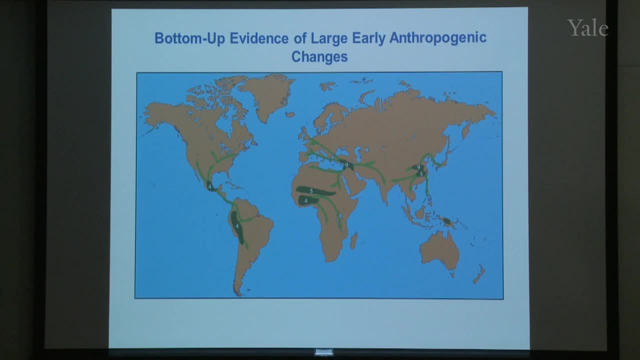 and up is not natural. And what can you think of as not natural? Well, it's humans. I think this is powerful evidence. I don't see how people can argue against it, But it doesn't convince everyone, So that's one reason the hypothesis is still lingering. 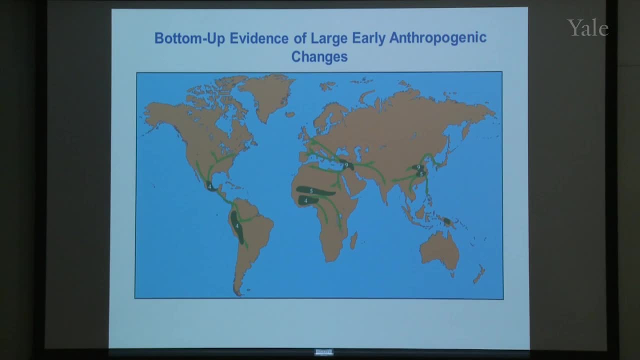 The other kind of evidence which I call bottom up, because at the time that the greenhouse gases are behaving anomalously, humans are. They're coming up with domesticated crops and animals. These numbers in white are in thousands of years ago and they mark the time when domestication, which had already 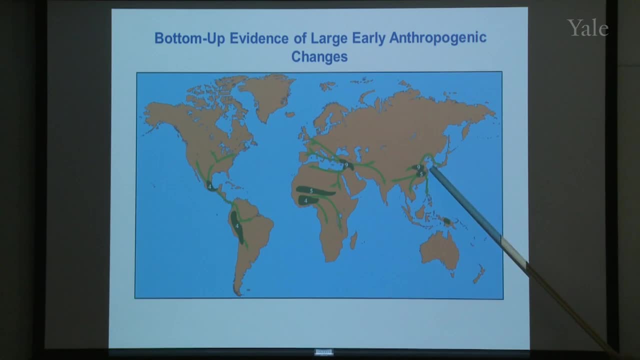 occurred begins to spread. So 9,000 years ago in northern China, 9,000 years ago in the Fertile Crescent, the original domestication goes back farther, 5,000 years ago, for rice out of south central China, 5,000 years. 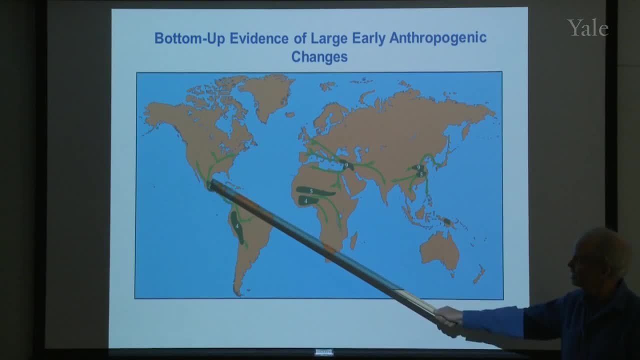 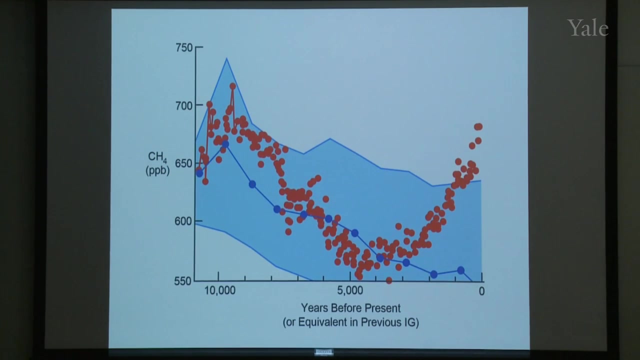 ago in Africa, 4,000 years ago in Mexico and Peru. So the whole time that these anomalies are getting stronger, agriculture is spreading And agriculture can affect both methane and CO2.. So I'll start with methane and remind you that it's 5,000 years ago that the methane 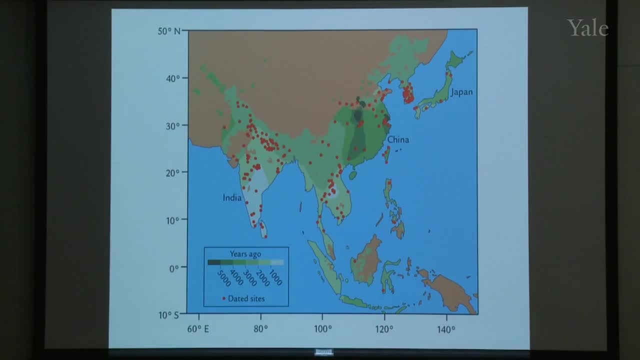 trend goes the wrong way. This is a compilation that just came out three years ago. two years ago, no, three years ago. Dorian Fuller University, College London. All the red dots are data points. carbon-14 dated data points. 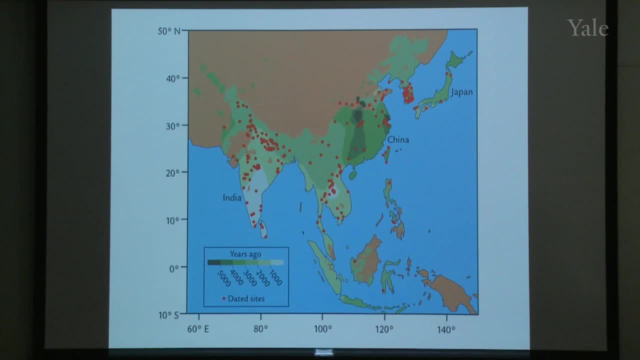 showing the first arrival of irrigated rice into all this area of southern Asia. And the reason irrigated rice is important is that the rice patties are basically swamps. You can think of them as human-made swamps, And in the rice patties the water's not circulating. 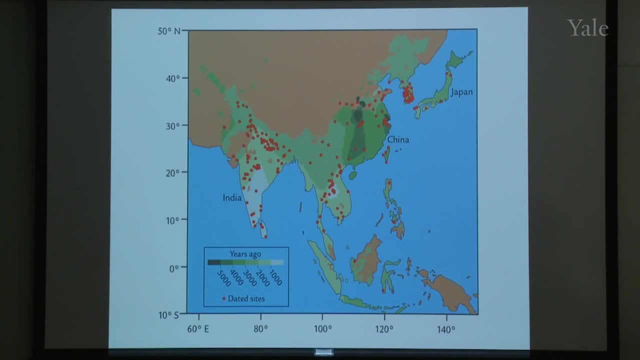 It's just sitting there and it's keeping the feet of the rice in the water so that it'll grow fast. And methane: there's enough carbon in the patties that it strips the oxygen out of the water. And what comes out? 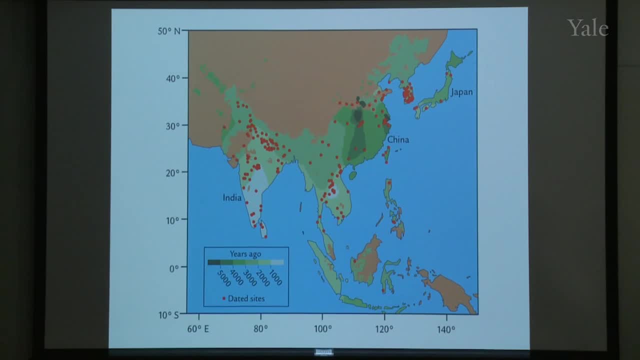 After that, After that is methane, which is the same thing you get if you're looking at a stagnant pool or pond, or swamp. We would call it swamp gas, at least in some parts of the country. So this is the spread of man-made swamp gas. 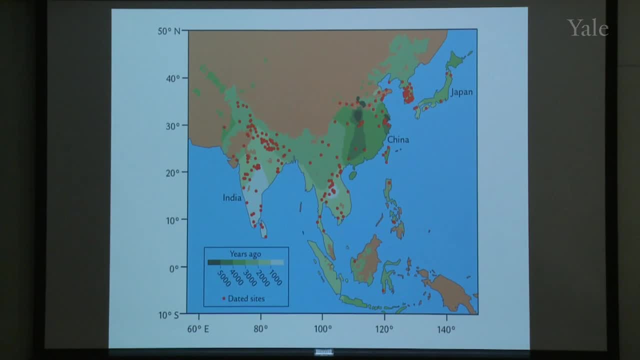 producing methane across all of southern Asia Starts around 5,000 years ago in the Yangtze River Valley, where the domestication occurred, And by 1,000 years ago it's basically spread everywhere that it's going to spread or where it's farmed today. 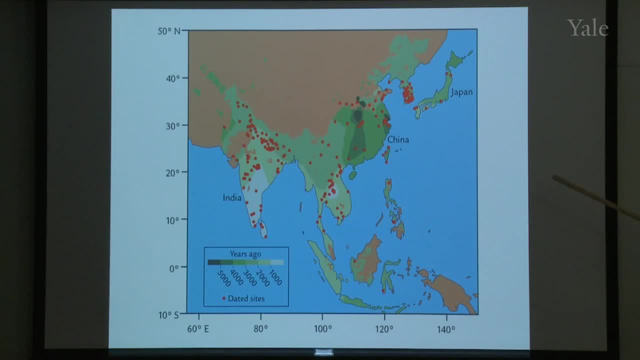 So Dorian Fuller took these times of first arrival of irrigated rice into these areas and then applied a model in which he assumed that the rice growing would densify. I always have trouble with this. I have trouble finding a word. It would cover the landscape progressively. 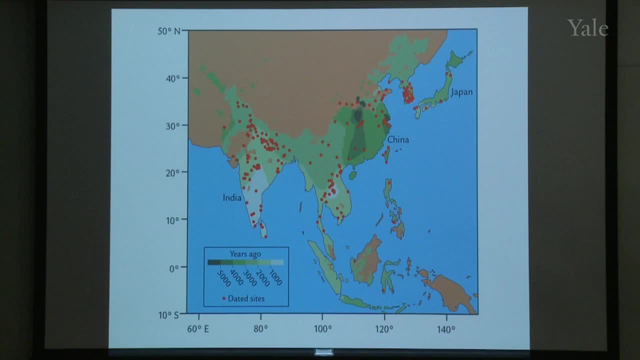 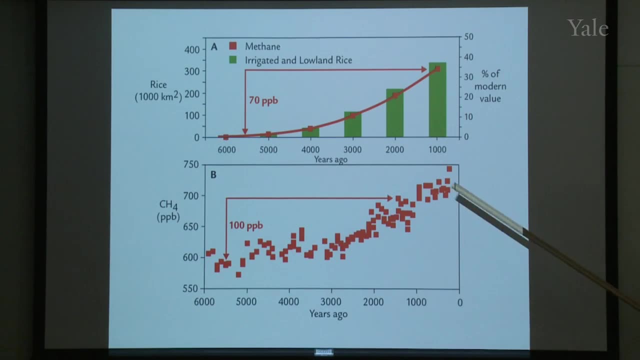 from just a few rice patties to the modern sprawl of rice patties And he came up with a plot of the upward trend in irrigated rice farming as a percentage of the modern value. It was nothing at 6,000 years ago, a little bit at 5,000.. 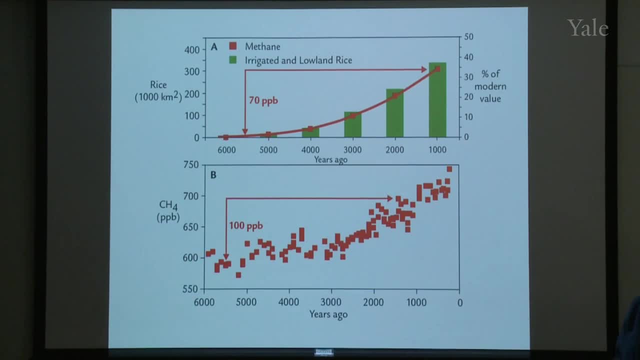 And, mind you, that's just when the methane trend starts to go the wrong way. And from that he calculated using the methane, using the irrigated rice area and using modern relationships between irrigated rice area methane emissions and methane concentrations in the atmosphere. 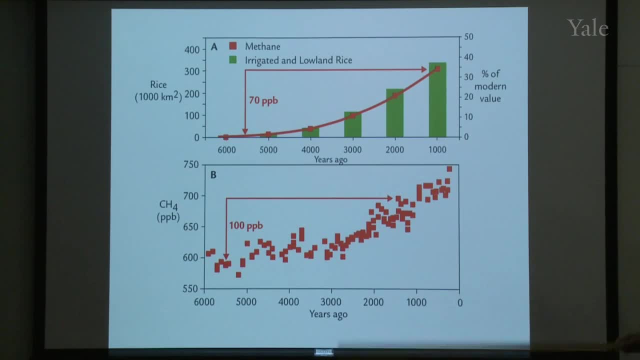 He calculated. He calculated a methane curve doing that over the time between 5,000 and 1,000 years ago, And here's what the ice core says that it did. So he calculated 70 parts per billion. The actual concentration rose 100.. 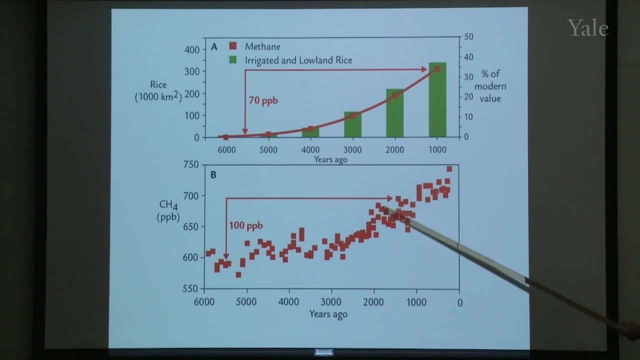 So the rice irrigation is explaining a good chunk of this rise. But there is an added factor. You remember the natural trend of methane? It was something like this. It was going down all the way from 10,000 years ago straight through to today. 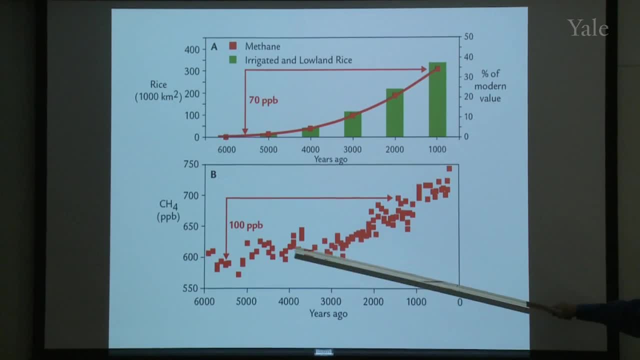 So the methane anomaly is not just the increase, It's the fact that it didn't decrease the way it should have. So you have to factor that in. So this 70 parts per billion is a smaller fraction of the observed 100 parts per billion than you might think. 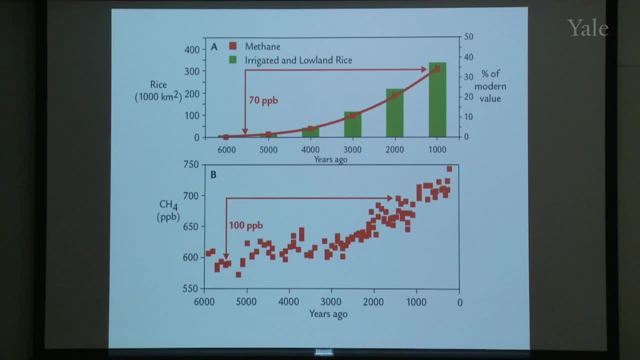 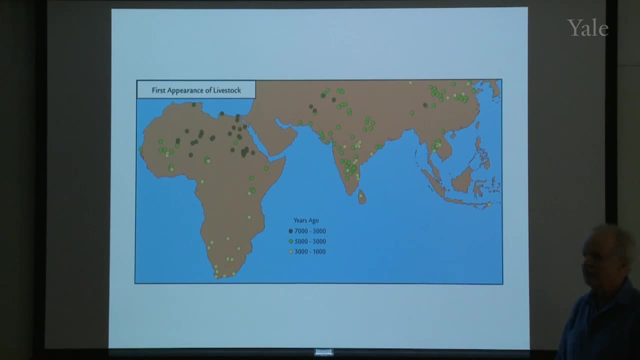 There was a question- and I'll pause in a minute and take it Fuller- also mapped the spread of livestock across the continents for this interval: 7 to 5,000,, 5 to 3,, 3 to 1.. 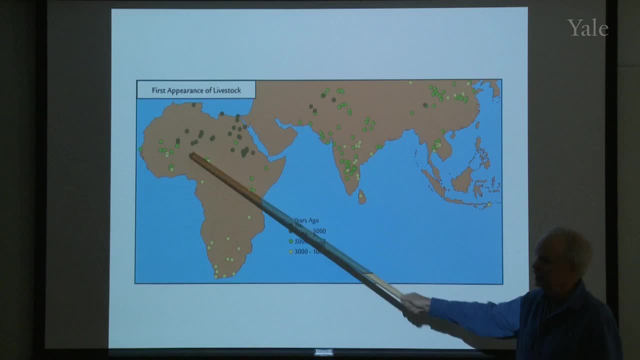 And if you go back 7 to 5,000 years ago, there are livestock in the Sahara, where the valleys are in many cases grasslands, because the monsoon is running much more strong, And a little bit in the Iranian Plateau. 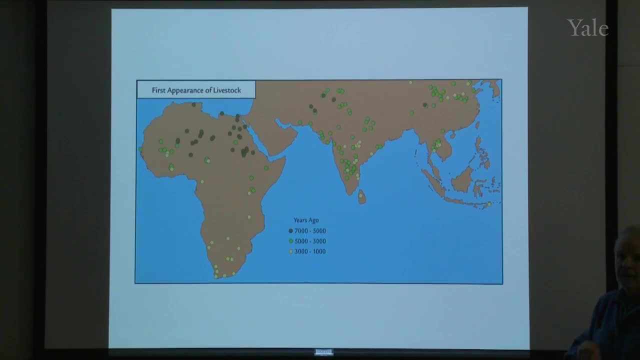 and some in Western China, which is a very arid region. These are not forested areas, They were not and they are not. So there's cattle and other livestock, But the land has a low carrying capacity So it's probably not that many livestock. 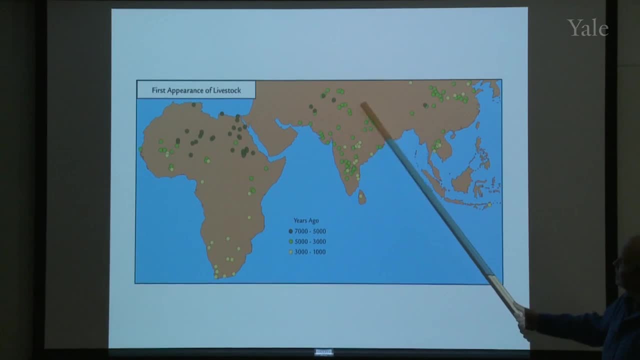 By 5,000 to 3,000 years ago. you're getting into India and China in areas which are naturally forested, So if you've got livestock, people have to clear the forests to allow livestock to feed And the carrying capacity in these wetter areas. 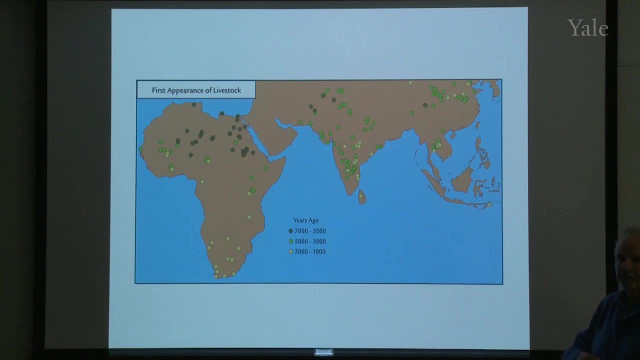 is much higher. So once livestock gets in there there can be high density on the land. So livestock spreads down into India, over to Eastern China and all the way down into Africa by 3,000 to 1,000 years ago. 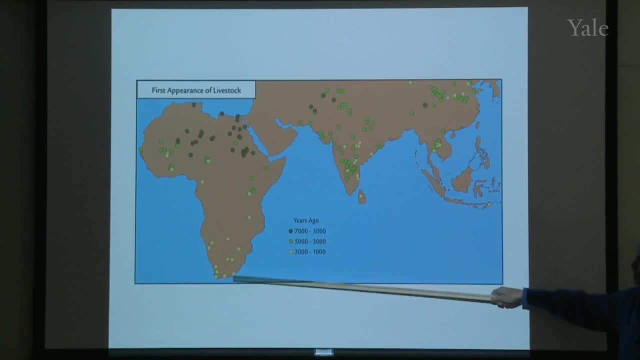 So this map shows you that extra methane is being generated here, here, here, and also in Europe, where people are just getting into, which I'll show you in a minute. So Could I just ask the calculation that you showed? can I assume that a count was taken? 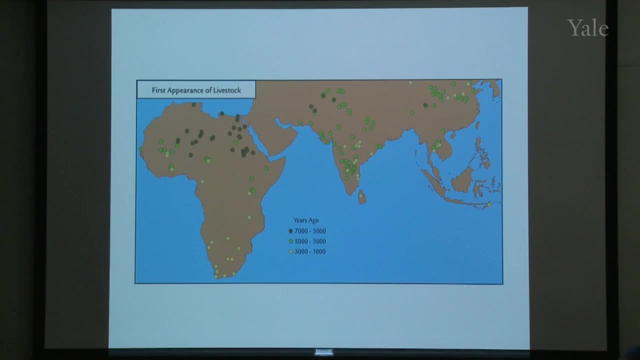 of a lifetime of methane in the atmosphere. It's a fairly short lifetime, It's very short. It's so short that it's pretty close to if you've got an acre, a hectare of rice paddy, you've got a certain amount of methane coming off. 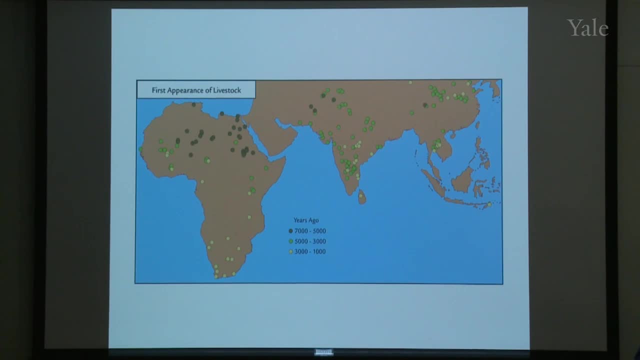 And it's going to sustain a certain amount of methane in the atmosphere, And so it's completely by analogy with the modern relationship. That calculation includes the oxidation of methane. That implicit, That implicit- Well, yeah, Those observations implicitly include it. 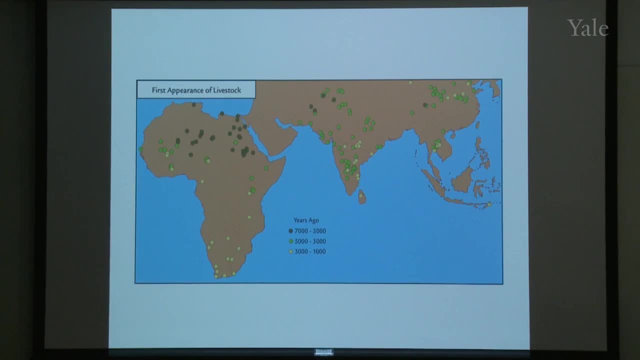 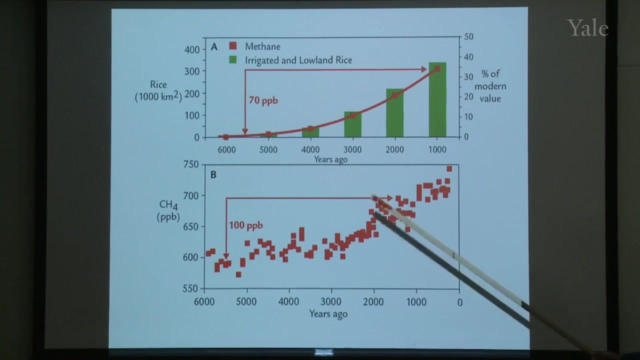 No, But the calculation you showed on the last slide, my understanding was that was an accumulation from the estimated rice growing, for example. But did that include the oxidation of methane? It may have. I mean it goes through the steps of rice area. 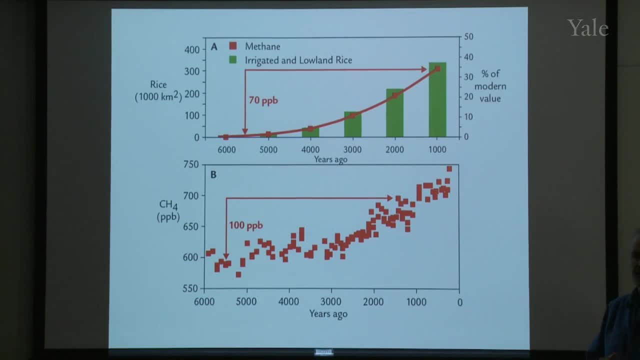 rice emissions linking to rice, sustained rice concentration in the atmosphere- the same relations that are used today. So it's just got the residence time. Yeah, I mean implicitly: yes, The residence time doesn't matter as long as the fluxes are changing. 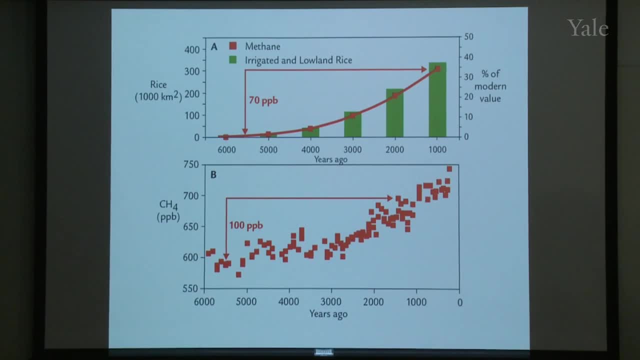 I mean, if there is an increase in methane flux, there's going to be an increase in the concentration of methane in the atmosphere. But people that are calculating how much of the methane concentration in the atmosphere is sustained by rice irrigation, they work back to the same numbers that Dorian Fuller is working. 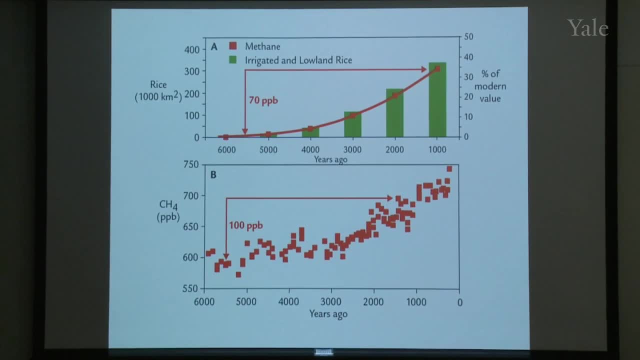 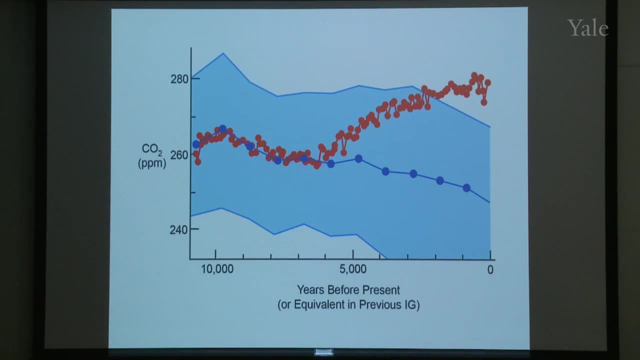 forward to. I get it. It's in that kind of steady state. Yeah, So that's methane. So there is rice irrigation doesn't explain it all. Maybe it explains half of the difference between the rise and the fall that should have happened. 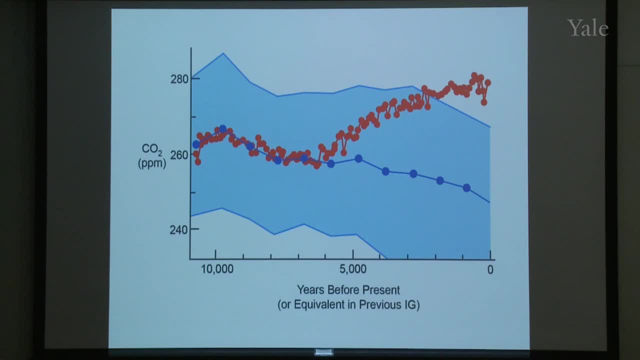 But livestock's out there. That's a really hard one to calculate, So you don't make it. There's too many. We could talk about that later. There's too many things you have to take into account. There's also biomass burning, which you could think of as if you get the debris from your crops and from your weeding, put it in a pile and burn it. If there's stuff smoldering in the bottom of the pile, that'll yield methane. If it's a clean, burn fire. 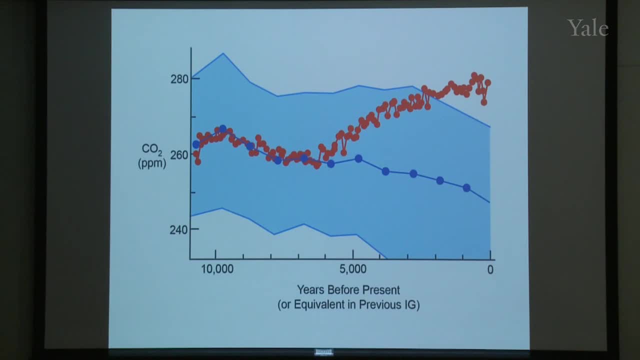 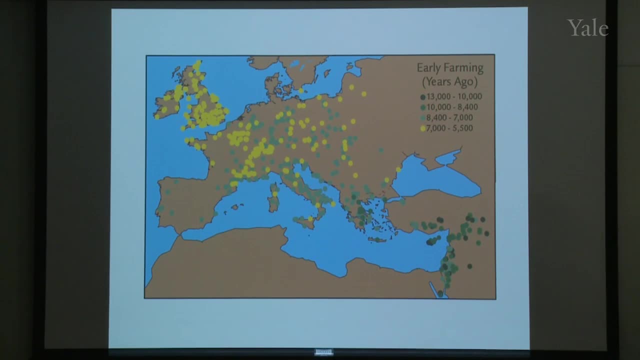 It'll lead, It'll yield carbon dioxide, But the stuff that's burning in this muffled environment doesn't. So now here's evidence for deforestation. I already showed you some. that involves that. This is work from Zohari and Hoff in the late 1990s. 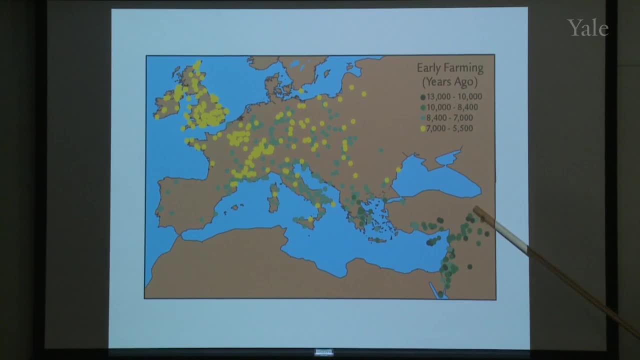 Here's the Fertile Crescent with domestication of livestock: cattle, goats, sheep, pigs, sheep and pigs, and crops of wheat, barley peas, lentils- a huge number of things that we eat today- And you can see that these two colors, which bracket 8,400. 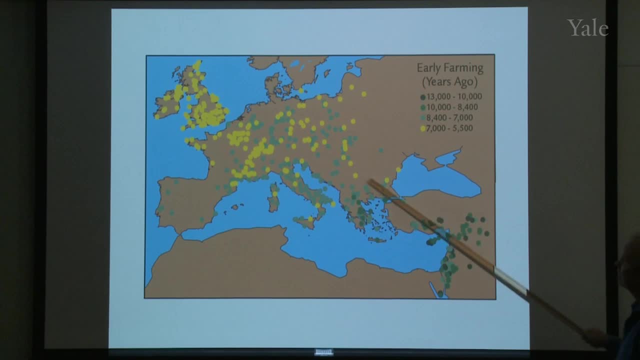 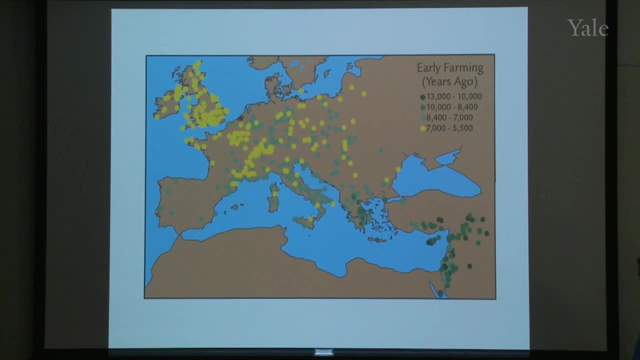 Agriculture has arrived at some density. So this 8,400 to 5,500, remember I showed you the CO2 curve starts to rise around 6,500.. So it goes the wrong way. So this spread of agriculture is very favorable to correlate. 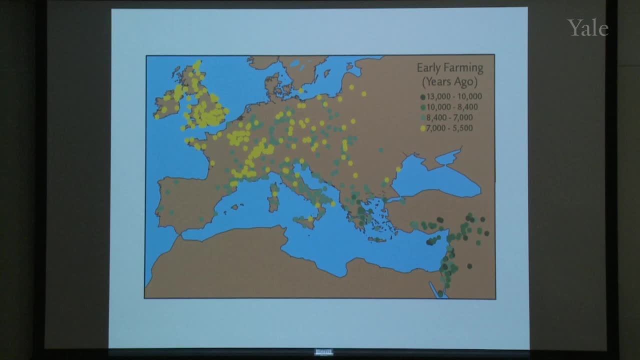 with the beginning of the wrong way. CO2 trend Point of interest. 5,500 years ago- we're not even into the Bronze Age- People are taking trees down with flint, very sharp, nicely crafted flint axes. They just girdle the trees and wait for them to die. 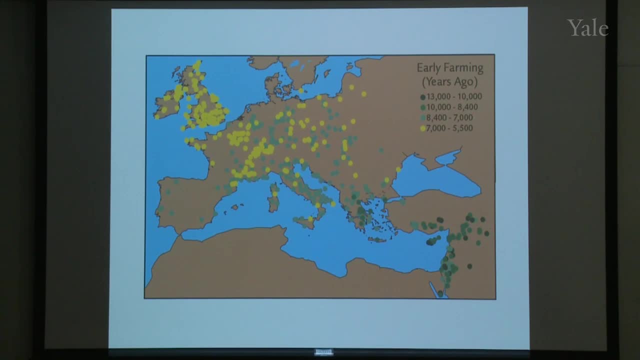 The debris falls on the landscape, They burn it, They stick what you would call today dibble sticks And you plant the seeds, They grow, Crops grow for a few years And then the soil plays out And you have to move on and do it again. 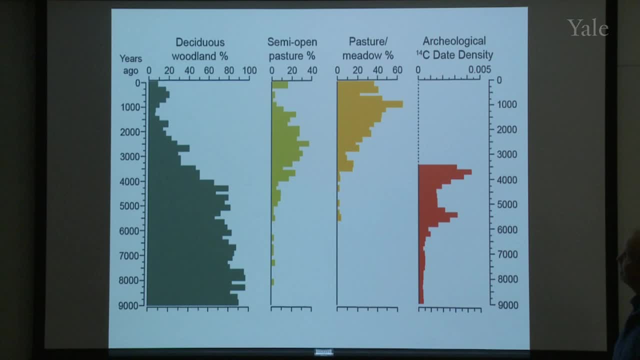 Here's from England, a compilation from England. We'll start with this. What is the density of C14-dated archaeological sites in England? And you see it starts to pick up somewhere 6,500 to 6,000, reaches a maximum. 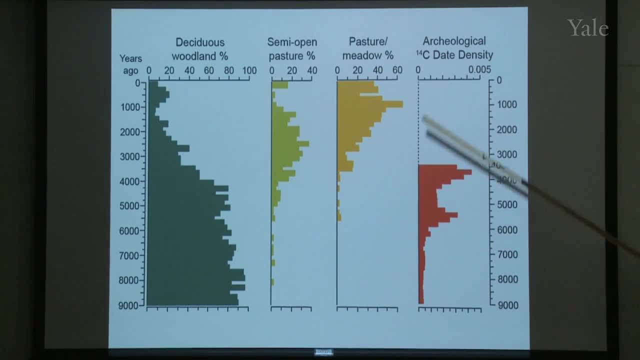 It goes back, comes back up, And then they- this compilation didn't try to map beyond that, plot beyond that, But that's that also consistent with that 6,500-year CO2 curve And meanwhile, the pollen which there's tricks to doing this. but deciduous woodland, pollen, forests basically starts a slow fade around maybe 6,000.. Come on, It goes very quickly after 4,000.. So basically, 1,000 years ago, Europe is as deforested as it is today. 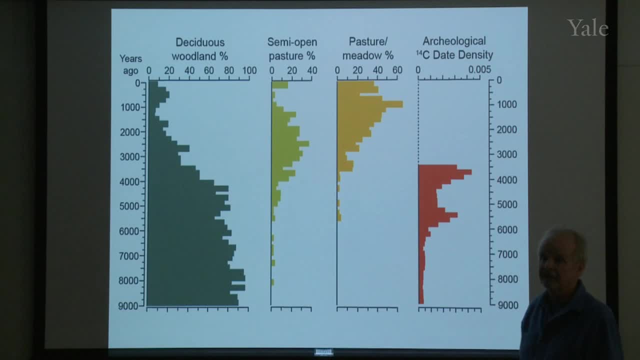 So this is getting into the question of how much deforestation happened and how much CO2 release happened before the industrial era, And the answer is a lot, most of it. There's been people in the literature saying that for 20 or 30 years. 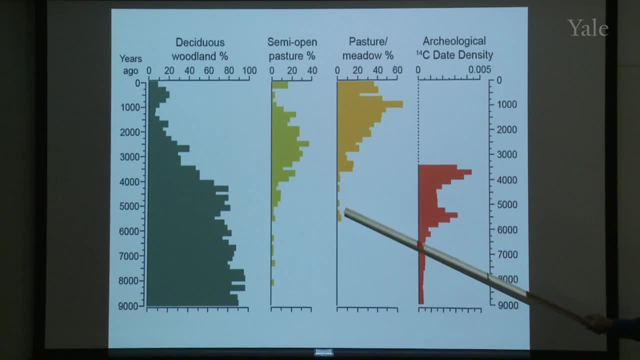 So what comes in is pasture, semi-open pasture, and pasture and meadow replacing. So the anthropogenic by these plots, the anthropogenic pulse is after 4,000, not quite as early as the 6,000-year CO2 reversal. 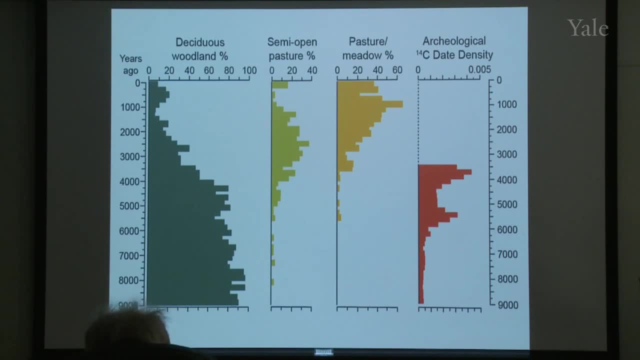 But for those that don't like the early anthropogenic hypothesis, you just cannot say that the Industrial Revolution was the time when the major deforestation happened. It's clearly very early. Is there a question? I don't think so. I have a question. 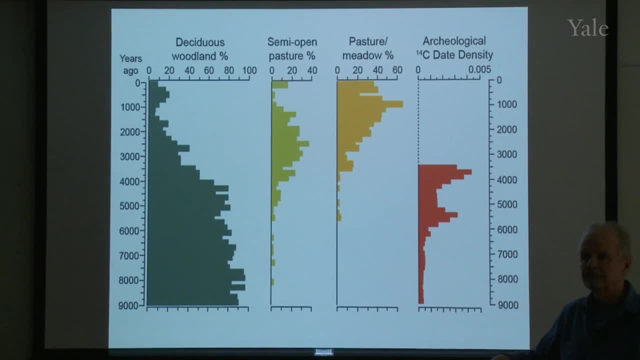 If you're going to account for CO2 through biomass burning, you can be quantitative about that right. CO2 by- yeah, fire Deforestation, Fire Deforestation. You can be quantitative in terms of the mass Right Right. 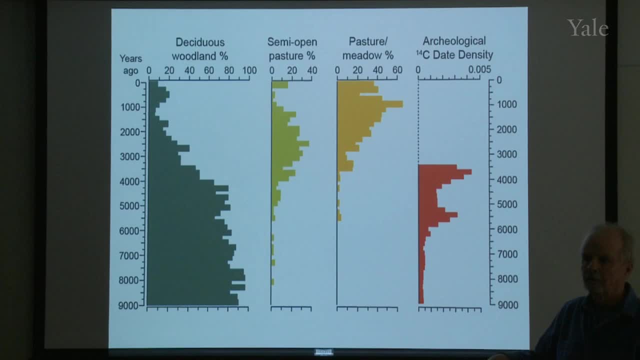 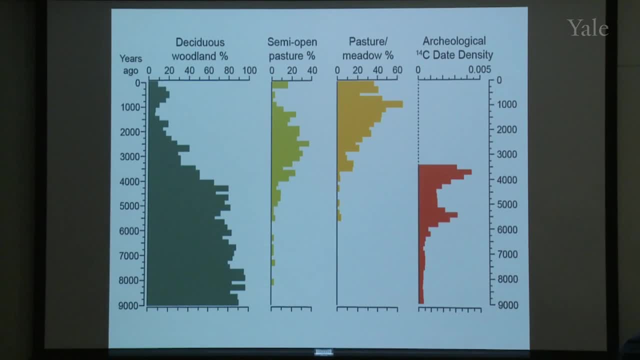 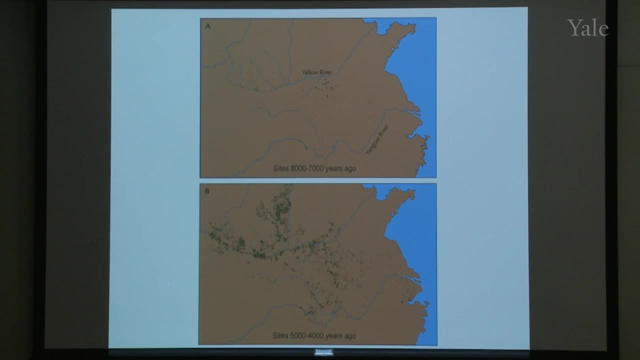 the carbon that would need to be released and associated with the ocean and all the rest. Yeah, I'll get to that, or at least part of that, in a little while. China has an enormous amount of data. I don't think Anne was here, who I met last night. 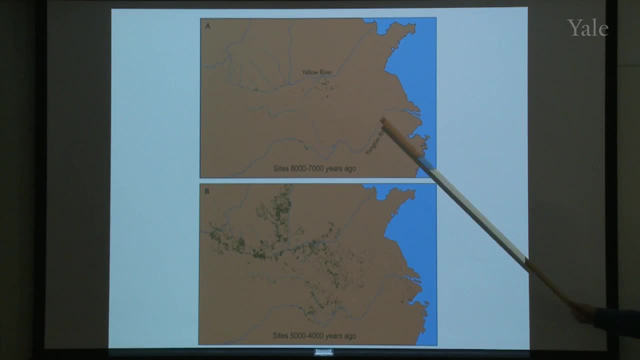 But there's much more than is shown here. But this is a plot of the climate. the number of archaeological sites in China between 8,000 and 7,000 years ago and between 5,000 and 4,000 years ago. 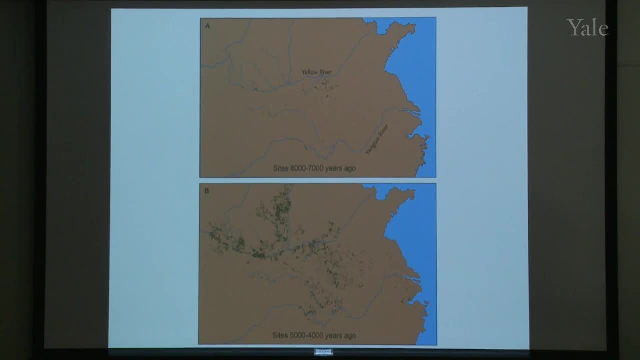 so two equal length time slices. 8,000 to 7,000 years ago, you see a scattering of sites up around the Yellow River, just a few in the Yangtze area. 5,000 to 4,000 years ago, the Yangtze, the yellow. 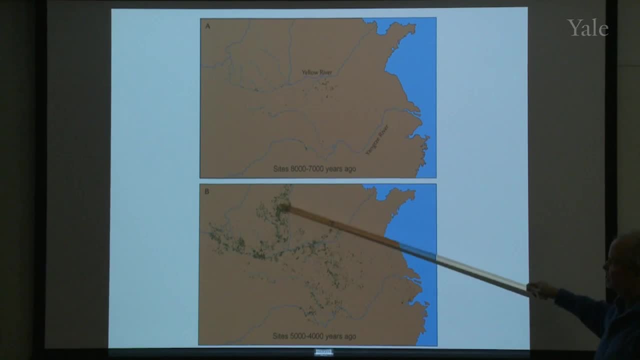 which goes up like this and then loops back down, is just jammed with archaeological sites. Everybody was a farmer, so this is all clearance And the density of sites between here and here that's a 30- to 40-fold increase. 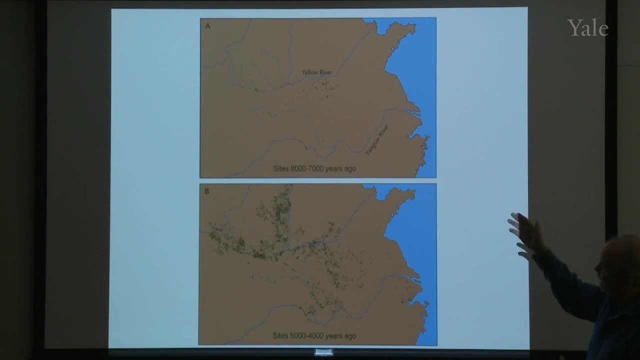 So that's a massive amount of deforestation after 7,000 years ago and by 4,000 years ago, And that's again consistent with the CO2 curve going in the wrong direction. Now what's going to pick up after this level is: 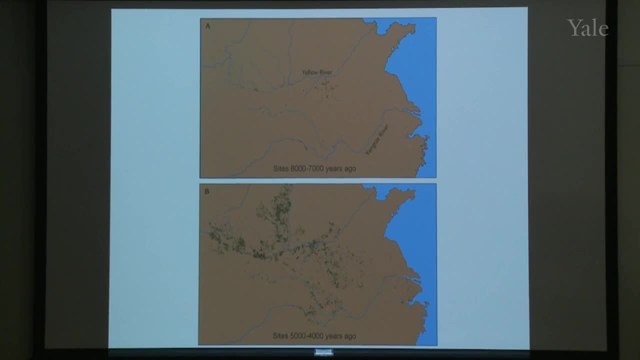 here's where the rice cultivation begins, the wet rice cultivation. So all this area south of here and down into south of China is going to be deforested as the terrain goes over to rice paddies. So the But those are the two areas, China and Europe. 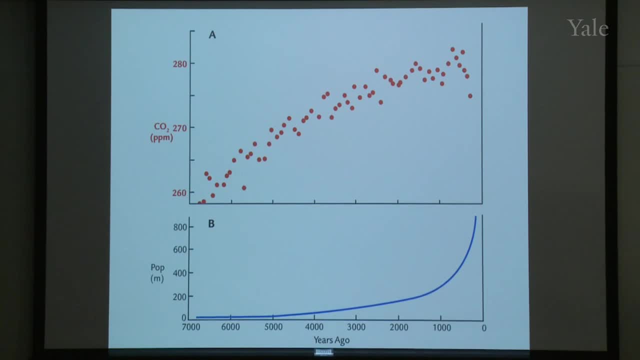 That was Britain, but the same pictures emerging for West Central Europe. The two areas. we have a lot of data show a lot of early deforestation back on time scales consistent with the early anthropogenic hypothesis. Now what I think is still the criticism of the hypothesis, which still has reasonable. 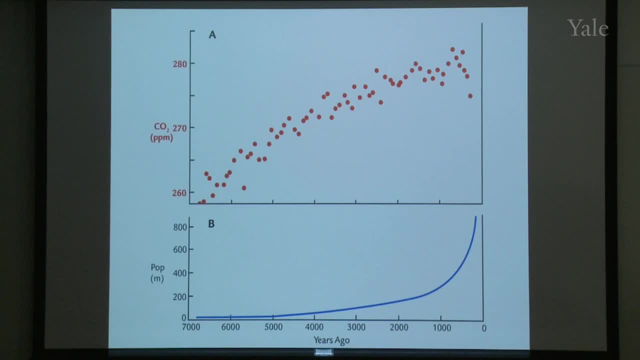 validity at this point it's being worked at and knocked down is. this is a simplification, But here's the CO2 rise starting about 6,500, rising rather quickly and kind of leveling off. coming into this, If you follow most people's population reconstruction, they tend to use these geometric curves. 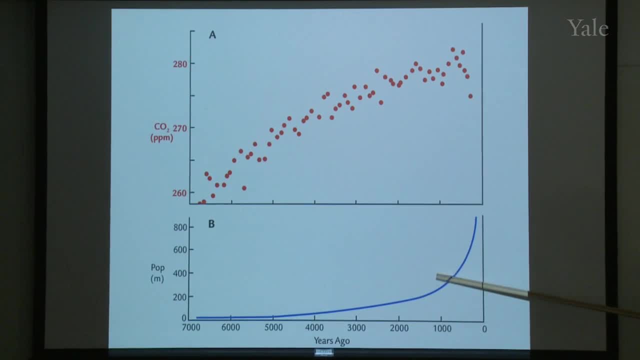 There's actually knowledge of population. Well, if you're a stickler for accuracy, we only know population pretty well back to about 500 years ago on a global basis. But you know population in China pretty well to here and also in Europe. 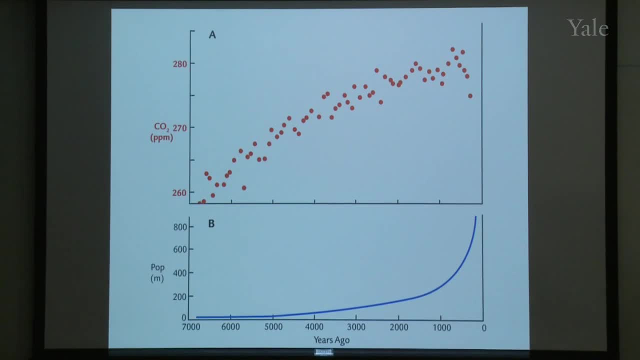 So that's about 40 percent of the planet And yeah, It doesn't look quite like this, but it's basically in that direction. Anything before 2000 is basically a hindcast. It's a backwards projection using a geometric model which assumes to put it in different. 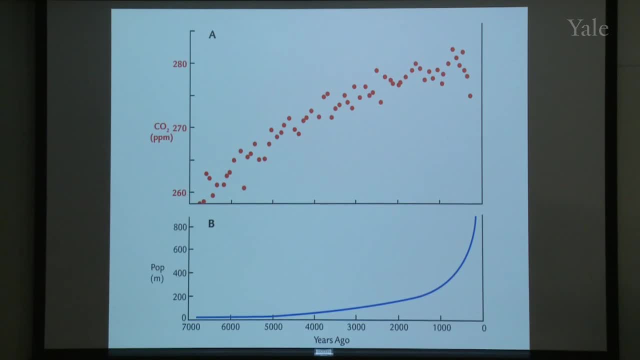 terms. it assumes a doubling of population somewhere around about every thousand years. These models assume a constant rate of doubling of population all the way back from 2000 to seven or eight thousand years ago. Now there's a problem with that assumption. It has the same fractional growth rate. so whether you're here on the curve or there, 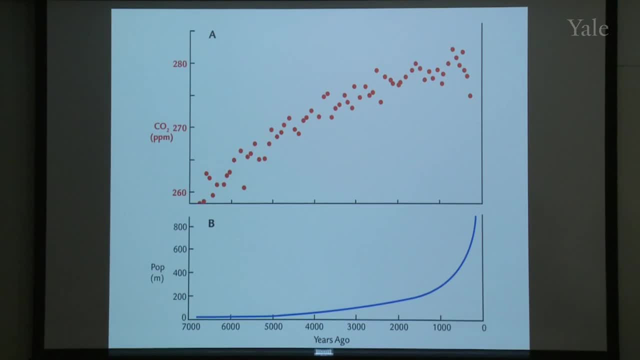 on the curve. the fractional growth rate of the population as a fraction of the population that existed is the same all the way through for 5000 years. That requires that all the constraints on population growth are flat, constant for 5000 years, which is a little—. 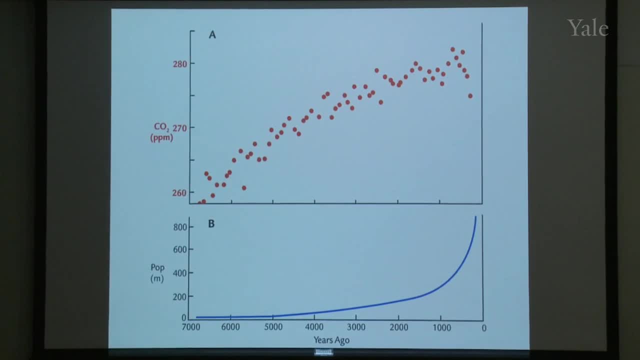 There's no constant. Yeah, What? There's no constraints? People just keep reproducing and increasing. Well, yeah, but they do it at a certain rate, which can involve constraints and non-constraints, But the rate is constant, which essentially means the environmental—it implies that 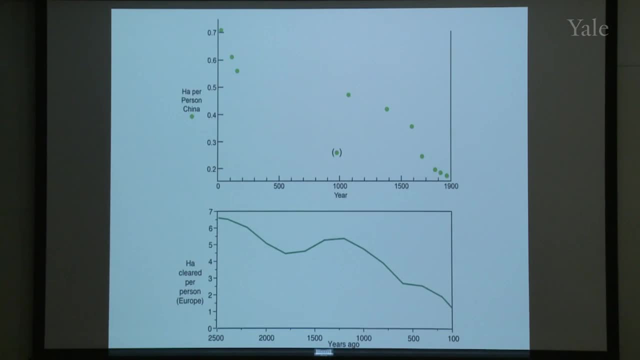 the environmental constraints are constant. Now that doesn't work very well. Here's a plot of hectares farmed per person. That's actual cropland, the area that a person- average person- farms. By the time you're back, you're up to the modern day. 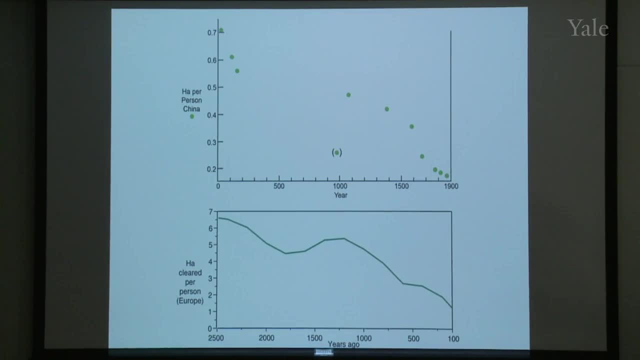 It's these tiny little garden plots in China. Typical agriculture in China is a garden plot, But as you go back there's reliable population data and reliable estimates of area farmed, collected by the dynasties, starting with the Han dynasty, back in here. 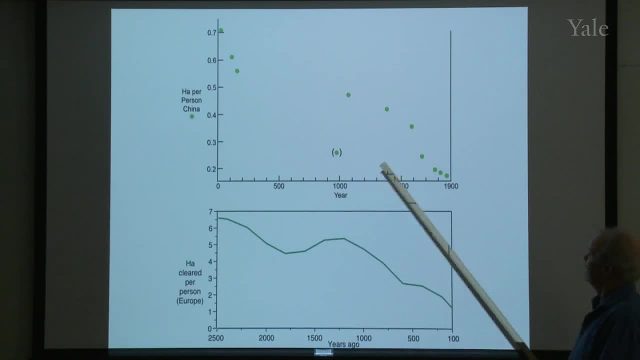 You can calculate area farmed per person and instead of 0.2, it's up in the 0.3.. Yeah, 0.18, it's up around 0.7, so it's about a factor of four decrease. 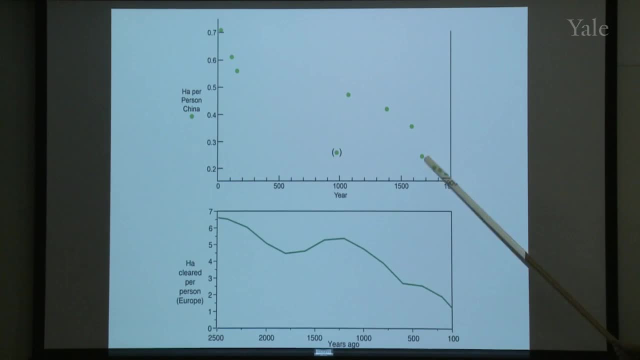 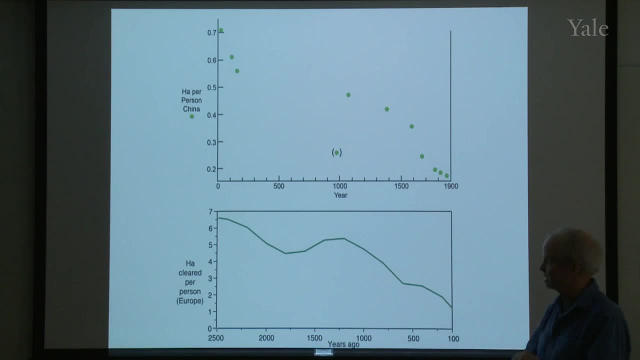 economy, That is, the global economy, was under $1.5 trillion, but it was under a lot of money. It was under $1.5 trillion. Can you imagine how much you could spend on the economy if you were to get on a car and 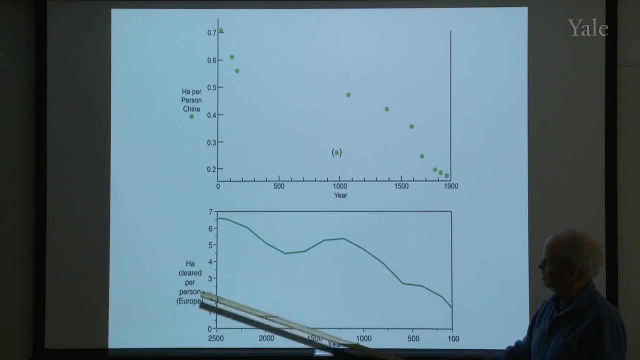 drive over there. It's not a lot and it's not a lot of money, but it's a lot of money. Yeah, You know, the economy really has a lot ofeds in it. It's not a lot and there's a lot of energy that's involved in the economy, but there's It's a different number. it's based on scattered maps of area deforested and population, which again is known reasonably well, And so this is how much forest was cleared, which is a much larger number than how much cropland was farmed, because it includes pastures and meadows and areas hillsides burned for. 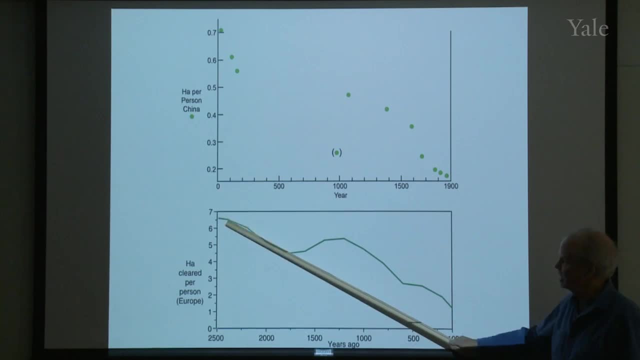 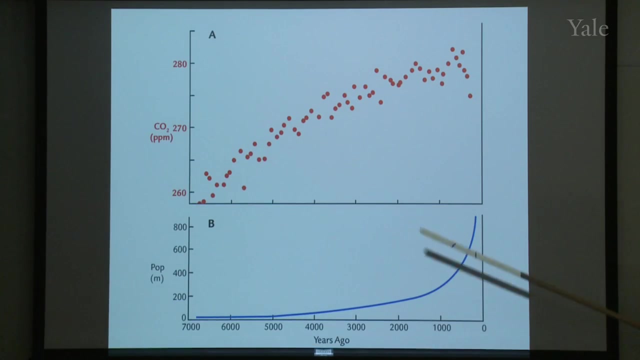 firewood and things like that, But you get the same factor of four decrease over the last 2,000 years, So people back here were using more land and I didn't make a point here. The problem with this plot is here's this big rise in CO2, and there's almost no rise. 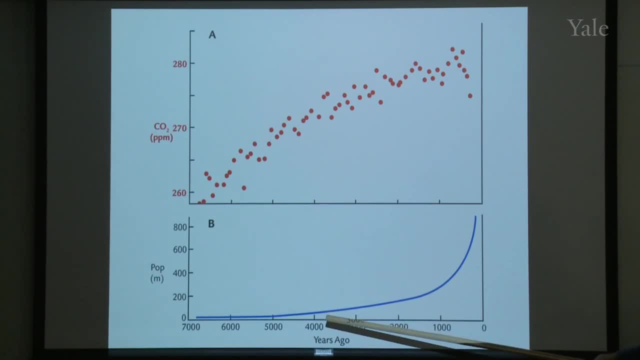 in population. So the valid criticism: how could so few people drive carbon dioxide- Carbon dioxide up so fast, early on? or to put it another way, if this is the cause and this is the effect, that's not a good relationship. The effect is thousands of years ahead of the cause. 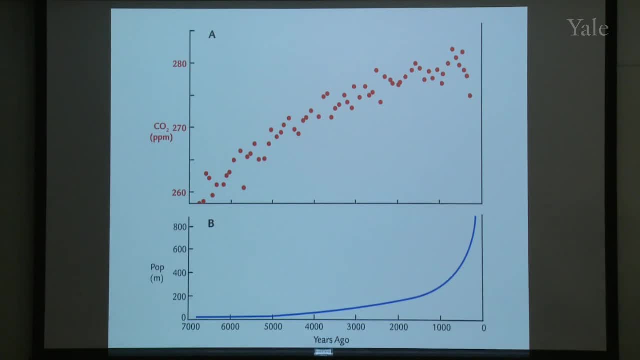 So part of the reason for that offset is that the populations back in here are not as low as they look. They're up higher by a factor of at least four even here, and it could be as high as 20.. Maybe five or 10 or so earlier. 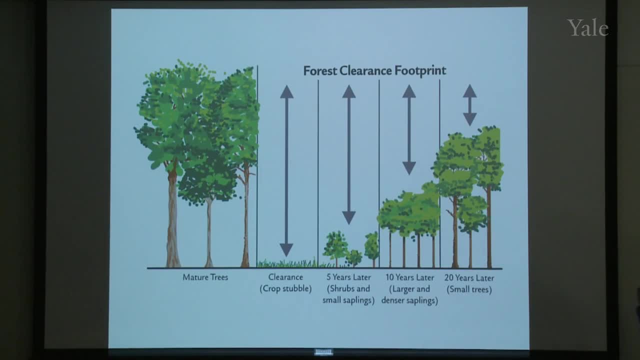 And to give you an idea of why that could be, if you take a mature forest and you cut it and you put crops in, as I was talking about earlier, the way people have tended to think about this- a lot of people and modelers have tended to think about it- is the amount. of carbon that's in the atmosphere is the difference between that and that? That's your calculation. But if people are moving every, it's usually every three to four years. they think by five years later. you're getting some carbon coming back, some saplings, you're getting larger. 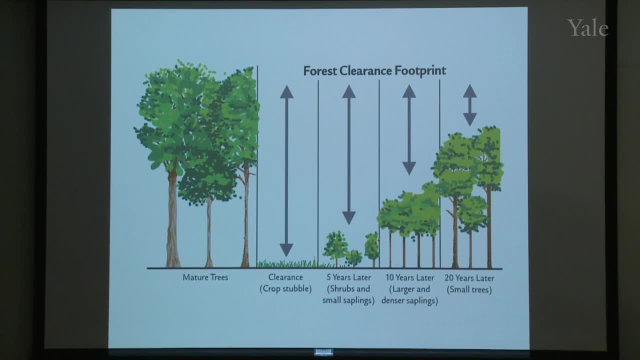 and denser saplings. You're getting trees 20 or 25 years later, but you're still not back to mature forests. So the carbon deficit, or the amount that went into the atmosphere, is this plus this, plus this plus this. 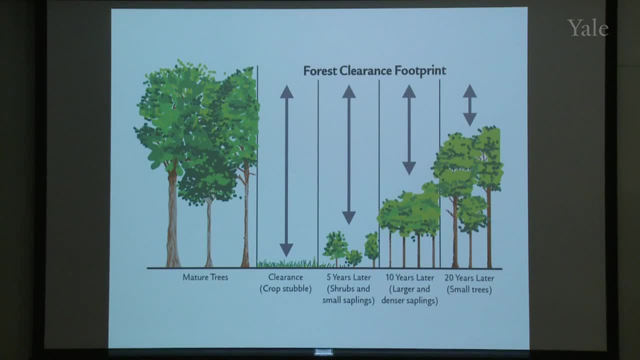 Right, So people leave a trail, a footprint of carbon emissions or- Averaged over a cycle of slash and burn. it's basically half that, Half the summation that I just did. Yeah, Yeah, you'd average out to be about half, or at least the maximum in clearance in 20. 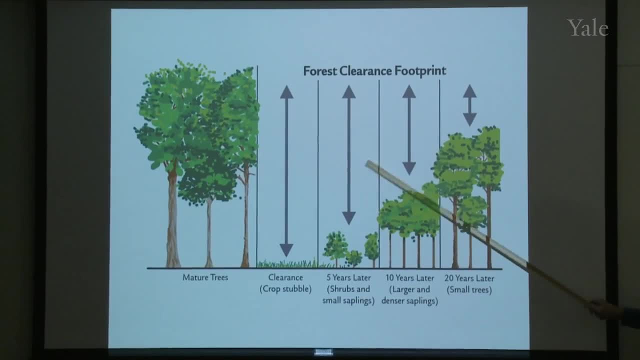 years. I would say you wouldn't use an average, You'd use the sum of these. I don't see how that's possible When you- When you deforest, if you put a plug of CO2 into the atmosphere, if the system is growing. 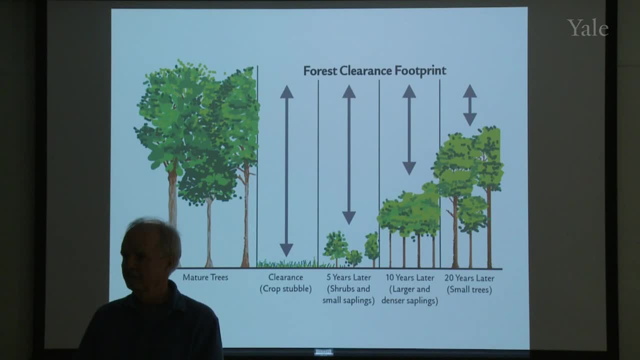 after that, then you're sequestering CO2.. Yeah Right, Going back to forest sequester. So you're not adding these arrows. The first plug is the only plug, and then there's a reduction in that plug And also- wait a minute- there's a couple other things that you haven't addressed yet. 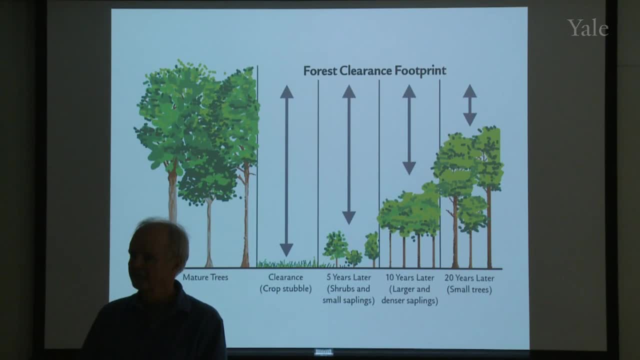 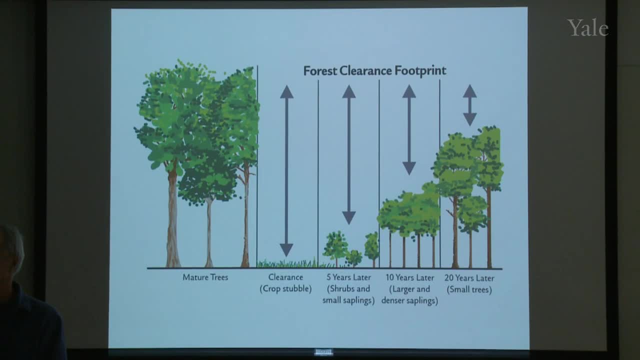 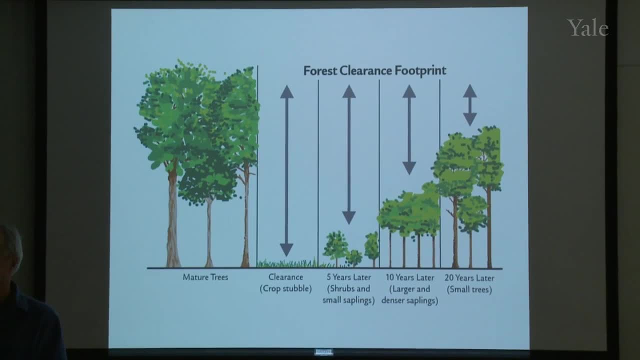 so it's even less So if the trend is going up. you have to sustain those emissions every step of the way. There always has to be more emissions in order to have an increasing signal, because the signal wants to be pulled out, unlike else. 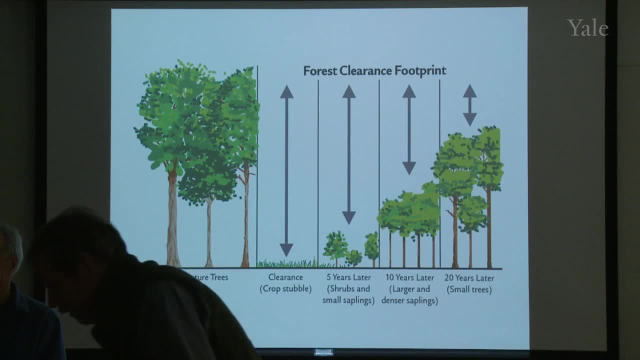 It has to be pulled out Like what? OK, for the same reasons as methane You need to have at any particular moment. any increasing trend means you have an increase in methane emissions or flux. I had an interesting confrontation with Paul Crutzen, who knows something. 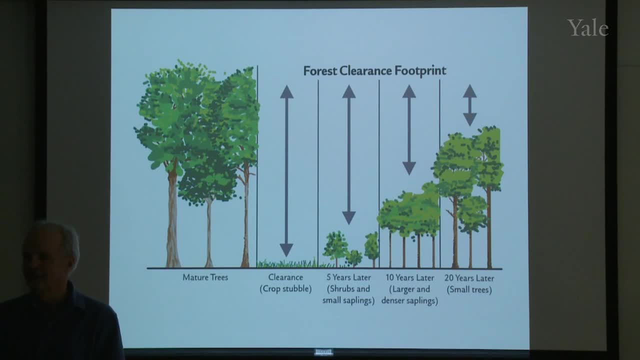 about this subject at a meeting about seven or eight years ago And he was making that more or less the same point as your first point, And I was saying, yes, but there is this deficit of carbon, It's coming back, but it's not back yet. 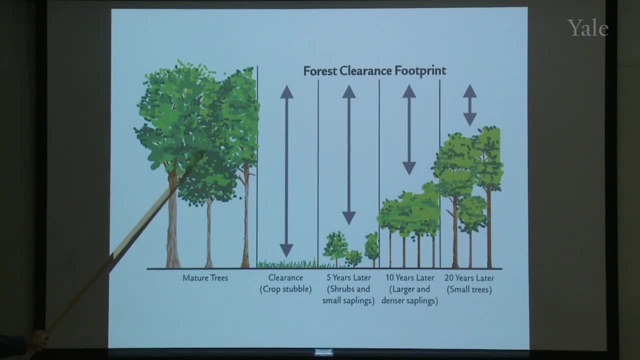 And this is just one slice. Three years from now, people are going to do this again and again, and again. So there is this for a family or for a person. there is this continuing footprint. So he didn't like it, He didn't believe me. 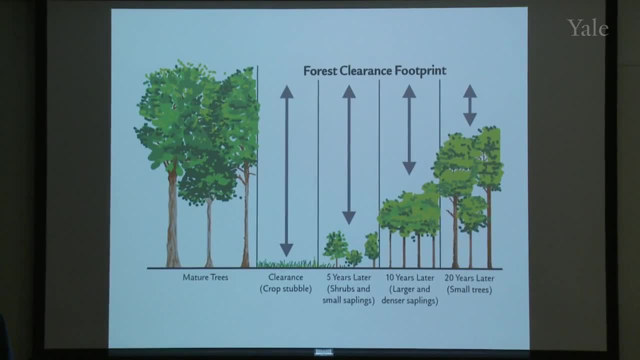 And I'm sitting at breakfast the next morning and he comes out and he says: you were right like that. So if you think about it, it's an obvious, intuitive mistake to make. But people leave a footprint And the people move around. 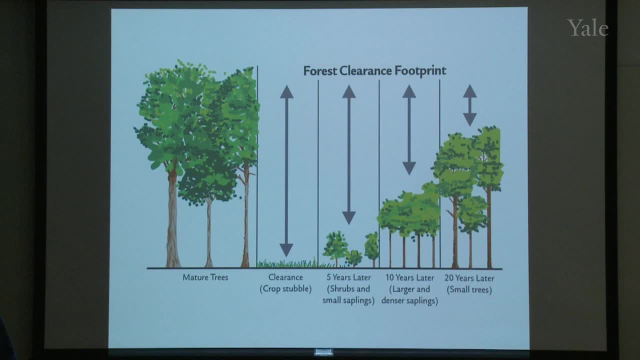 So, even though the whole forest in this particular region might grow back, there's still a footprint out there and it's following the people around, And so there are more people. quick answer: there's more people through time, more clearance, more. 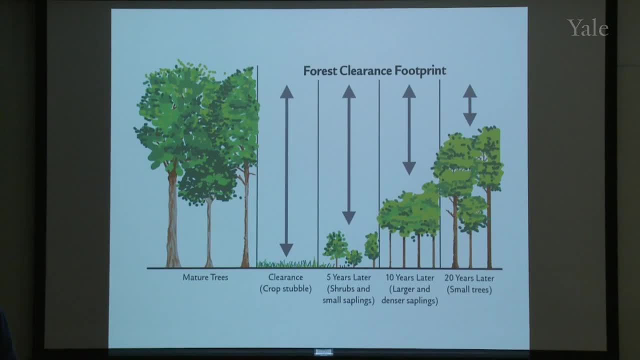 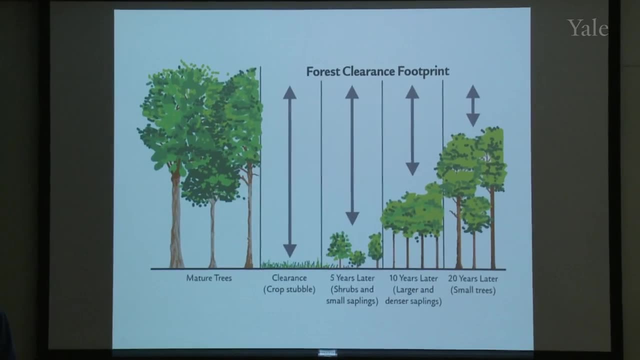 footprint. There's a lot of difference, moving around until finally areas become completely deforested And they don't grow back at all, which is when you get into the last couple of thousand years. But if you hold off, I think some of what I'm going to say 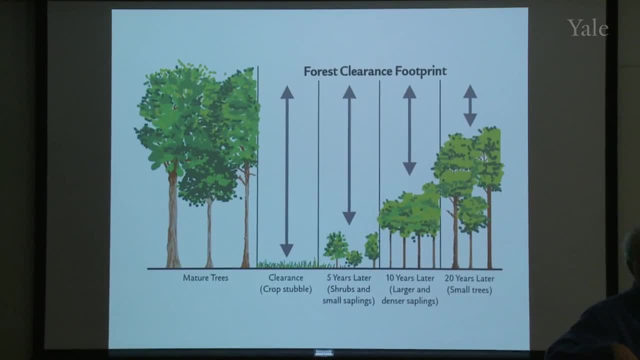 will cover this. I guess I have a question. Well, go ahead, Keep going, I'll ask the question. So that's part of the answer. You can't just look at the number of people on the Earth. You have to look at the fact that they're. 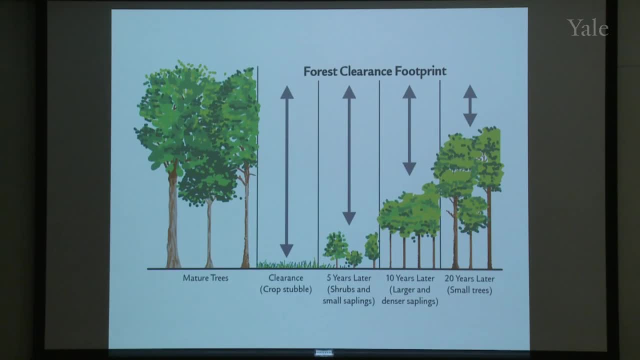 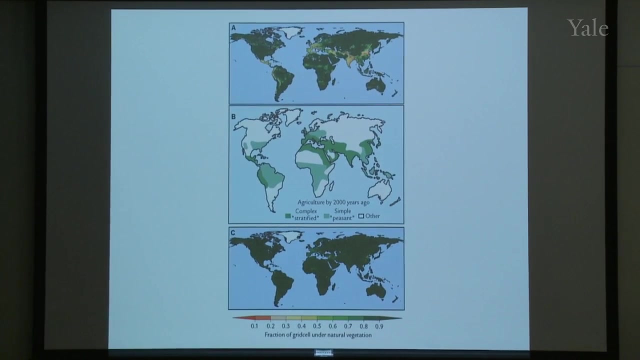 using perhaps four times or more More as much land. Their clearance footprint at any one time is four times as large as the population would suggest relative to 1800, where people are farming the same plot every year and not moving around. So the person that's dealt with this 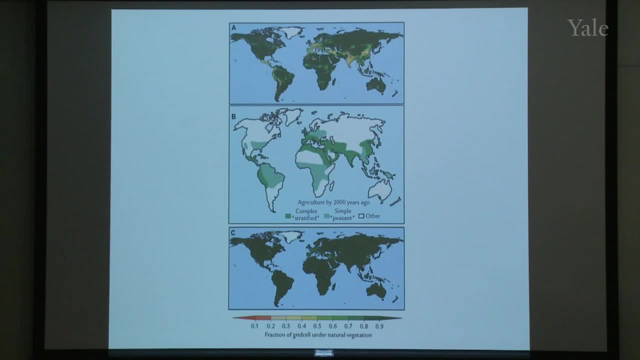 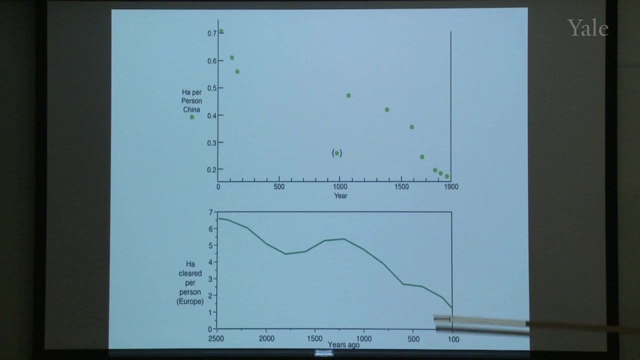 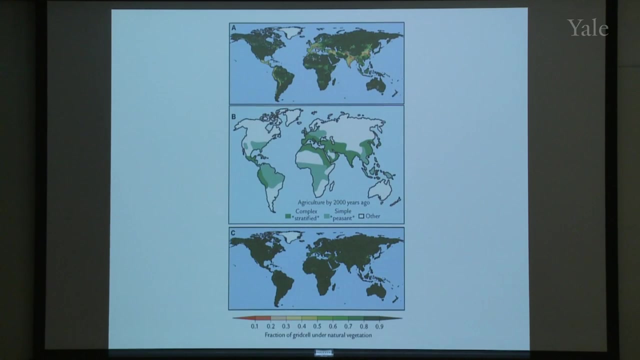 is Jed Kaplan, who I think was here. Jed Kaplan spoke earlier in the autumn And he ran two sets of models. One set of models assumes that the per capita footprint is the same low value that it was basically here, That's 1700, 1800, 1900. 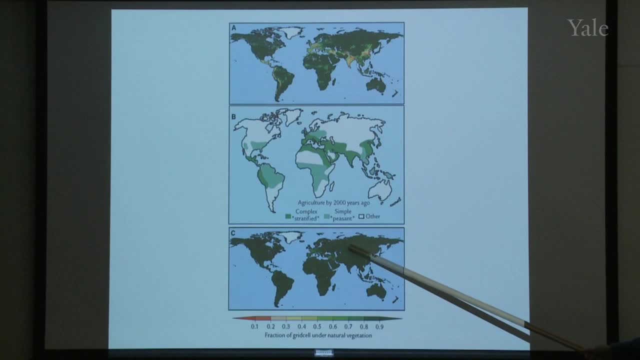 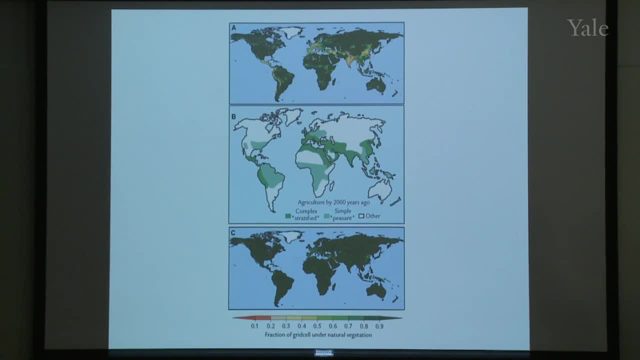 I don't know, I don't see that there's hardly any deforestation. Well, I just showed you that Britain is mostly deforested And China looks like it might be mostly deforested. But if you run a model land use simulation, 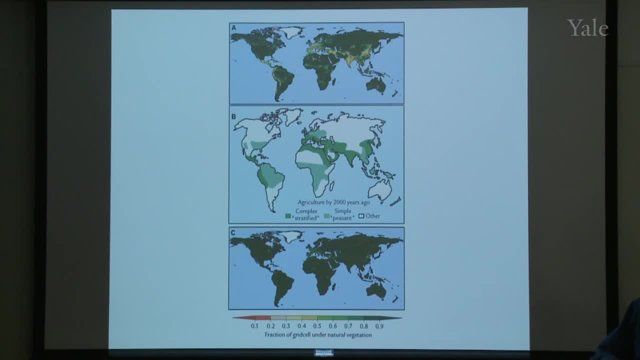 that assumes larger per capita clearance. early on you get a map that looks like that. So not just Europe and China In India, but the Inca, the Aztecs. There's the Fertile Crescent. You get larger splotches that are substantially deforested. 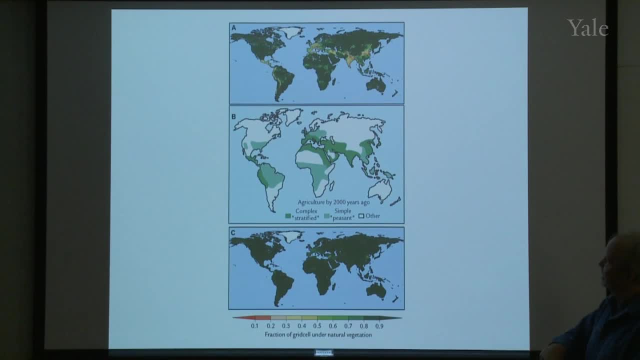 2,000 years ago. Here's a map from archaeologists published in the 1990s talking And this is basically: this is intense, relatively intense agriculture here and here which matches here and here which matches. So, And Kaplan's model looks much more like what the 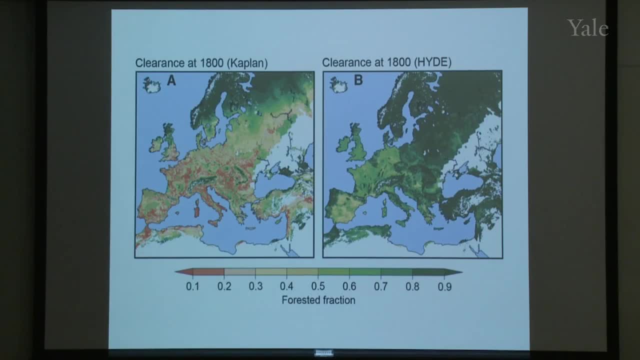 archaeological literature would suggest, But more persuasively if you use the model. this is the same kind of model: land use simulation. If you use the model, that and all these models allow for regrowth of forest if it's shifting cultures. 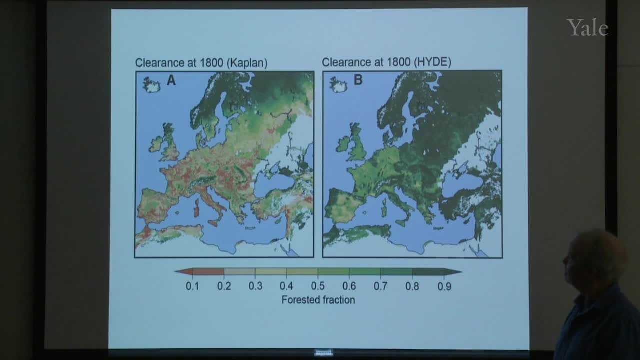 shifting agriculture. If you use the, If you use, If you use the model that assumes constant small per capita clearance, like we had in 1700 or 1800,, you end up with Europe being still mostly forested at 1800 AD. 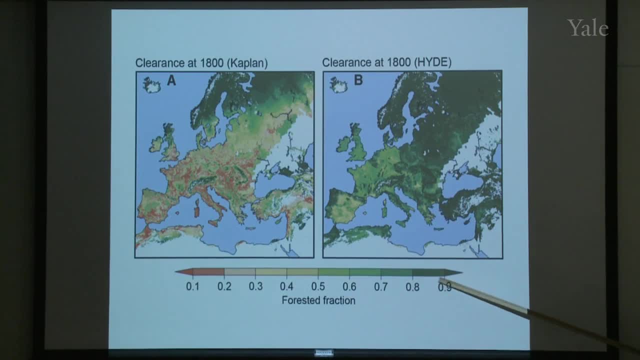 This is Jed Kaplan. again, Somewhere in the 50% up to 80% or 90% says that Europe is mostly deforested in 1800. Whereas Kaplan's model with higher early clearance gives you a Europe that's mostly deforested. 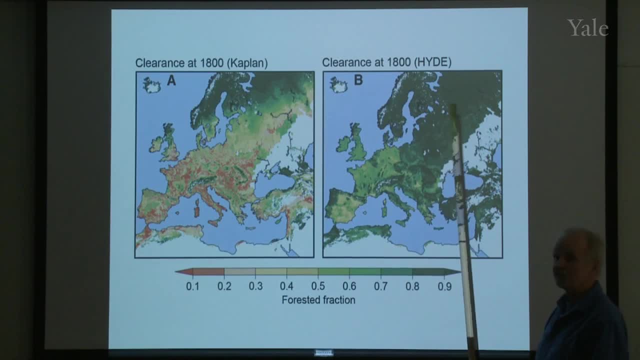 Well, we know which one of these maps is correct. That's wrong Because Europe has been reforesting since 1800.. Most of west central Europe's been reforesting, So if it was at 50% to 70% forested, 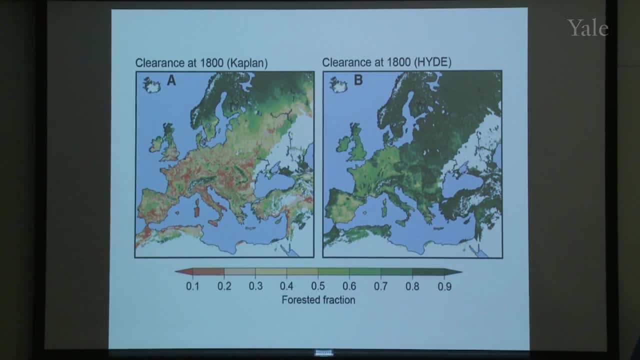 and it's been reforesting. Europe must be covered with forest. Well, Europe is mostly deforested, So this map is completely consistent with the fact that Europe has been reforesting since these map estimates, So Kaplan, must be approximately correct. 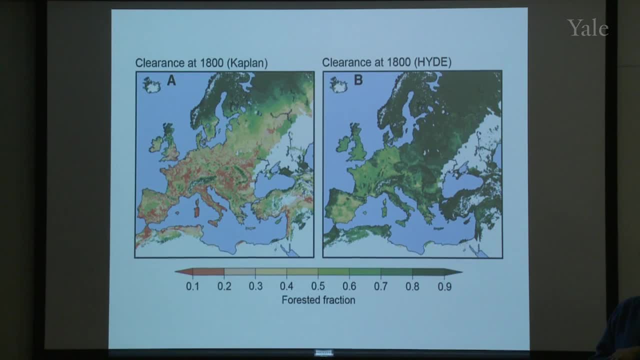 There's very large early deforestation And it's consistent with land use simulation models. There's three other models that give you: Europe, China, India, everywhere still largely deforested at 1800, which has contributed to this idea that the industrial era is. 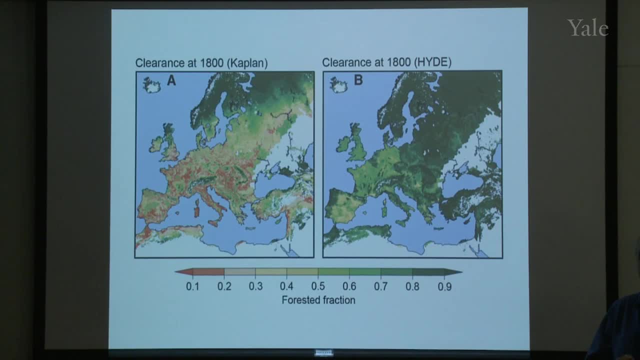 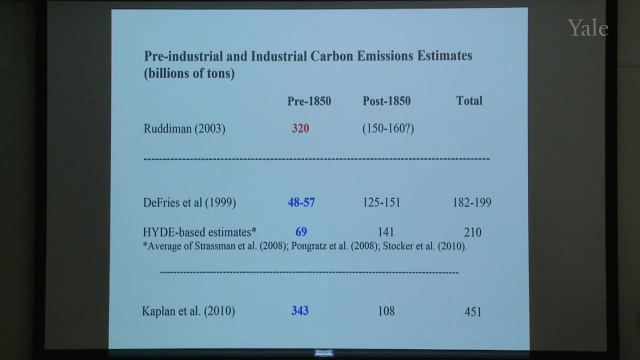 the big change of forest cover just the last 150 years. That's not true. It's much, much older. So I did a real back of the envelope calculation and guessed in this paper that something like 320 billion billion tons of forest might have been. 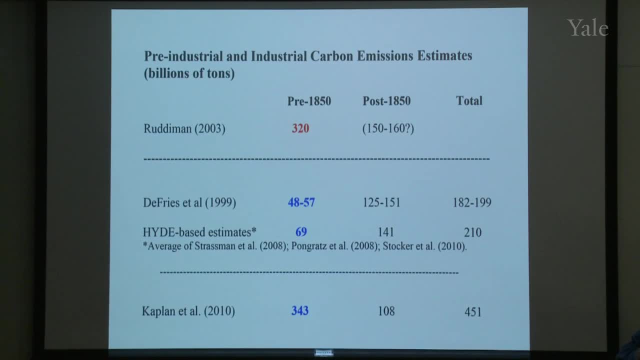 carbon might have been released to the atmosphere by 1850. And I did that by reading that literature that told me that there was major early deforestation, And I got this number: 320.. Along has come this paper and three others that have made that assumption of constant per capita. 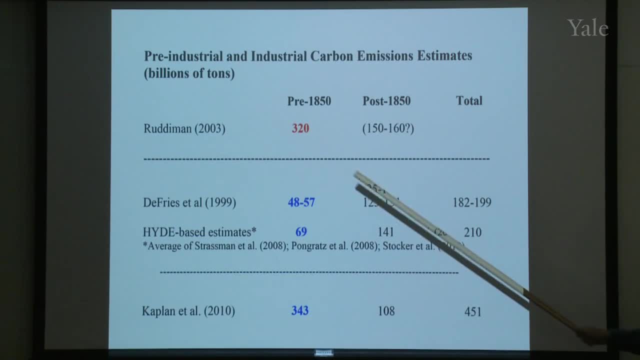 deforestation. And they get, And they get, And they get Numbers way smaller. So this has been a serious criticism of the hypothesis Numbers in the 50 to 70 billion tons instead of 320. But these papers all implicitly assumed- 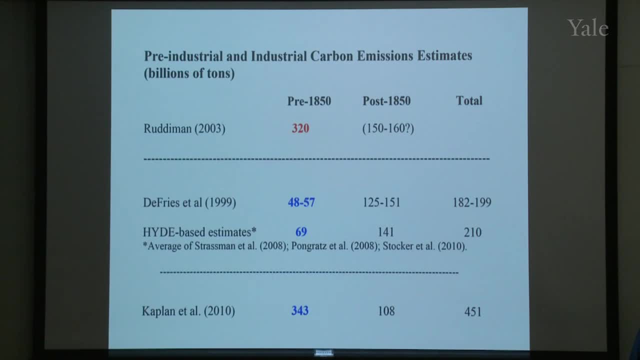 small constant per capita deforestation, which is not justified because we know that from the historical record, Kaplan gets a number that's pretty close to my lucky guess. That would be the equivalent if it was completely equilibrated with the ocean, the atmosphere-ocean exchanges. 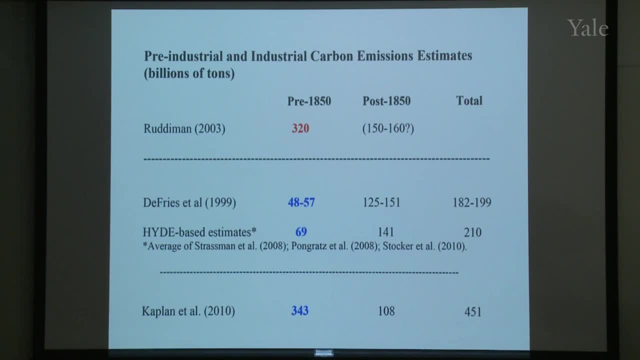 and geochemical exchanges, it would be about 24 parts per million CO2 anomaly due to deforestation, And I said from the top down view, I thought it would be about 40, the full anomaly. So this is moving in that direction. 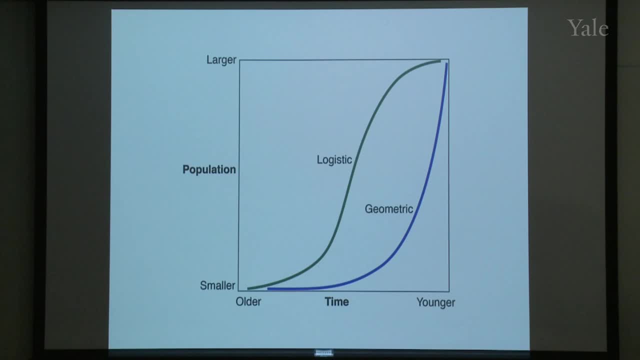 So part of the story is that a good part of the community has missed the fact that early people were very wasteful in their use of the land. They used a lot of land because they could, Once you get squeezed onto your one hectare of land. there's not much you can do about it. You just got to figure out a way to grow more crops, use manure, more manure, rotate your crops, things like that. But early on you just cut some forest farm a bit cut. 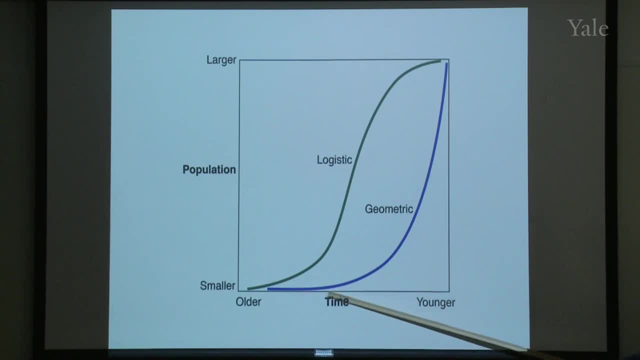 some forest farm a bit. So I mentioned earlier that these models of population growth, which you called guesses, I think, as you go back before 2,000 years ago, Total swag, Sweet, wild-ass guess. Oh yeah, OK, I'll buy that. 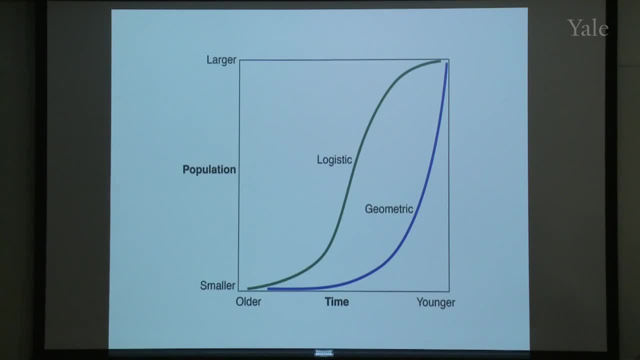 It's a model and bad input is bad output. So if you get that wrong, you're in trouble. There's another Who's in love with this calculator. You're doing my. the part I'm thinking in the back of my head as I talk is you're. 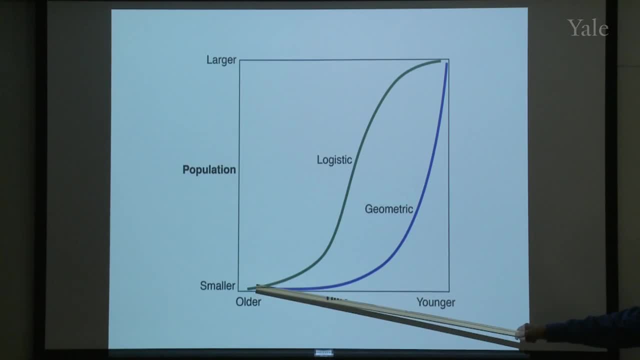 No, no, no Things. I would love to say TI-50. So they're different models, though Very common use may be people in the room that know much more about it than I do. Ecological models- ecosystem models. 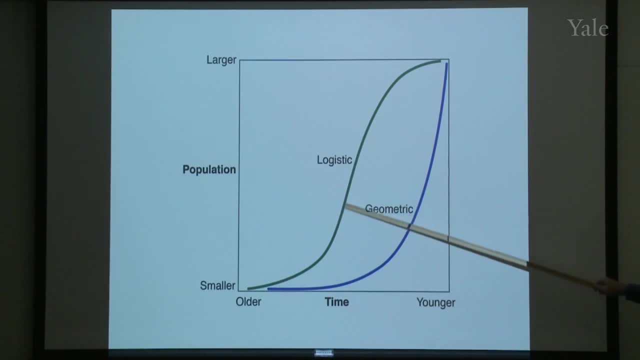 have a logistic shape And they basically have a much earlier rise relative to these geometric models. But then they tail off And the reasoning is logistic models. the resources are more abundant initially, But then they start to get used up. Life gets tougher. So think about people in forests going in here, people going into forested river valleys with rich soils, lots of water, growing crops, having terrific crops, Big families moving on. By the time you get into the last few thousand years, the land is occupied. 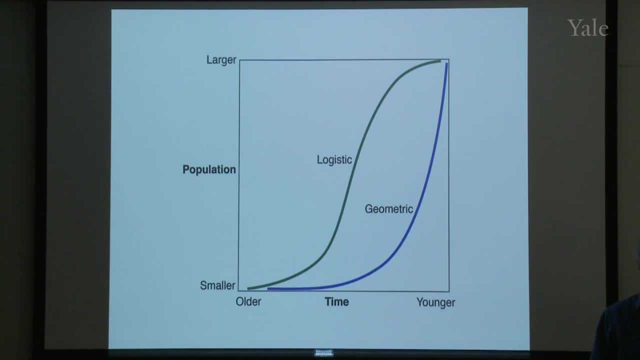 So you have a smaller plot of land, Or you're farming a hillside, Or you're having to farm in an arid region. So the rate of growth, the fractional rate of increase, is slower. There's a paper out in PNAS two years ago. 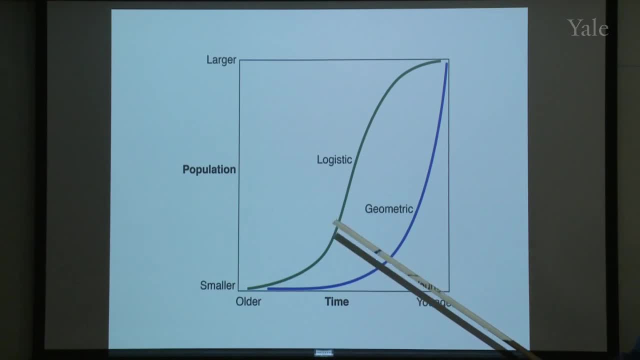 that shows that the fastest rates of growth using a mitochondrial DNA In Europe, southern southeastern Asia, south of China and North Africa- those are all sources of agricultural innovation- The fastest rates of growth are just when agriculture gets started. Fractional rates of growth. Total rates of growth are still going up faster more recently, But the fractional rates of growth, which puts more of the growth back in this kind of an interval? It's just after agriculture arrives, which is when you have this wonderful landscape just waiting for you to use. 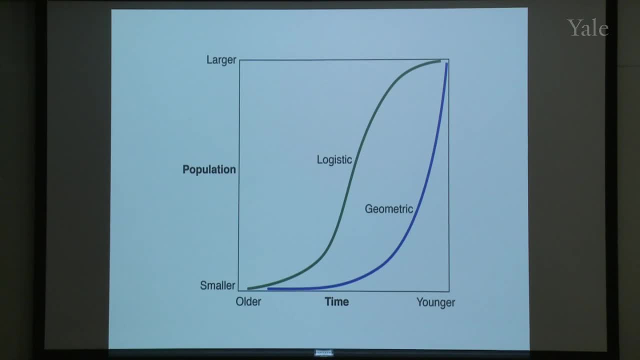 So this hasn't really been incorporated into papers, very, very much to deal with the effect that you're going to have. But basically, this DNA evidence And I showed you that factor of 40 increase in archeological The density of sites or number of sites in China. 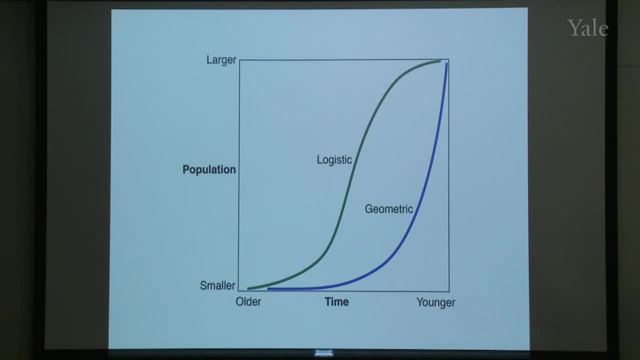 And I showed you evidence for increasing archeological sites in Europe, in Britain. I think when the population models, which are totally hypothetical, when they start to get grounded a little better, we'll find that there were more people much earlier than we thought. 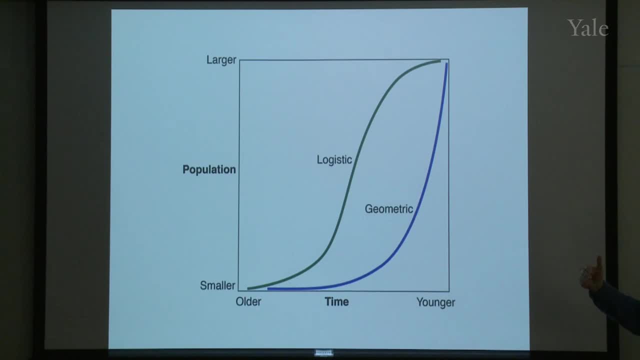 And if there's more people and they're using more land, you're going to start to close that gap, Or maybe completely close the gap between the explain that early CO2 rise. There were a lot of people then And they were growing very, very fast. 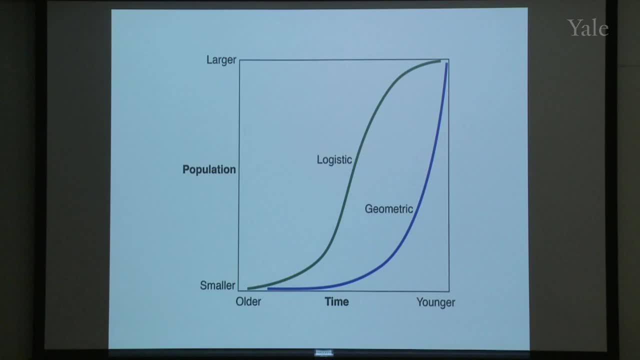 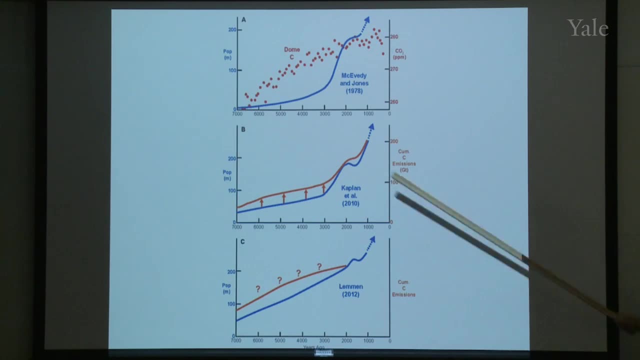 And they were using a lot of land. I have two more figures, but I don't think they help very much. Oh yeah, this one might help a little bit. So here's what I would call the geometric view. Here's that CO2 rise. 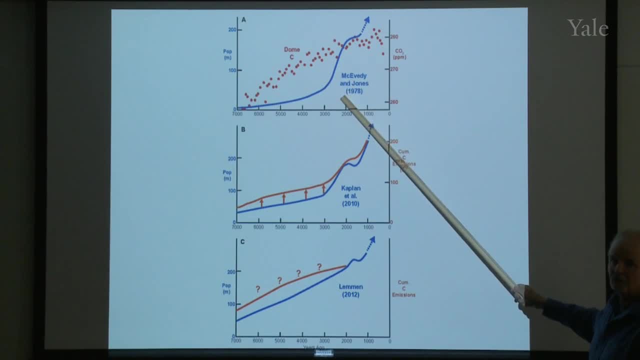 And this is: This is a slightly different version of McEvity and Jones, which is basically it's a geometric model prior to 2,000 years ago. So here's that mismatch. Jed Kaplan used a population model that started to incorporate some of this logistic population. 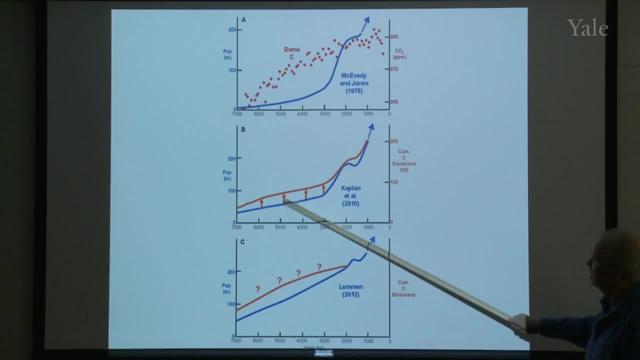 data. So his population curve is considerably higher, considerably earlier, And he gets that boost in carbon emissions. So this is, that's CO2.. This is, This is cumulative carbon emissions. He gets a boost which brings his cumulative carbon emissions. 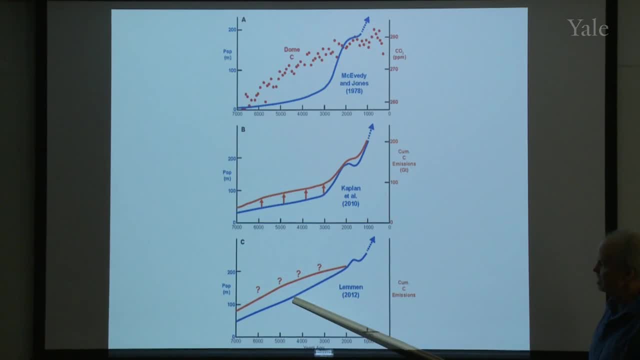 curve up higher. Carsten Lehmann in Germany is one of the ones doing this population modeling And his latest model looks like this. Still more people back in here, And I just eyeballed in what the carbon emissions curve might look like based on. 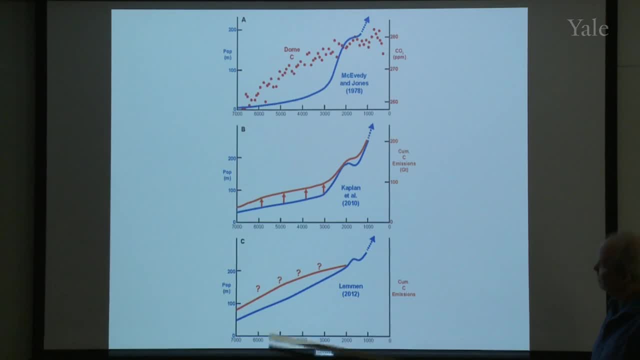 OK, OK. So I'm just going to stop here. I'm just going to go ahead and go back to the slide. I did a little bit of back and forth on that kind of a relationship And now, between 7,000 and 2,000 years ago, 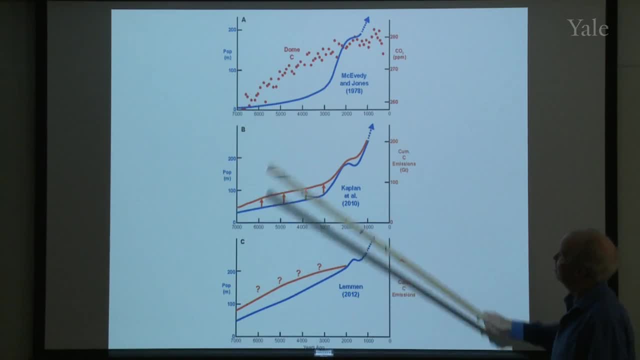 you're starting to get a higher increase and almost a hint of a convex shape. It's beginning to look pretty much like that. So this debate is the least resolved of everything I've told you, except somebody will ask me about delta-13, CO2.. 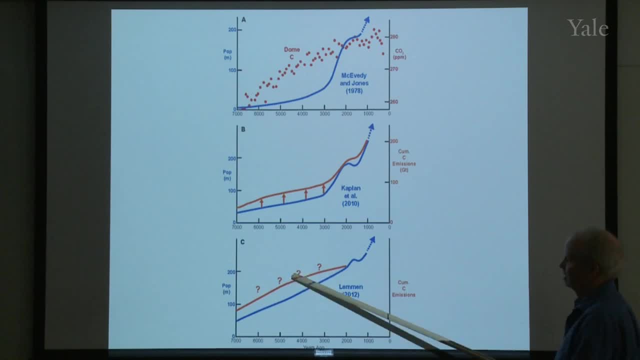 But I think this is the direction the whole thing's going to go: People that think there weren't enough people. there were more people than you think and they were using way more land. That's the way the evidence is taking us. 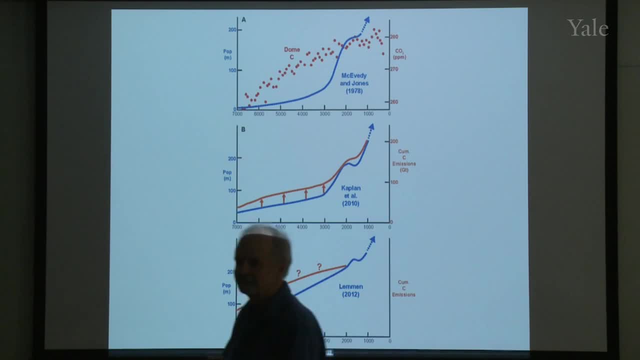 So you remind readers, since I was about to ask you about the C-13,, C-13.. I'm getting in an age where you need to speak up. You remind readers, since I was about to ask you about the C-13,. if deforestation needs, 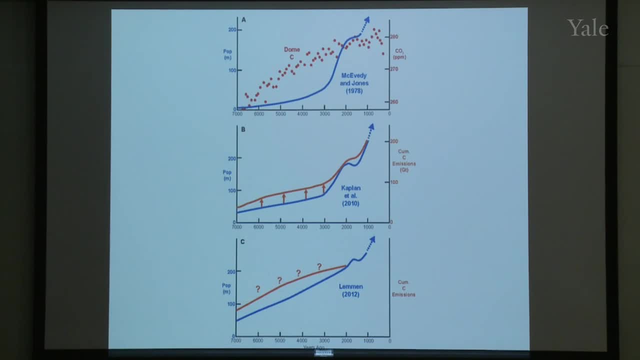 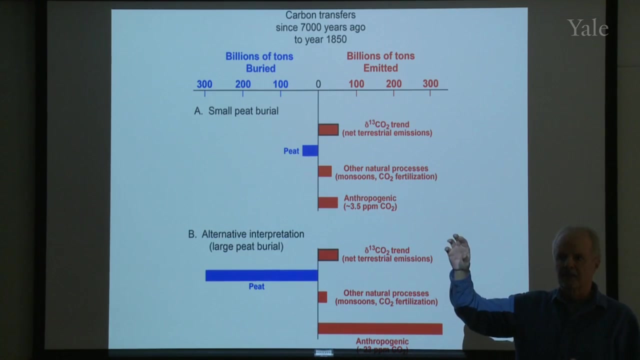 the whole CO2 increase signal, then C-13 can decrease how it supports that. OK, Matt, I can speak to part of the problem. So the basic evidence is that the Del-13 CO2 signal the C-13 composition of the CO2 in the air. 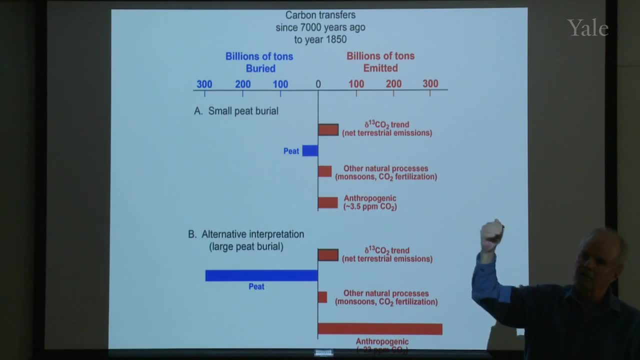 bubbles in the ice cores that are dated. it grows slightly more negative over the last 7,000 years, But it's only very slightly more negative And the people that came up with that data from Barron Institute, Elsig et al- first author- you have 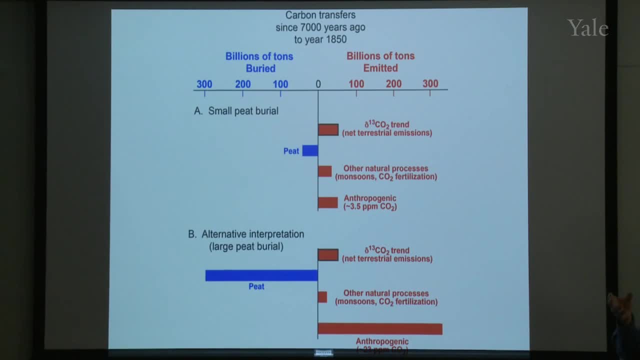 to do a mass balance calculation to figure out where things are going. I jumped over. The fact that it's going more negative in that ratio means that there's an excess of terrestrial carbon emissions over. It's only a very small excess And their conversion allowing for, so there's 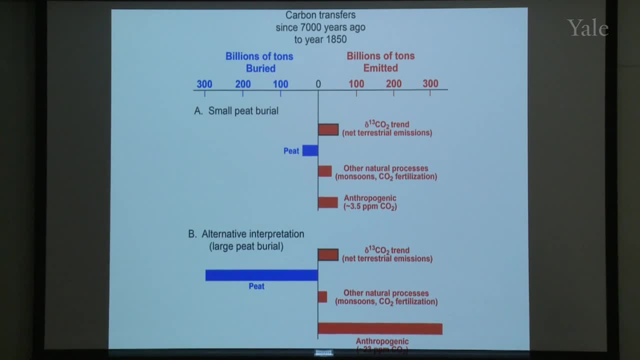 they allowed that. that trend suggests about that much by way of billions of tons of carbon emitted between 7,000 and pre-industrial. They allowed something for monsoons And they made an estimate of the peat, the carbon stored in peat. 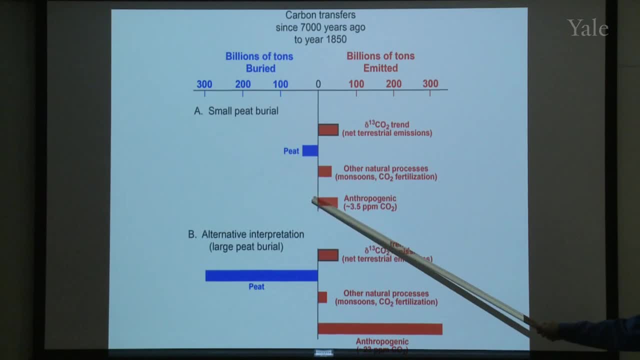 That's not emissions That's taking out of the atmosphere, And their estimate of the anthropogenic effect was 3.5. Well, I'm arguing for 40. And Kaplan's data, just on one factor, argues for 24.. So we're way out of agreement. 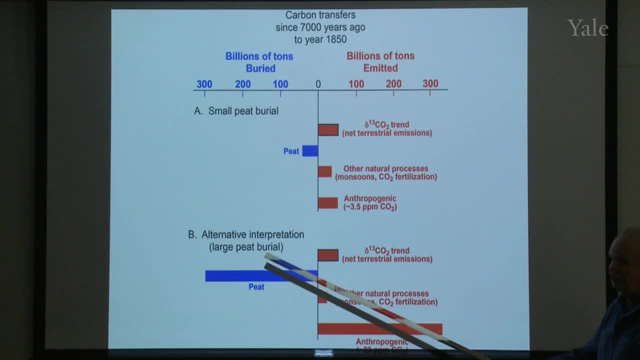 Well, I read that paper and I know something about the peat literature. that estimate is. It's simply not justifiable. There are two very impressive compilations of the amount of carbon buried in peat in the last 7,000 years. 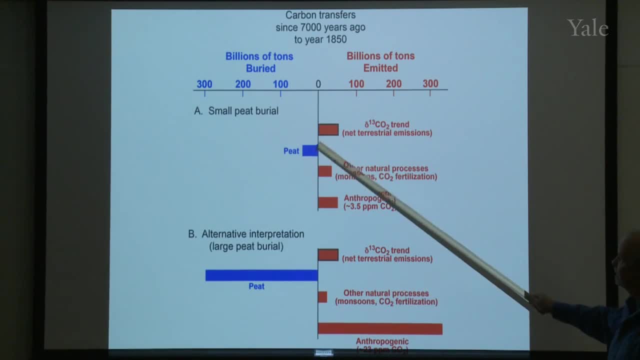 And there are about 300 billion tons, not 40. That trend is the observation that they made. I kept this. That should be the same as that. It doesn't look quite the same, So, assuming we know that's still the CO2 trend. 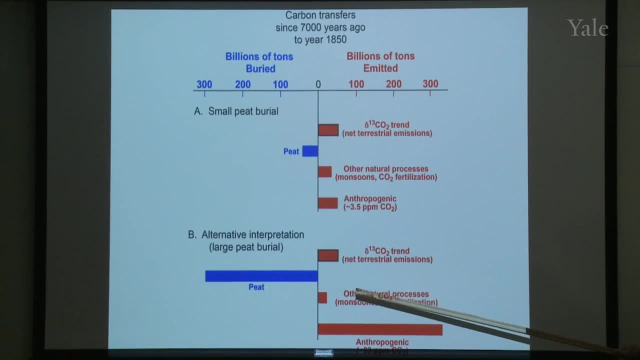 delta 13 CO2, we know. if that's a reasonable estimate and it's their estimate, then where's the balance for this? Well, I claim it's anthropogenic And that number would end up being about 300 billion tons, And if that sounds familiar, Kaplan got 340. 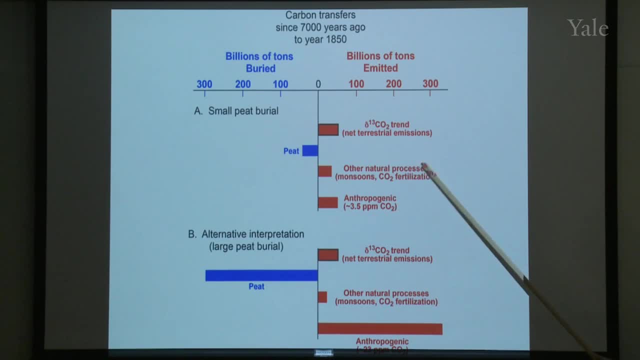 Now I've talked to Hubertus Fisher, who was a co-author and he's in that Bering group And they have, And they basically admitted that the peat storage was much larger than their estimate. And, Hubertus, unfortunately I've lost the email. 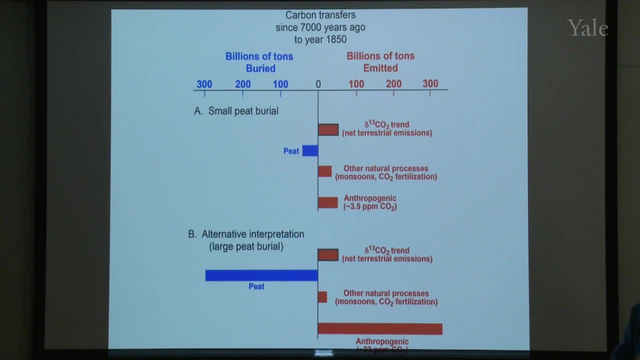 but he said in an email he said the delta 13 CO2 argument is no longer a killer argument against the early anthropogenic hypothesis. And then he said something to the effect of: there are too many large reservoirs which are not well known. 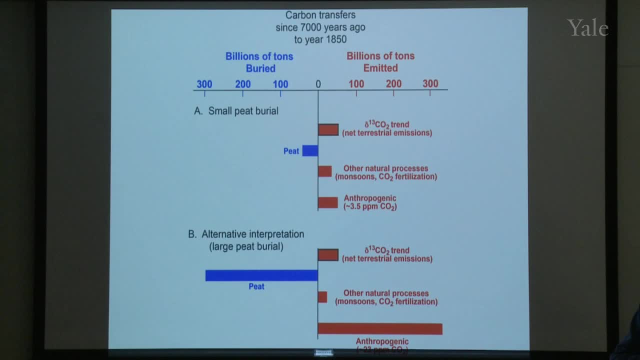 There's too much accommodation space. It just doesn't solve the problem. So something that I would say that virtually the whole community thinks is a killer argument is not by their admission. It still leaves some problems because that's still the net. terrestrial emissions.